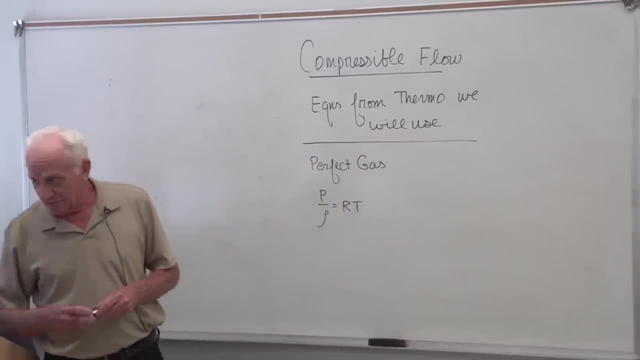 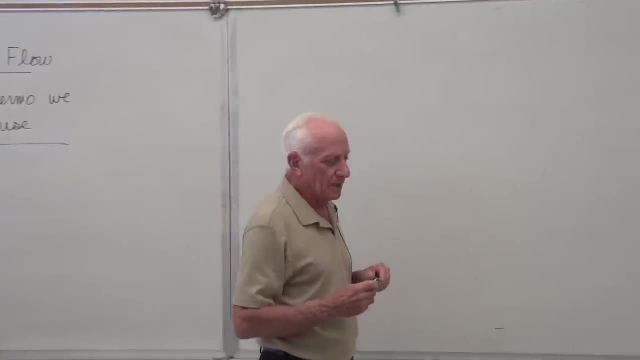 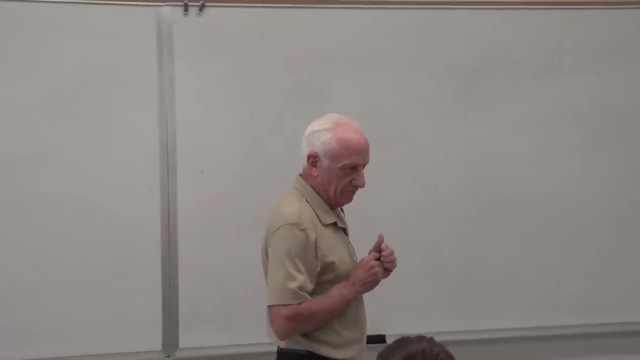 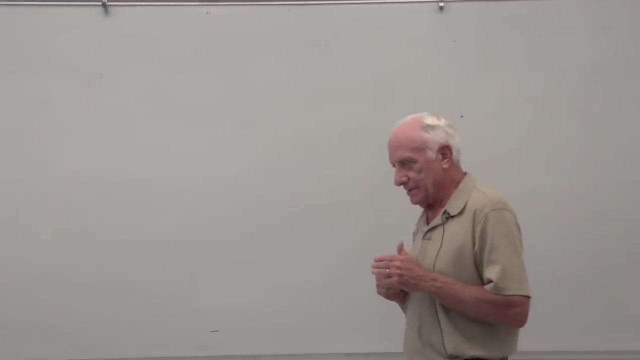 course is where compressibility effects are important in fluids. In ME 311, the first fluids one class, We pretty much treated the liquids as incompressible: Water, oil, whatever Incompressible. We pretty much treated gases, especially air, as incompressible. And that can be done. Air can be considered. 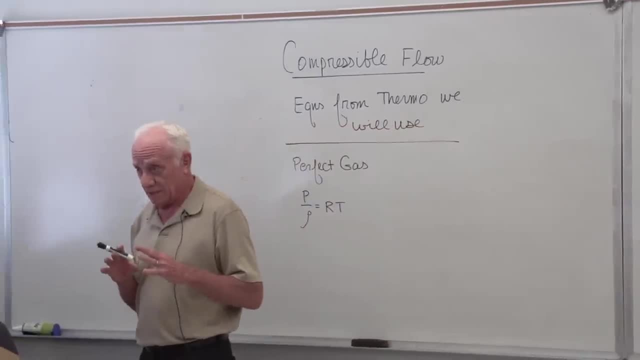 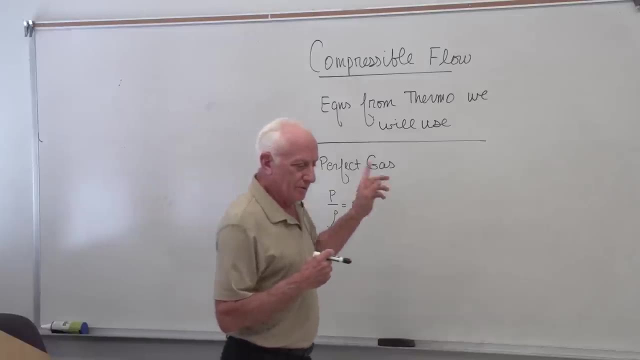 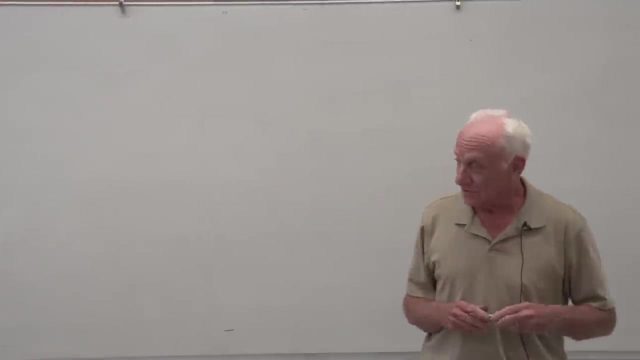 incompressible if the Mach number is less than about 0.3.. Less than about 0.3 the Mach number, But when you get to fluids 2 and you get to compressible, Compressible flow now is not an incompressible fluid anymore, It's a compressible fluid. 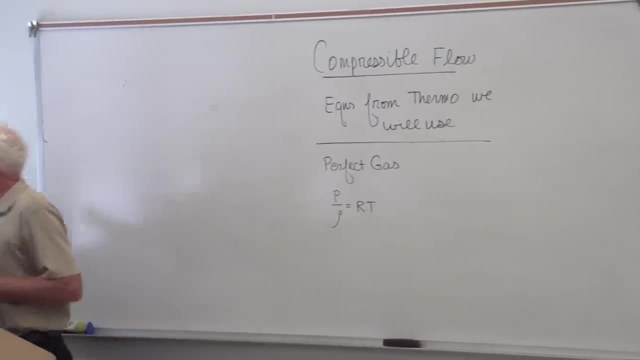 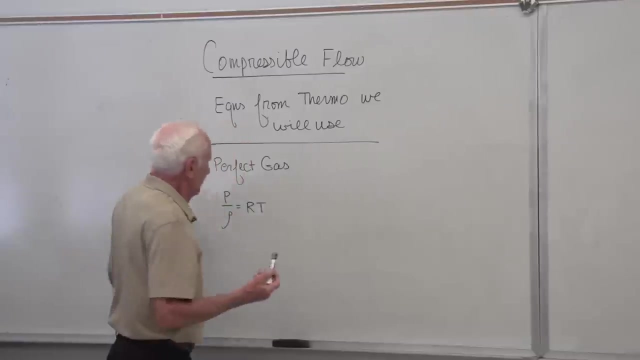 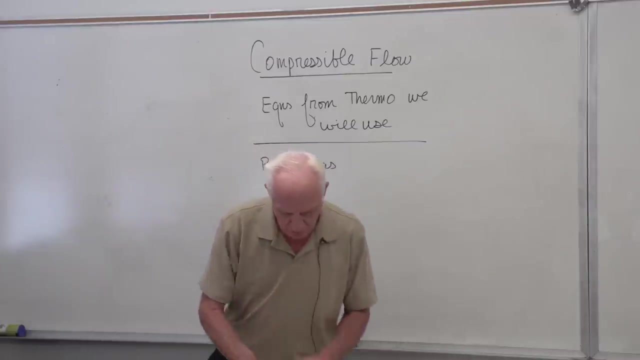 So we have to kind of shift gears in a way. We're going to pretty much be looking mainly at perfect gases. We know from thermal the definition in a perfect gas is one that obeys the perfect gas equation of state P over rho, equal RT. So I'll put down a number. 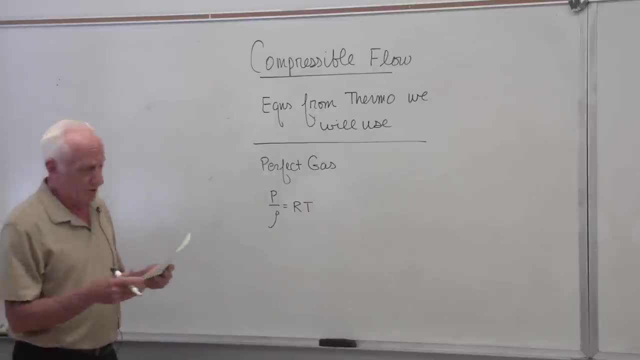 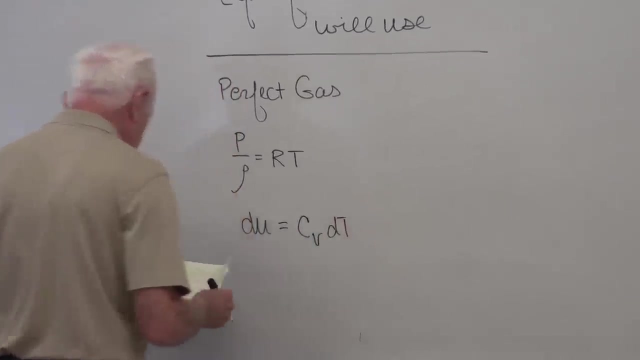 of equations which come from thermal that are going to be important in the compressible. Okay, Let's see the second one here. Yep, There it is. Change in internal energy is equal to C sub V DT, Specific heat of constant volume. And then we have 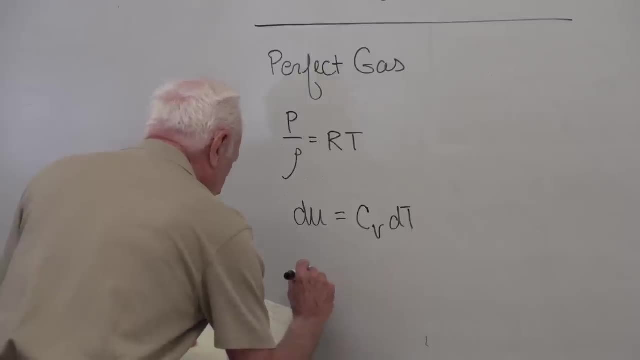 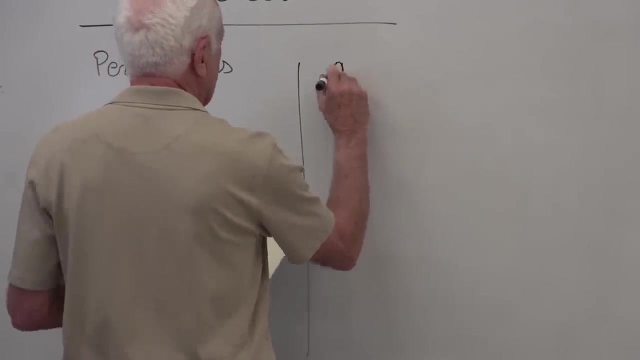 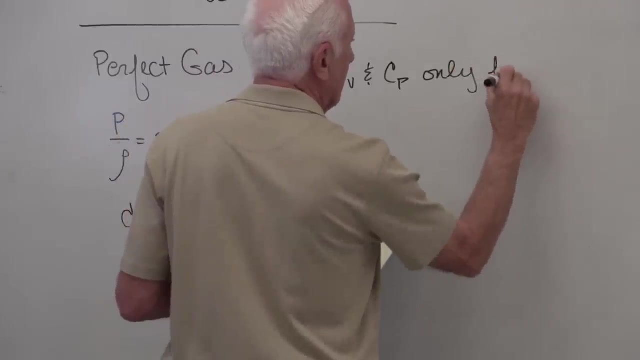 A sub V, DT. Okay, Okay. So we have H? U plus PV from thermal And we have- I'll put these just right here- C sub P and C sub V. only functions of temperature. Okay, Okay, Okay Okay. 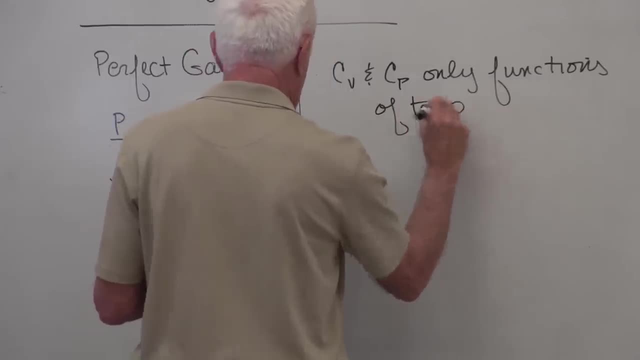 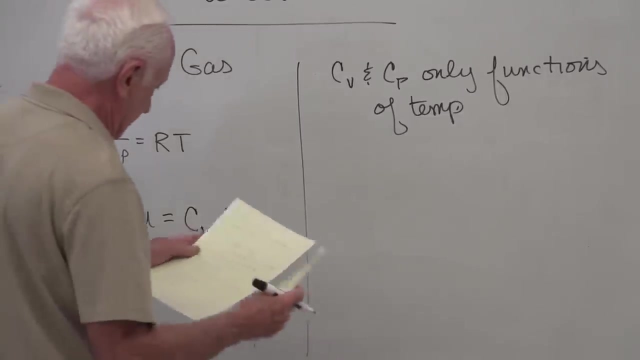 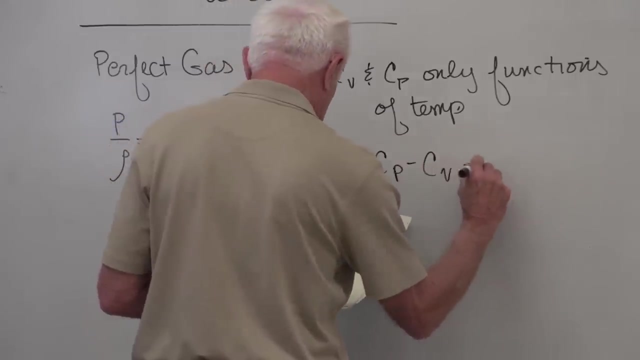 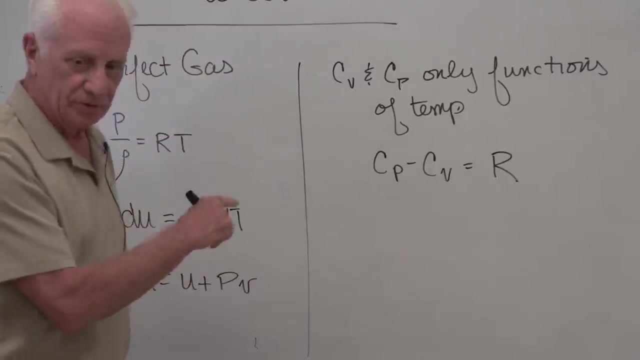 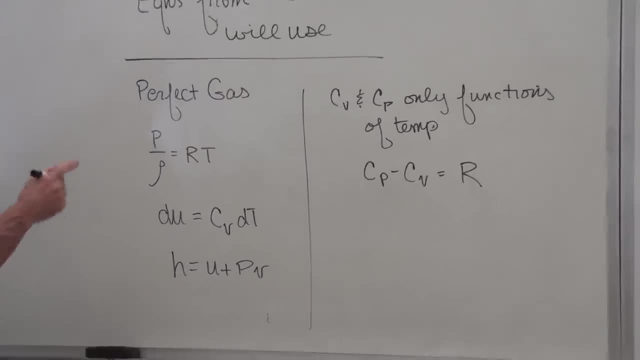 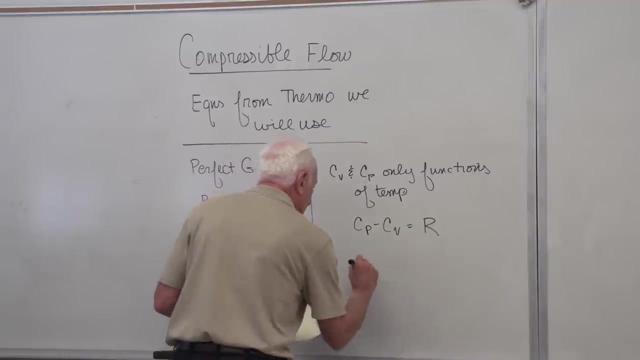 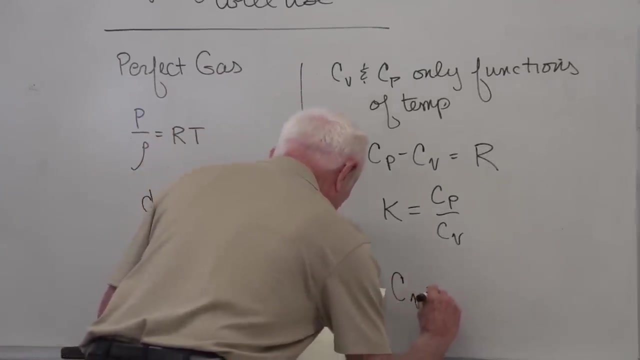 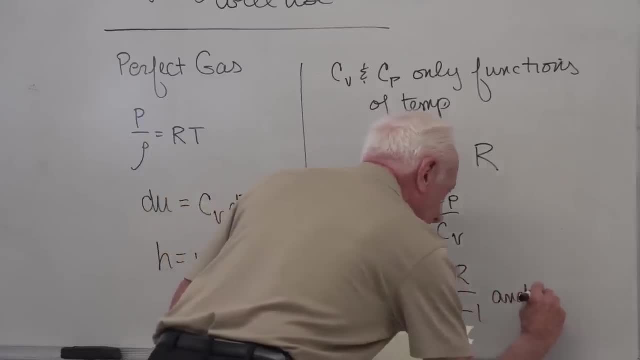 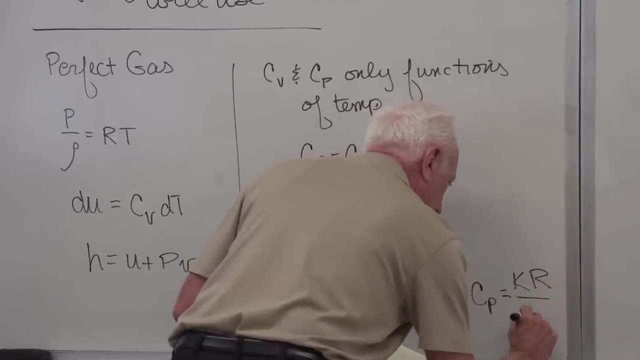 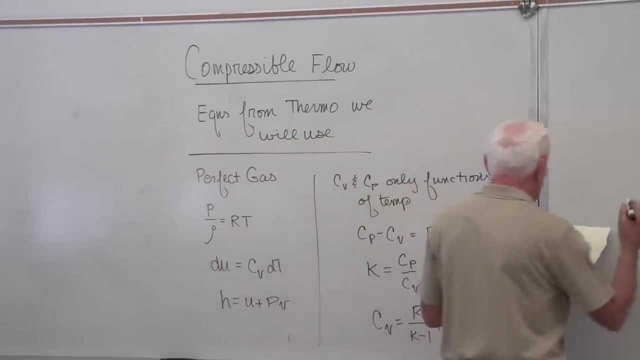 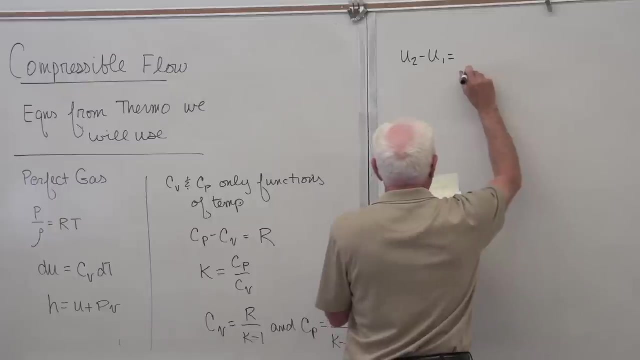 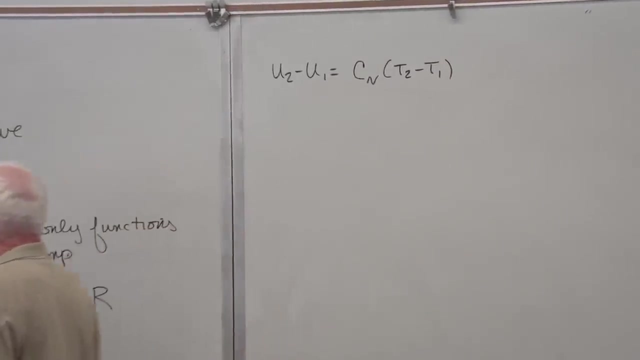 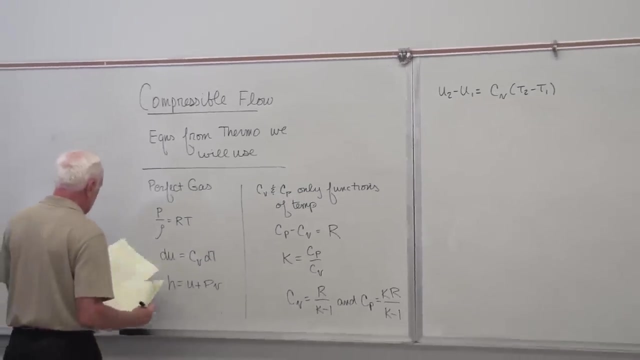 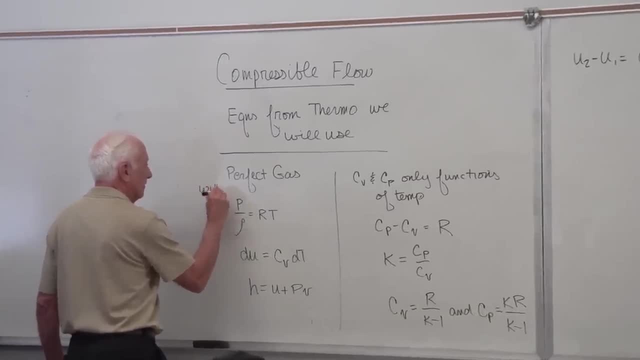 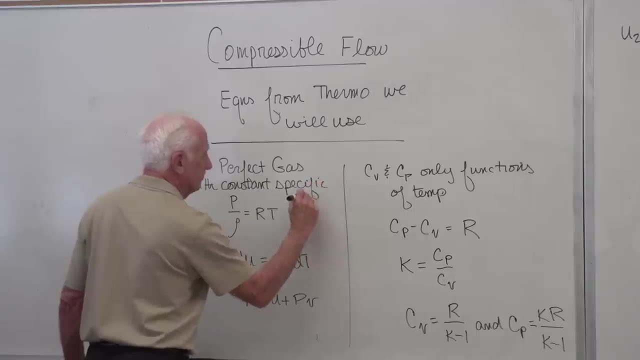 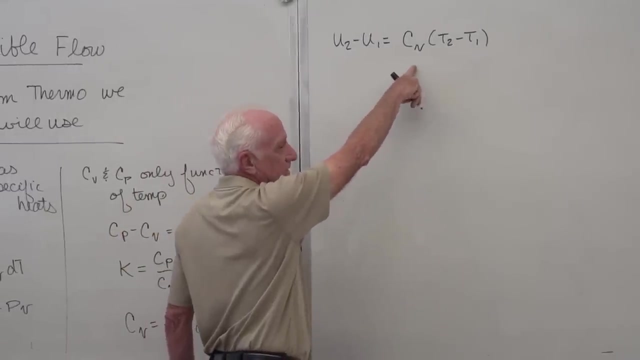 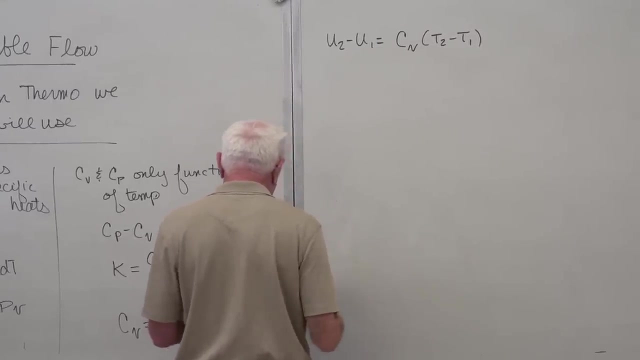 constant specific heats. so when we integrate C sub V, DT, the C sub V is constant. pulled outside the integral sign, we get that. Then we also have our equation for H that we're going to need H2 minus H1, C sub P, T2 minus T1.. 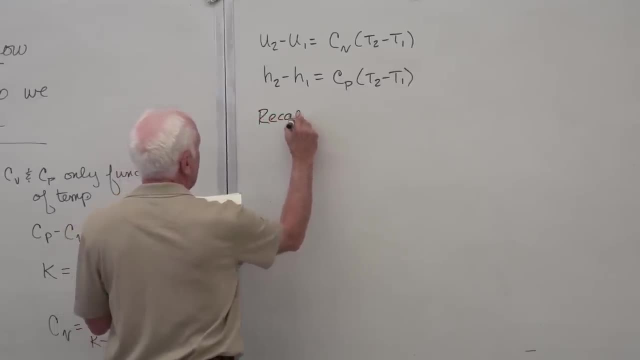 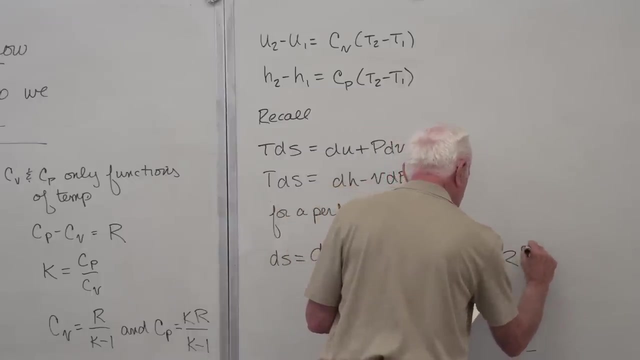 Then from thermal, we have the change in entropy, TDS and another form of it, and then we have, for a perfect gas, my DS, sol for DS or the other farm in terms of DH. 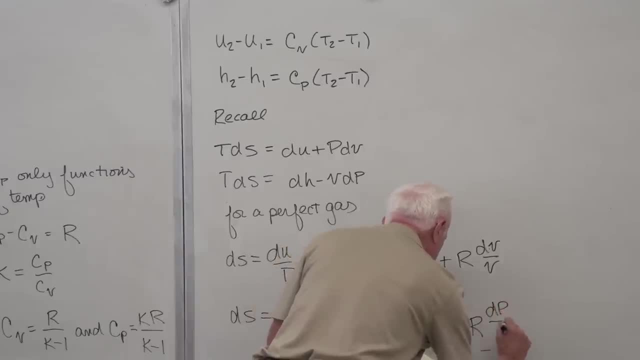 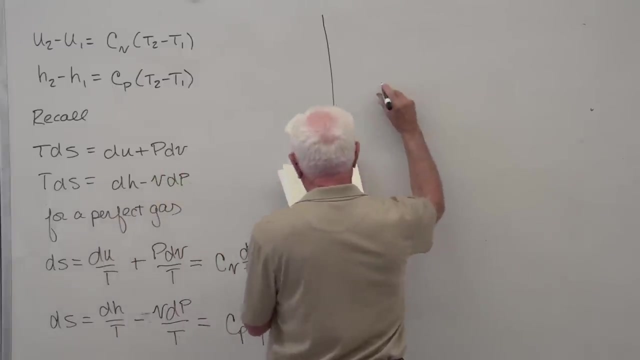 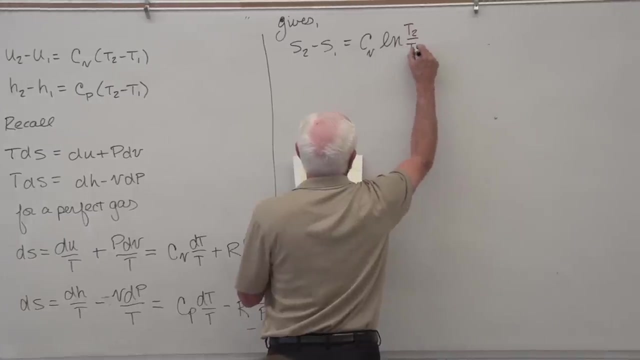 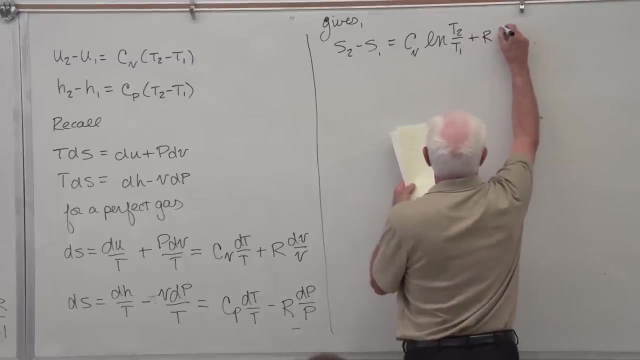 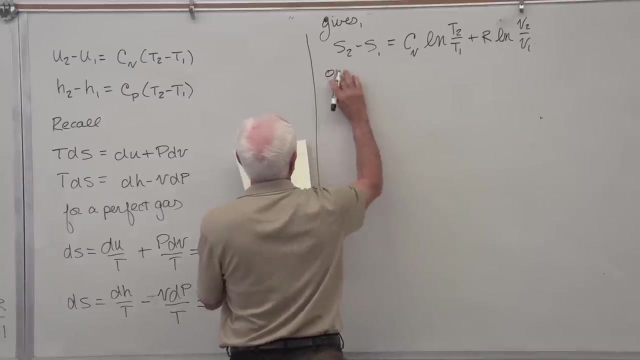 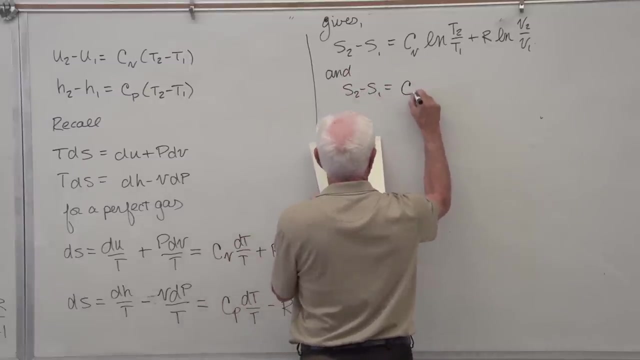 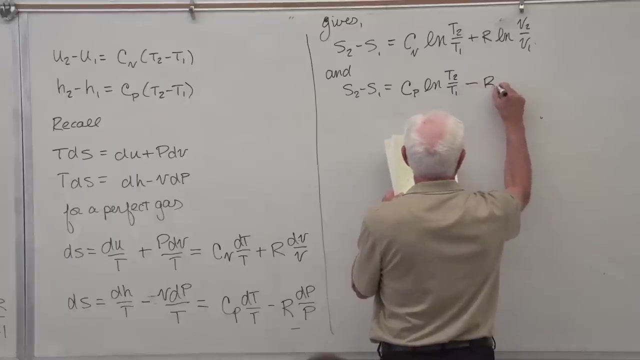 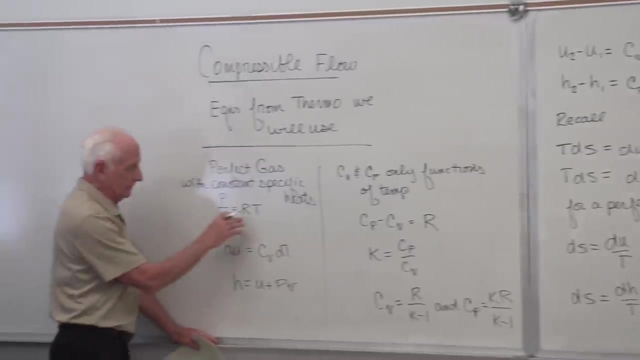 Okay, and then we integrate that DS, Temperature absolute. or in this farm let's just say, and We know in the perfect gas equation of state that temperature is absolute, that pressure is absolute, got to be. So everything you see here. 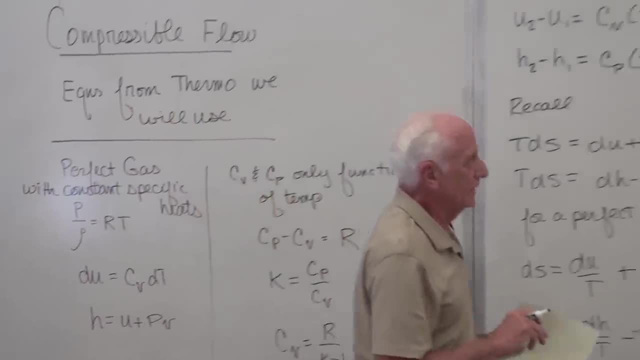 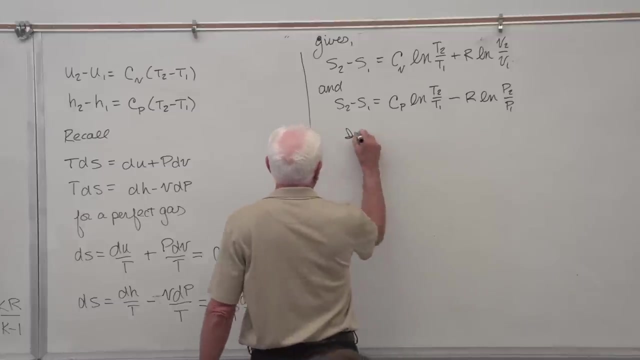 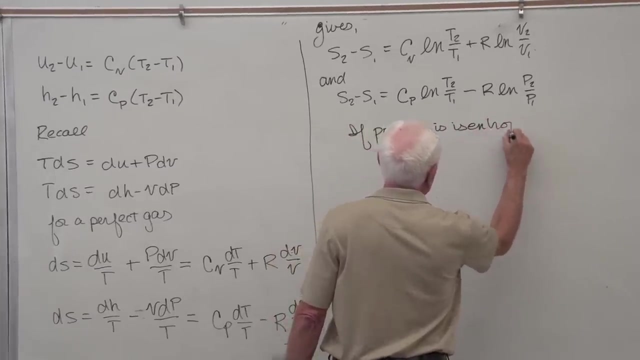 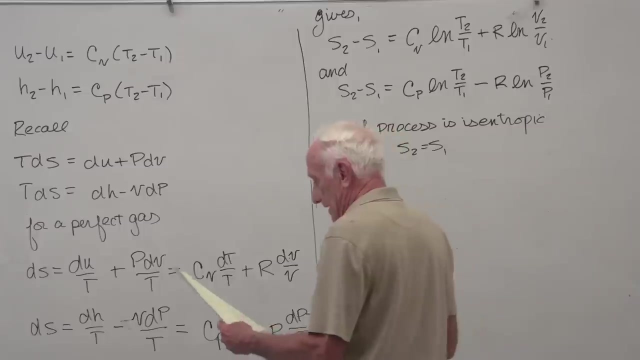 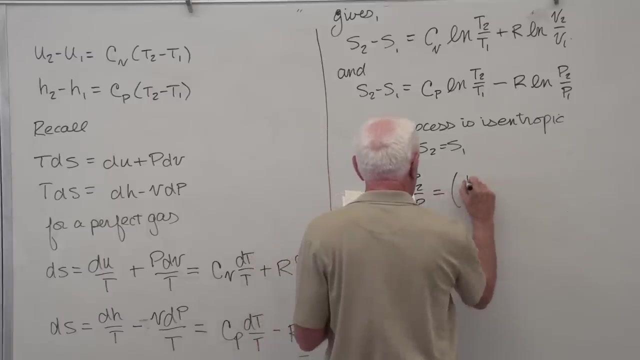 that pressure is absolute, that temperature is absolute, Not gauge, not relative. If process is isentropic, S2 equal S1.. So if that's the case, we get these equations. Okay, I think that's all we need there. 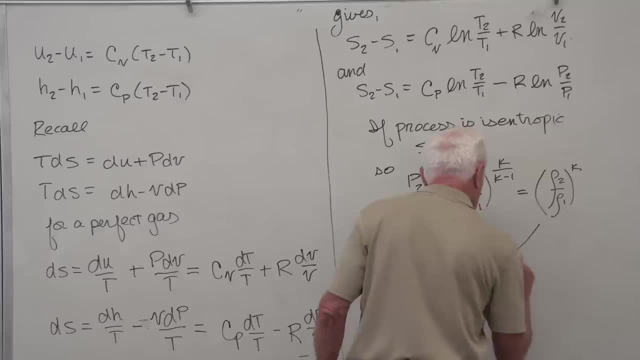 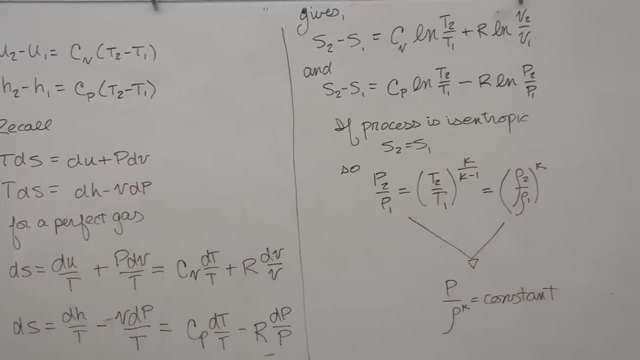 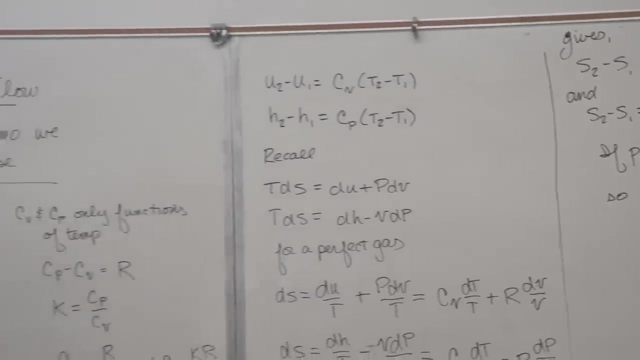 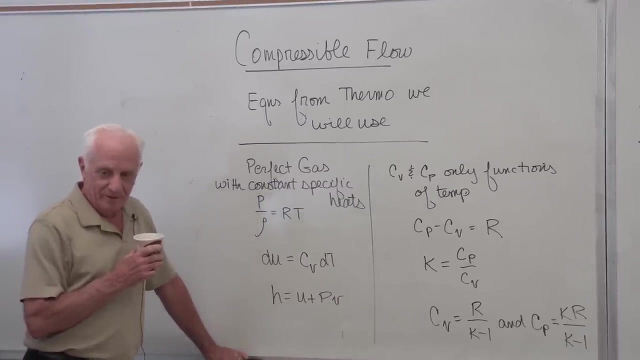 If you put these two guys together, you end up with this. That's a three-minute quick review of what we need in thermal for compressible flow. You probably these equations we'll use for derivations and for homework solutions and things like that. 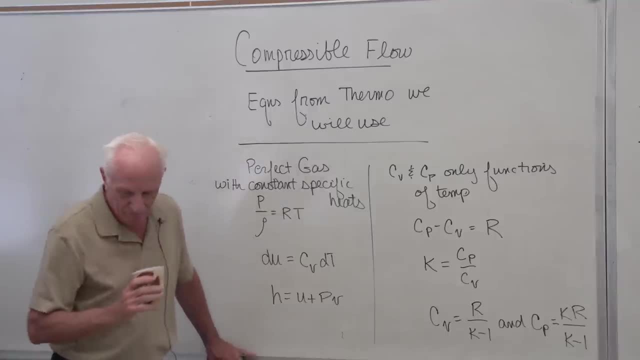 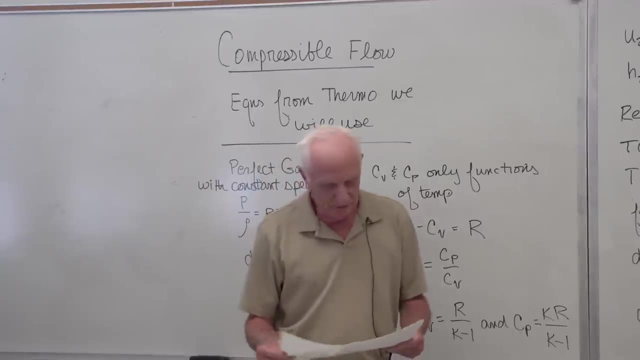 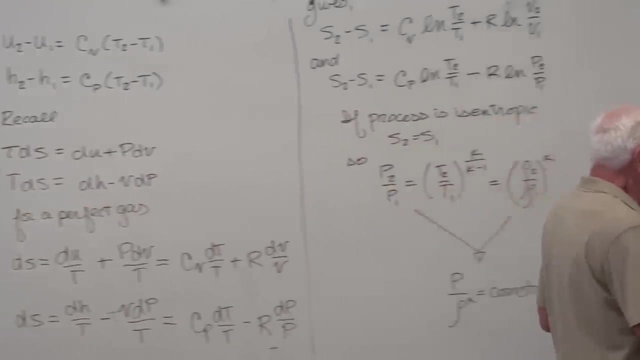 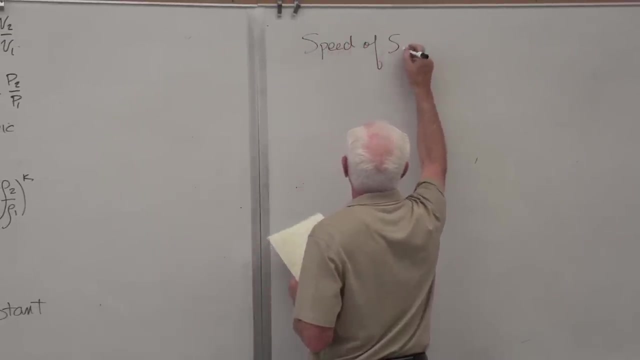 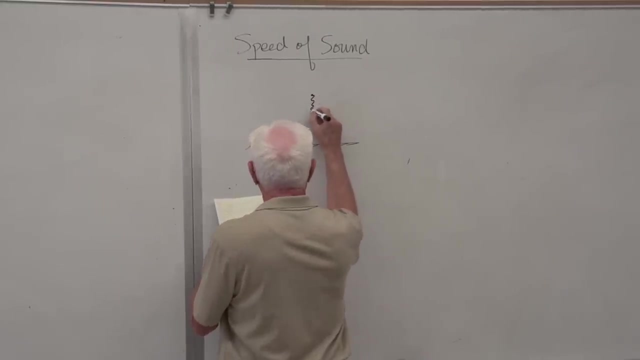 Okay, Now that gets us to the material we want to get to. The first thing we're going to do is look at the speed of sound in a compressible fluid, perfect gas. Okay, so here's the ground. This is a wave. 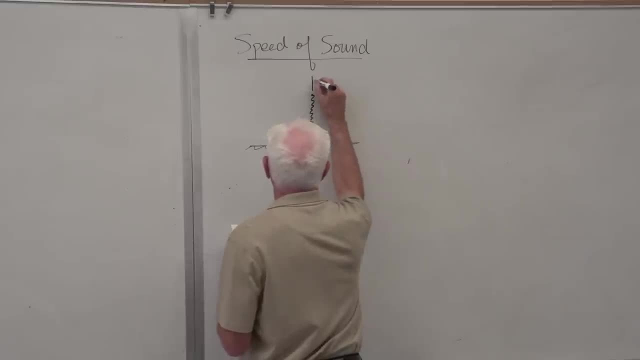 a sound wave C. It's moving in a region where the air is still, the velocity is zero, the density is zero, the pressure is P, So this sound wave is moving into a region of still air On the and, of course, 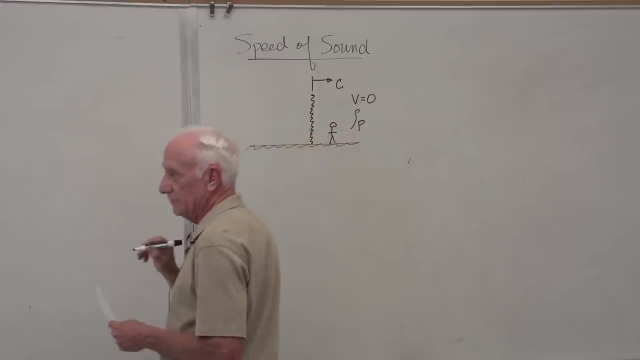 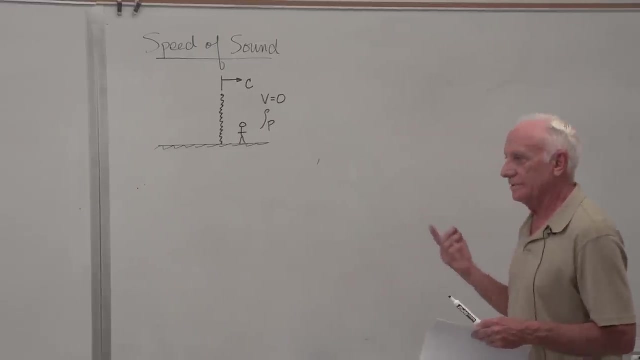 the observer is staying on the ground. Somebody does this. You hear the noise. How did you hear the noise? I don't see anything. How did it get to my ears? Well, there's a sound wave. That sound wave passed through the air. 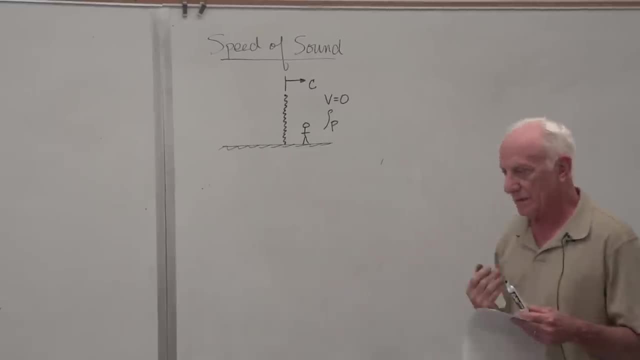 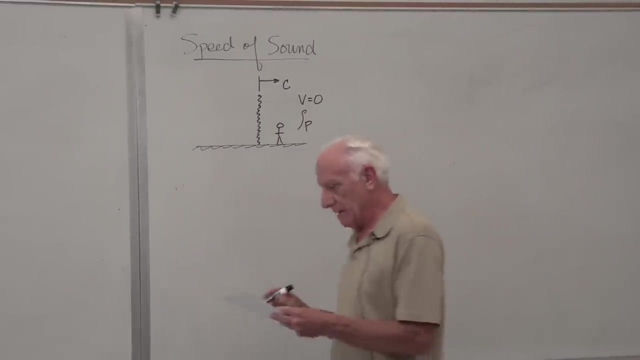 until it got to your ear, where your eardrum responded and you heard the sound. Okay, so you're the stationary observer and the sound wave went past you. On the other side of the sound wave, things change. The velocity now is a very small differential velocity. 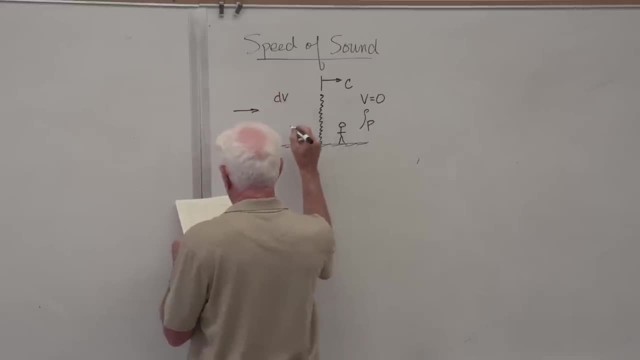 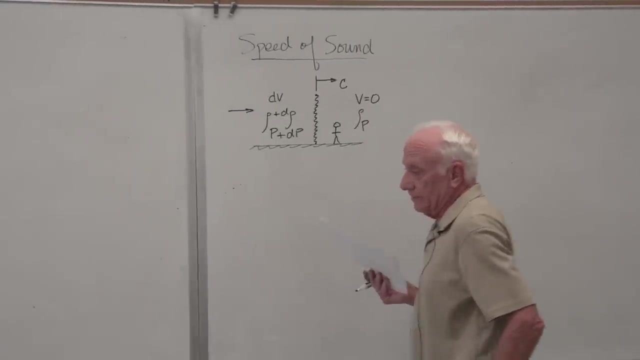 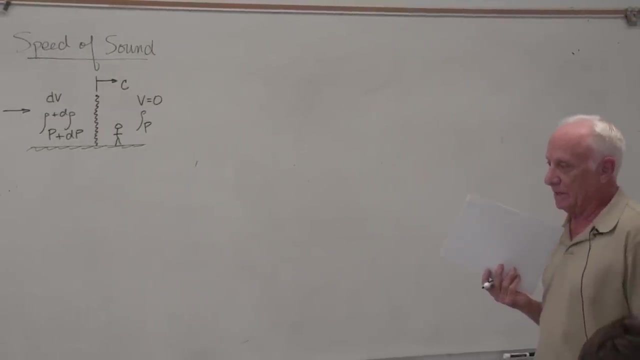 dV. The densities change, rho plus dRho. The pressures change, P plus dP on the other side of the sound wave. For the observer, this is an unsteady problem. The sound wave passes, Wait a few seconds. it's quiet again. 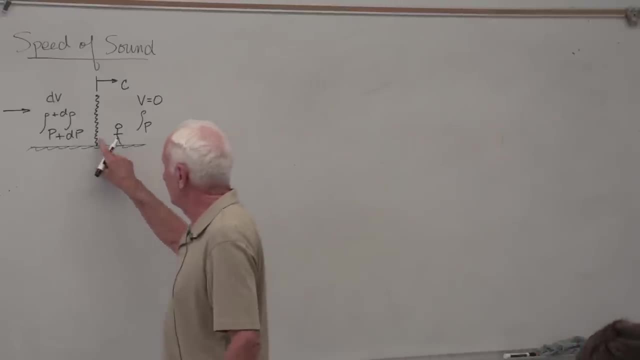 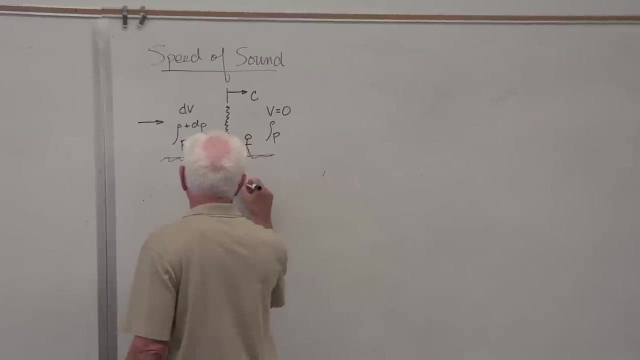 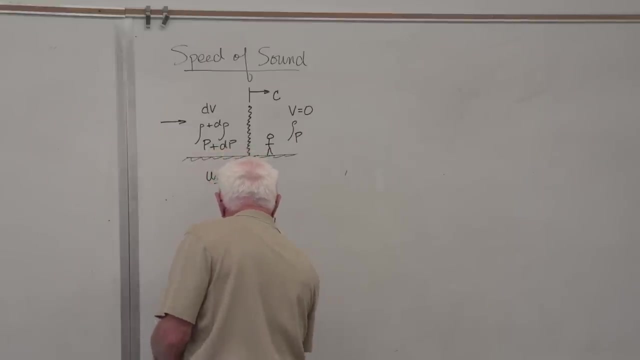 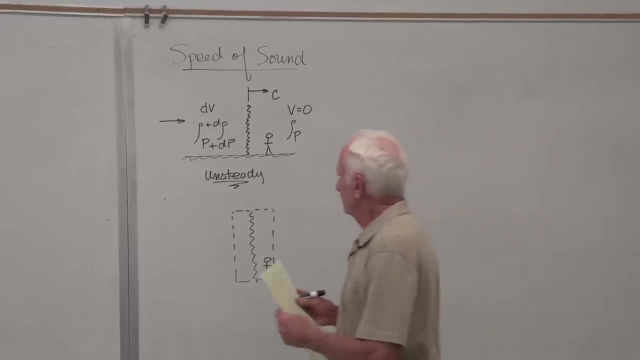 To make it a steady process, we attach the observer to the wave. Okay, this is unsteady. So now we attach the observer to the sound wave And the observer is standing with this. Okay, I'm the observer, I'm sitting on the sound wave. 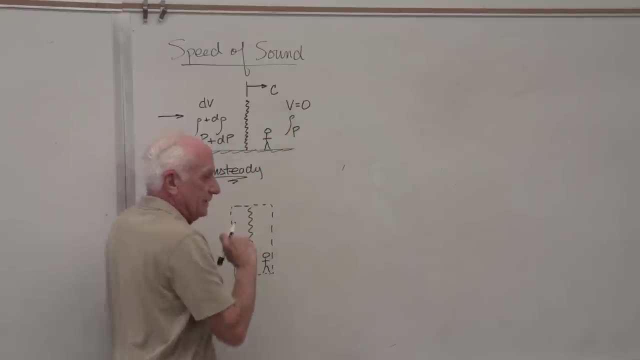 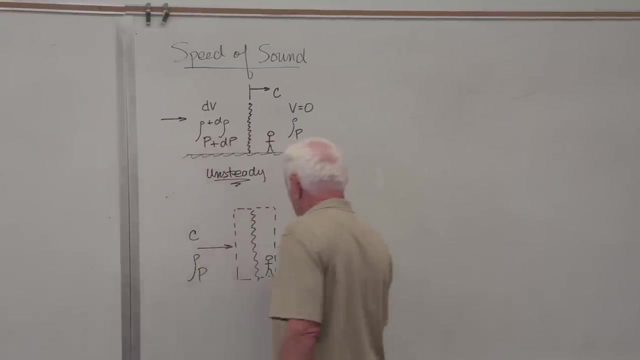 I see air approaching me at that speed c, where c is the speed of sound. So I see air approaching me at a speed c, The density is rho, the pressure is P. What's leaving the underside of my control volume? the dashed line is a relative velocity c minus dV. 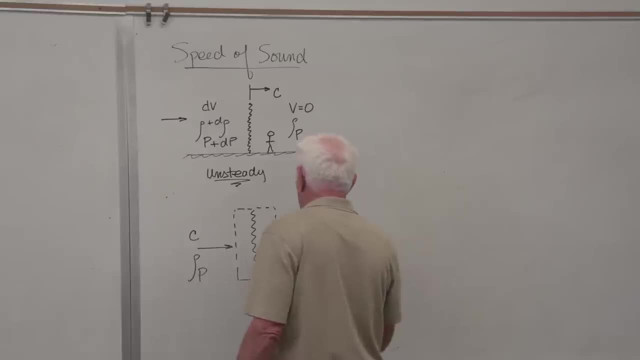 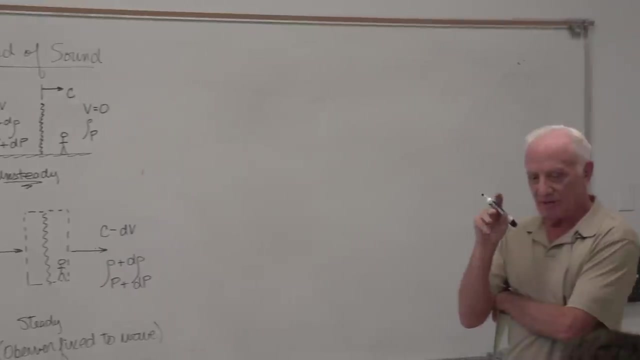 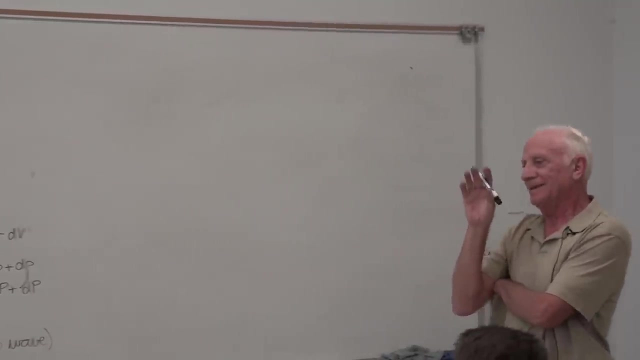 The pressure there is the same and the density is just like the above picture: P? rho plus d, rho, P plus dP. Now, this is steady Observer, fixed to sound wave. Our textbook calls the speed of sound a, Other books call it c. I like c. 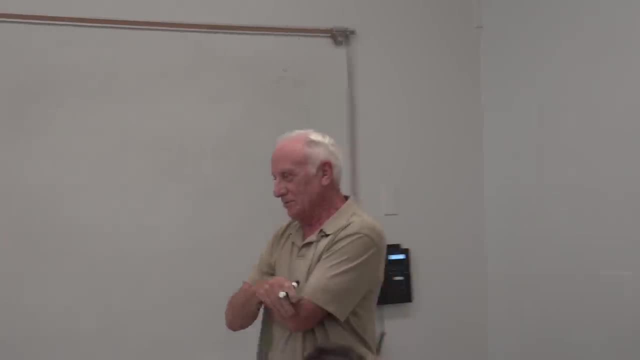 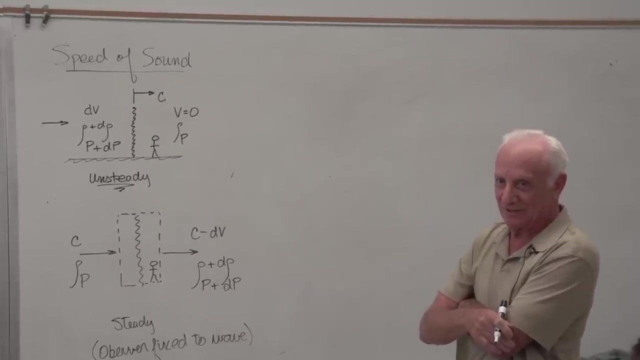 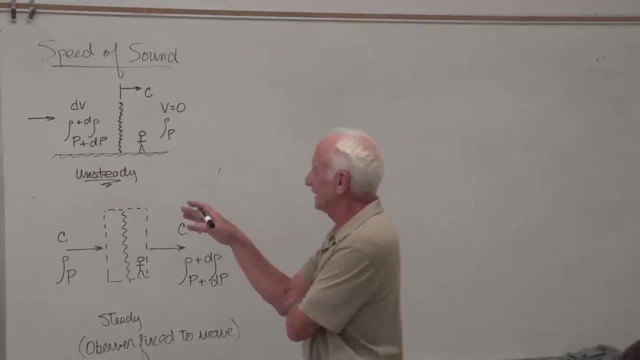 Because a can mean when you write a sentence, a can mean the speed of sound, or it can mean a in the sentence: Okay, apples and oranges. So when you read your textbook, you're going to see the symbol a, but I like to use the symbol c. 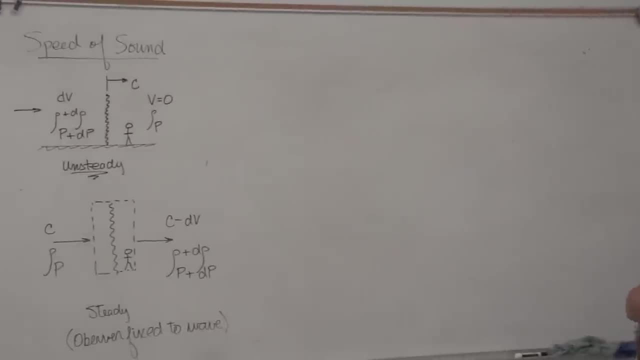 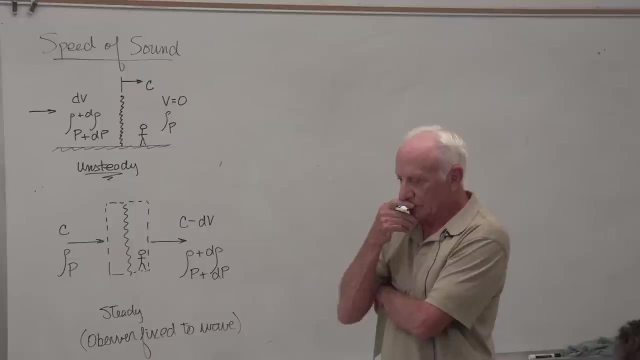 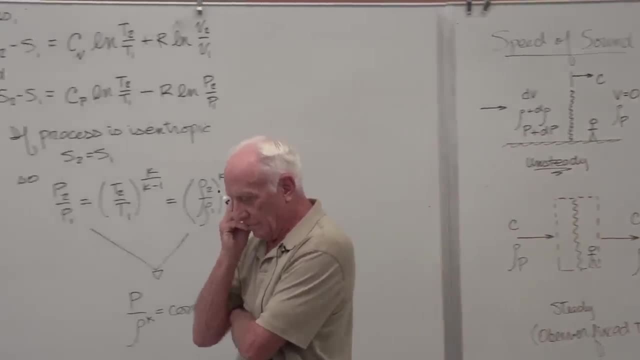 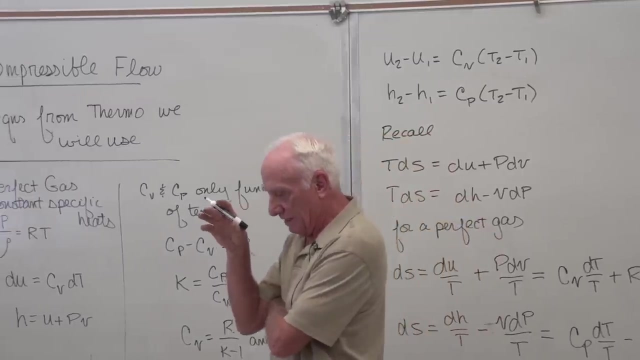 Sound wave is a very weak wave. It's a weak wave. What does weak wave mean? Well, you can look at two kinds of waves. Number one is a sound wave. When I talk to you, I don't blow your eardrum out. 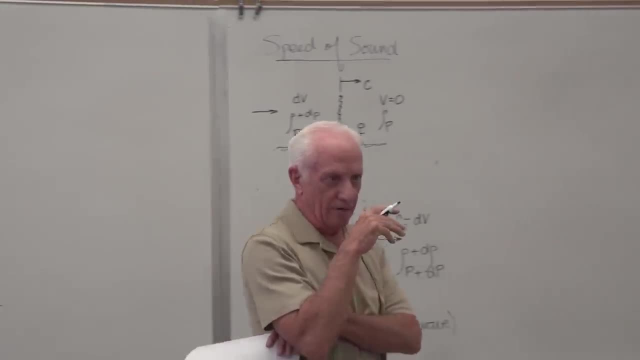 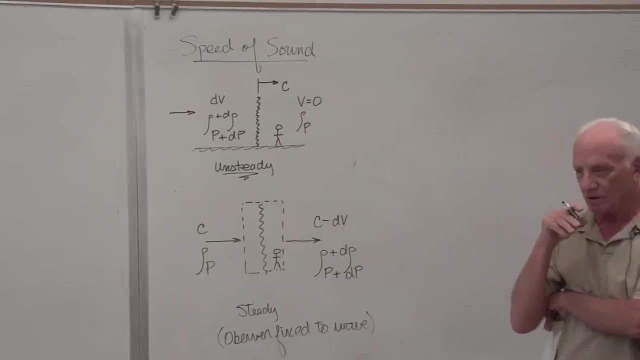 You're on the deck of an aircraft. carrier F-18 flies over 100 feet over the deck. It'll blow your eardrums out. That's not a weak wave. That's a very strong compression wave. So right now we're talking about sound waves. 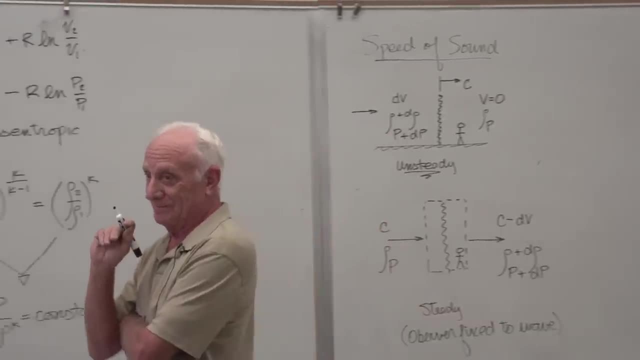 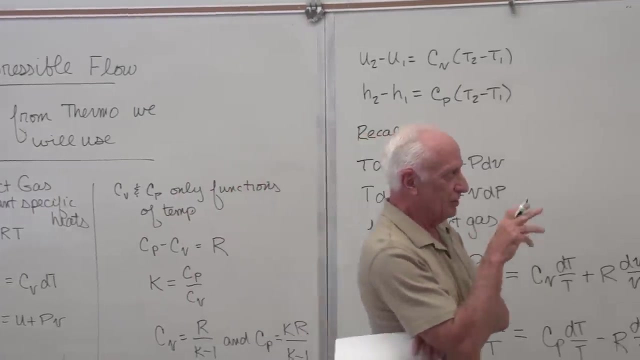 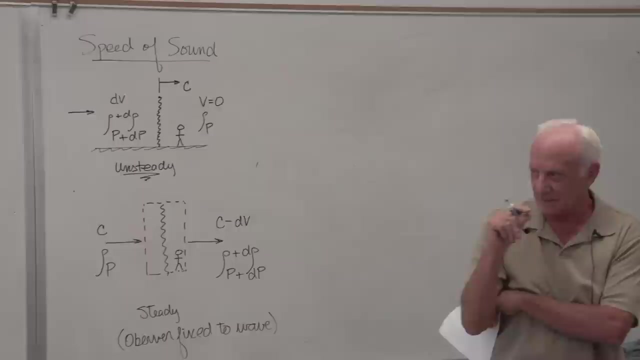 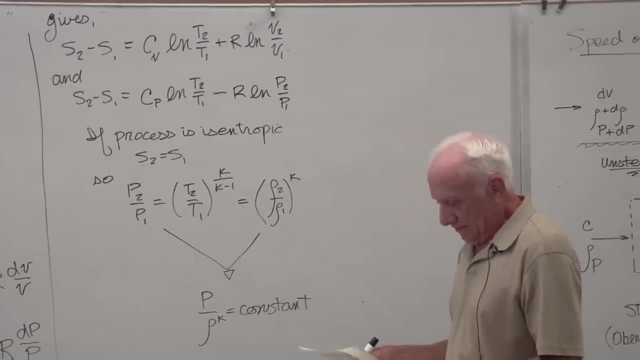 Later on we'll talk about shock waves, because they're strong, Big change in pressure. In this one there's a small differential change in pressure, a differential change in velocity, a differential change in density- small. Okay, Yes, the pressure difference is really really small in there. 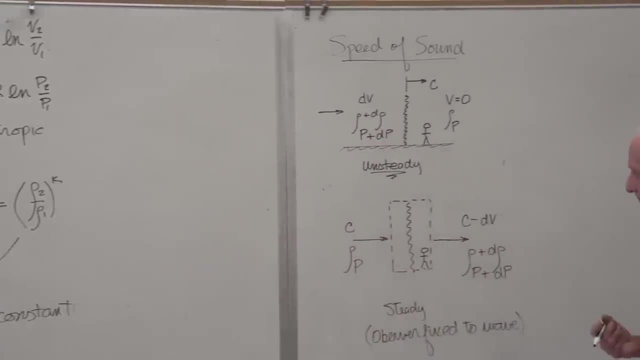 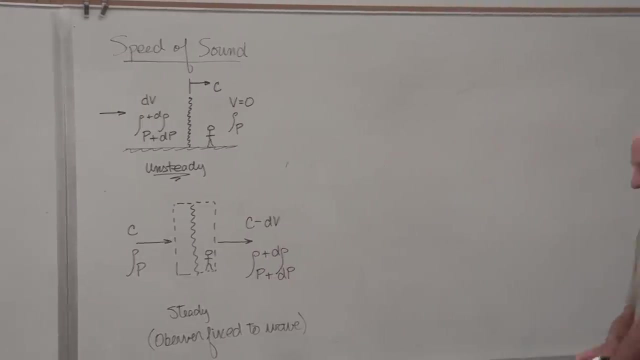 They pass through our ears pretty quickly. Bam and it's done, But we're riding with it now. Okay, So there's that picture. What are we going to do? Okay, Same old, same old Fluid mechanics. We're going to apply continuity and momentum. 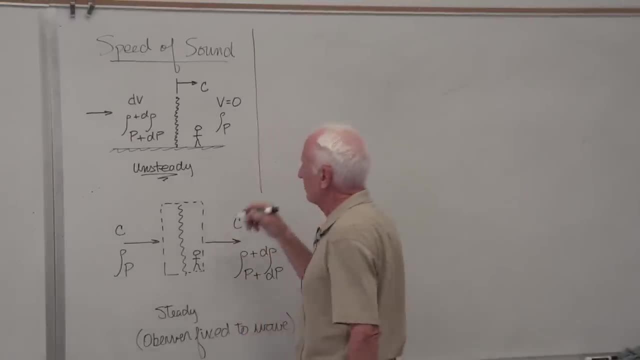 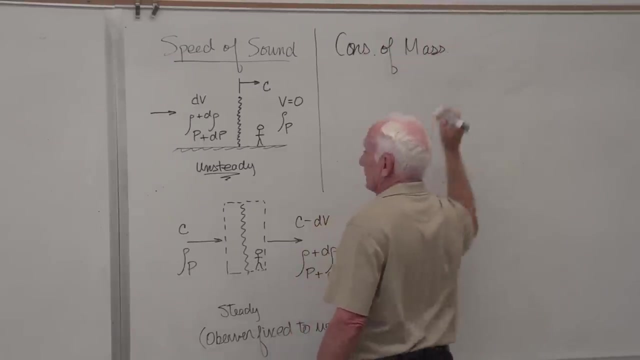 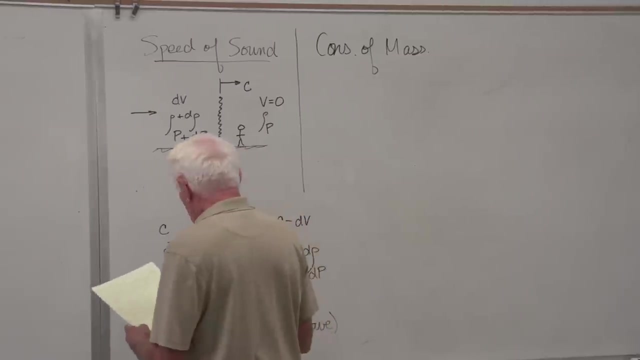 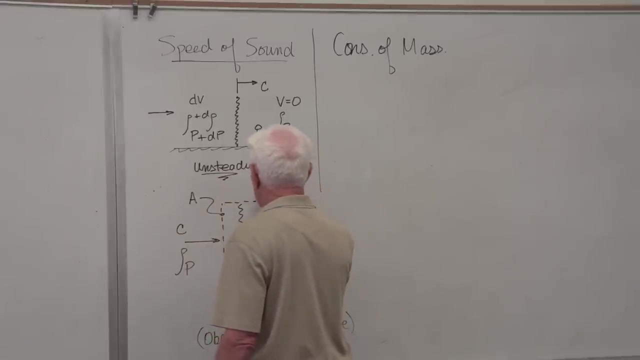 All right, First equation apply: continuity for that control volume. conservation of mass Steady state. What comes in the left goes out the right. Okay, I'm going to call this area on both sides A. This is my control surface. 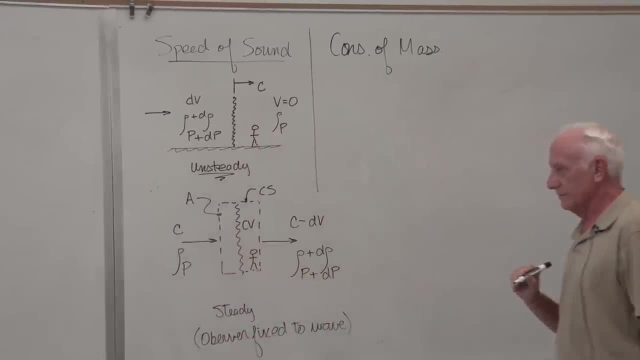 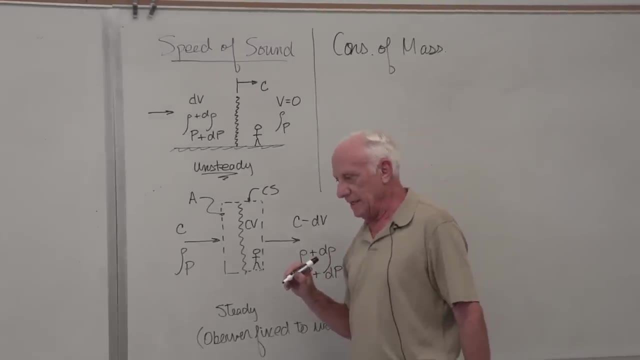 This is my control volume. There's the area A, normal to the velocity C. What comes in the left? we know M dot in, equal M dot out. What's M dot Rho, Av, Uh-huh Rho A. velocity C. 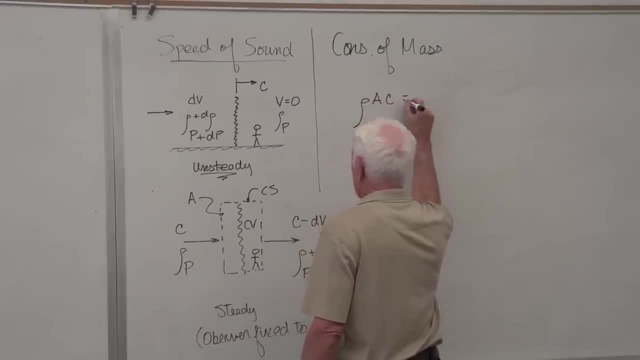 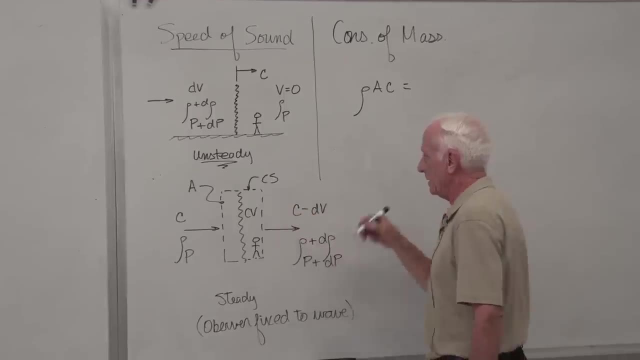 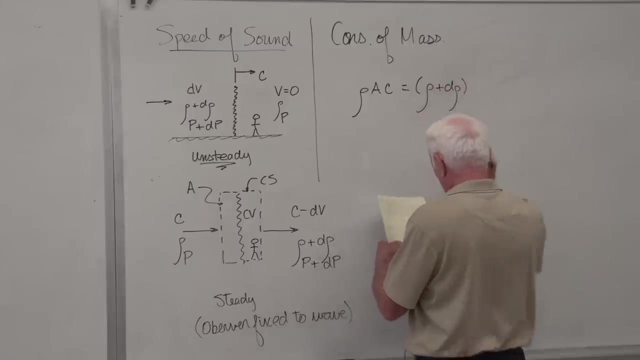 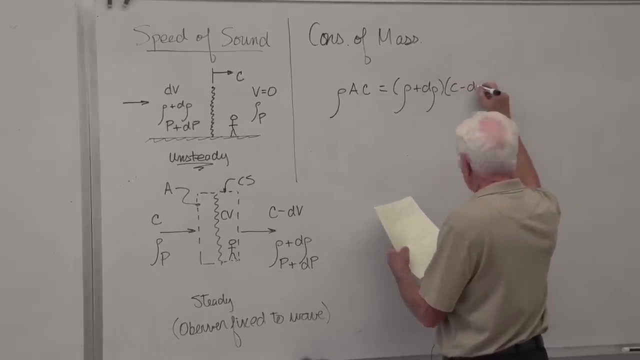 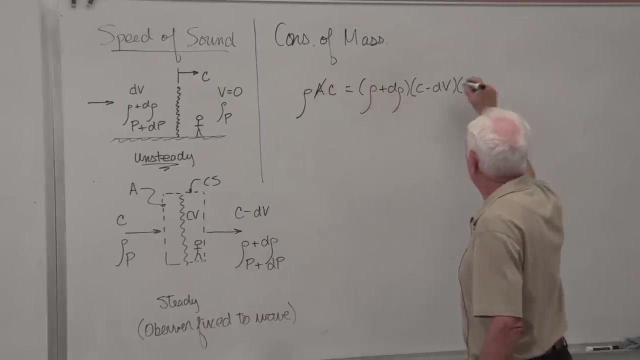 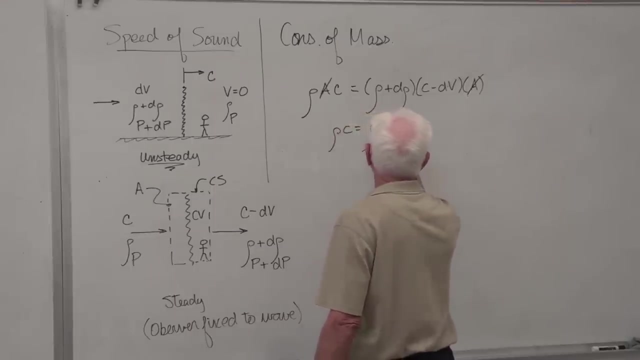 Okay, What goes out over here? Density here, Velocity here, Area here. I think I put up: Yeah, That's okay, Rho plus D, rho C minus DV. Sprinkle, Okay is A. Of course the area on both sides cancels, cancels, gone. Rho C equal Rho C. 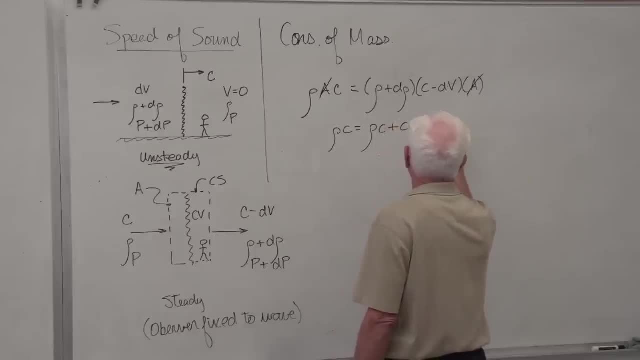 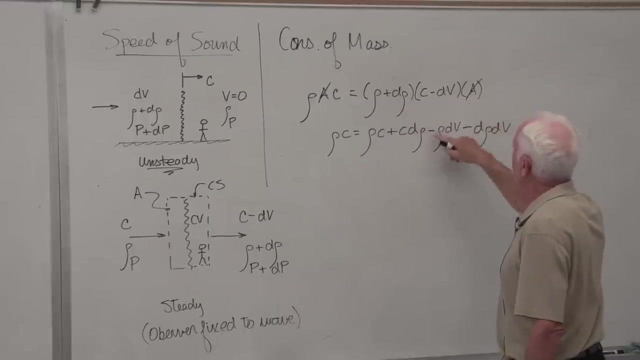 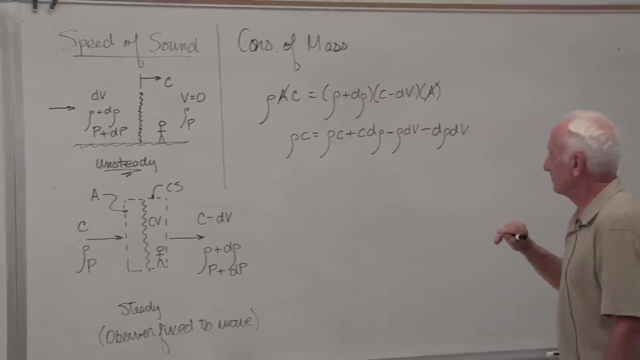 plus C D Rho minus Rho D V minus D Rho D V Rho. times C here Rho. times D V here minus sine C times D Rho here plus sine D V D Rho minus sine: OK, Both sides. 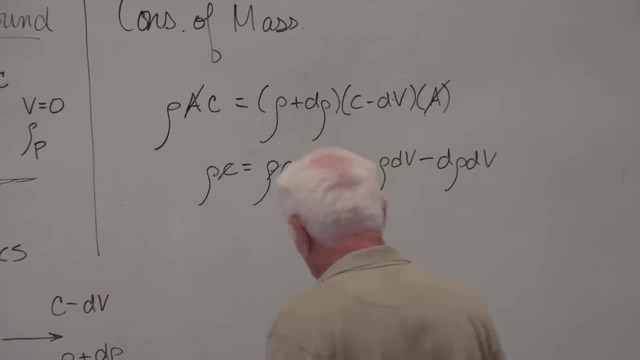 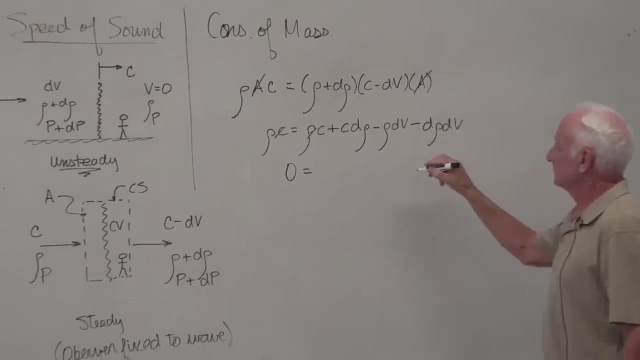 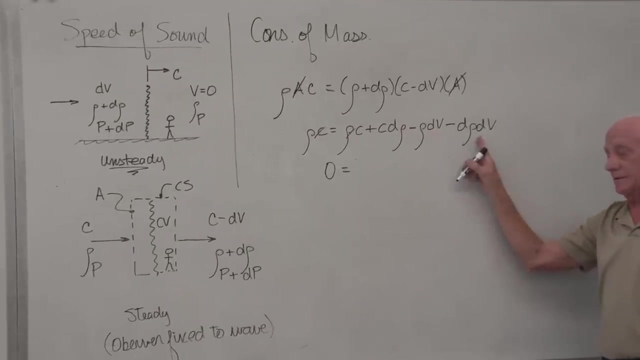 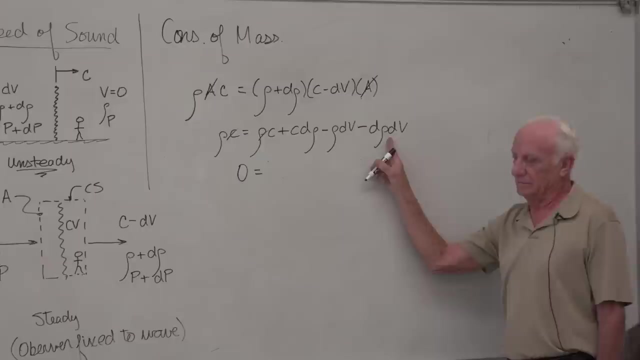 of the equation: cancel, cancel, Zero, equal. This guy has a differential D Rho, He's got a differential D V. He's got two differentials: D Rho, D V. If this number is small- and that's small, this guy is really small- Two small numbers. 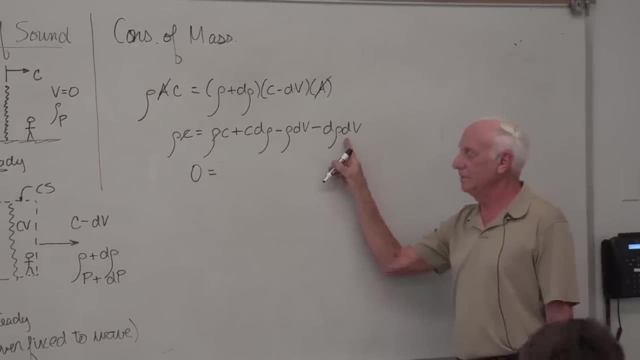 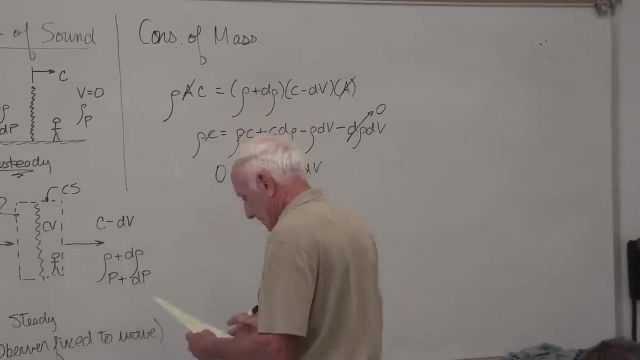 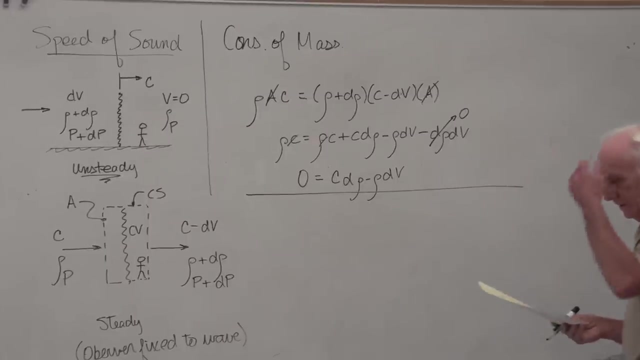 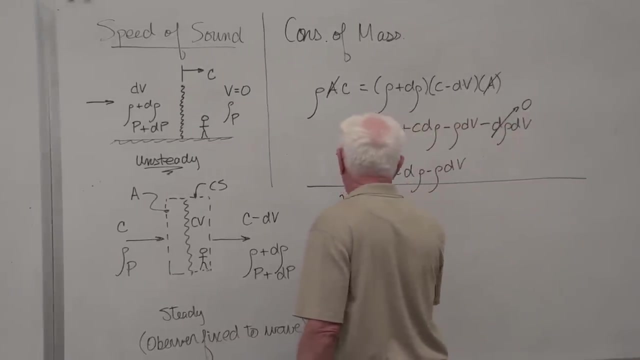 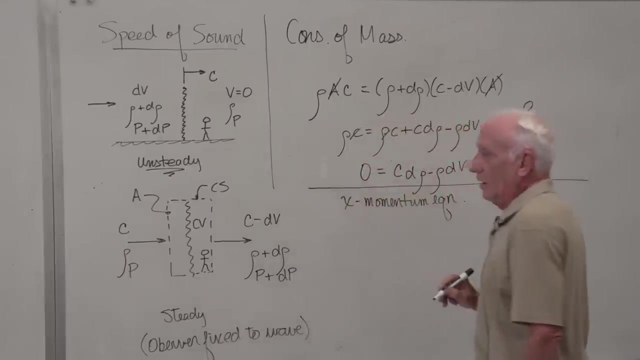 multiplied together. I'm going to ignore them, right? That's typical for what we do. We say: let's ignore higher order differentials. OK Gone, We're left with C D, Rho minus Rho, D, V, OK, Now. OK, That's conservation of mass. I'm going to write X momentum, OK. First, 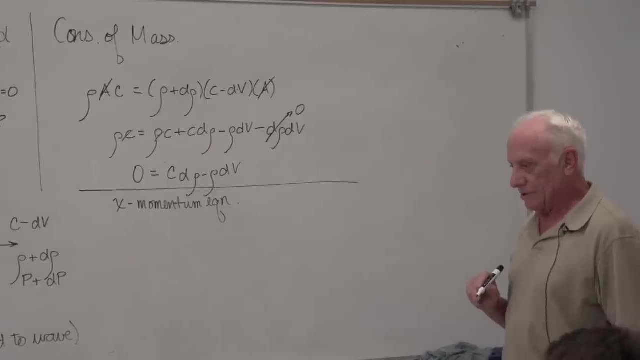 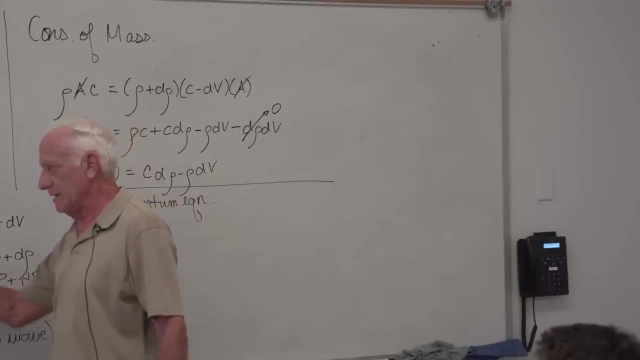 thing. left hand side momentum fluids. one Summation of the forces acting on the control surface. OK, Pressure force times area. Pressure force times area. Pressure times area gives me the pressure force. OK, Which way is it pointing To the right? 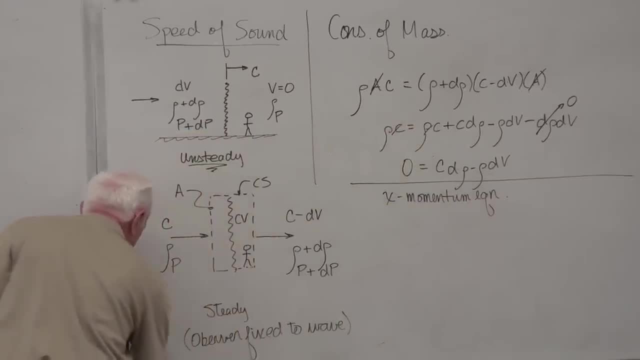 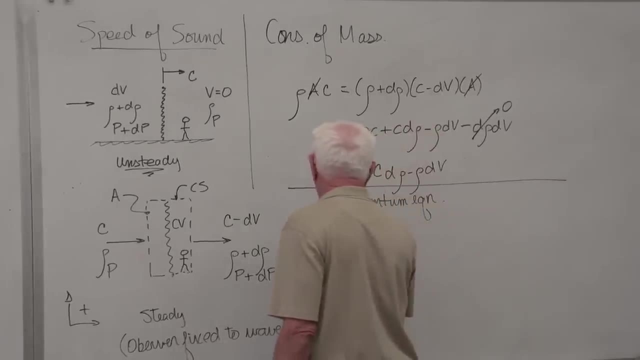 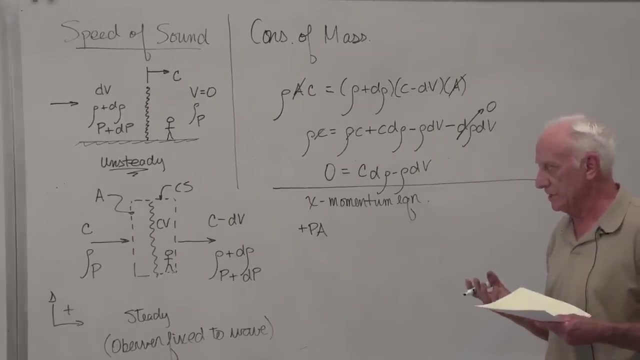 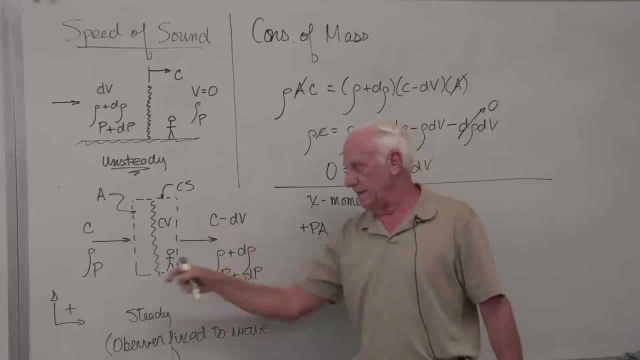 I define my coordinate system: positive to the right. positive up P times A On the left. pressure force is always a compressive stress on the control surface. It always points inward to the control surface. The pressure force on the right points this way: Negative. 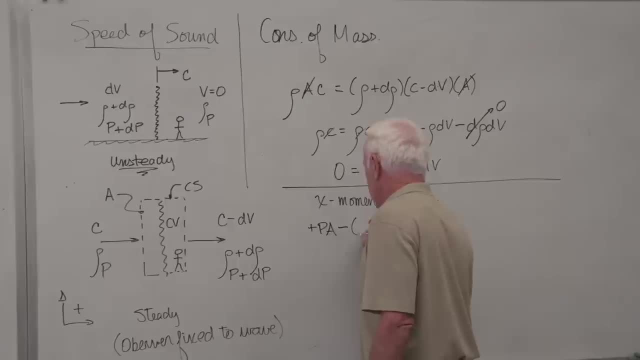 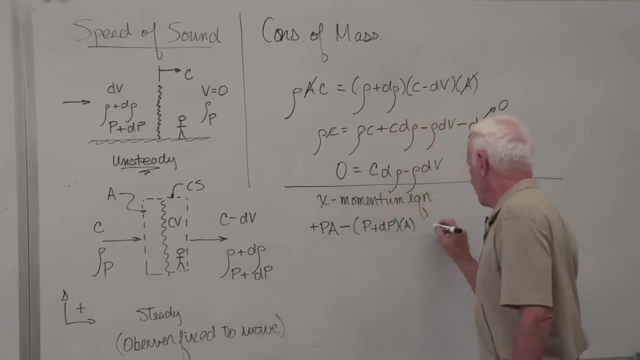 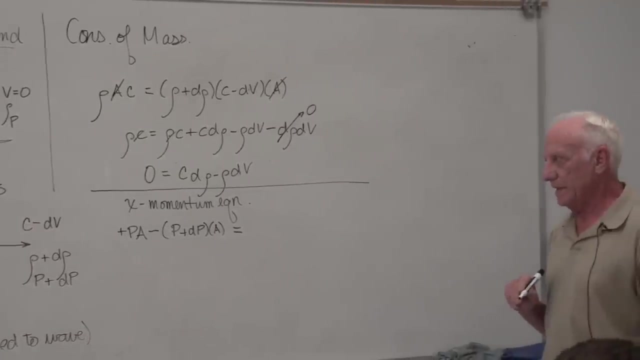 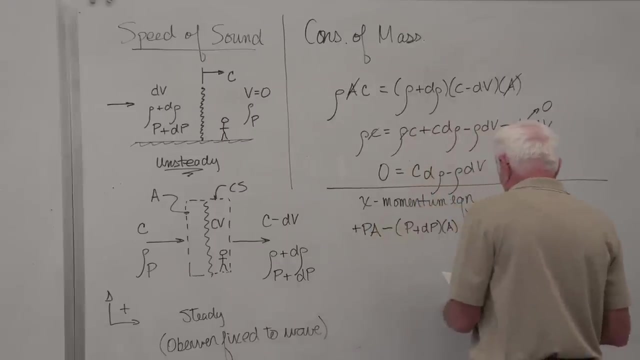 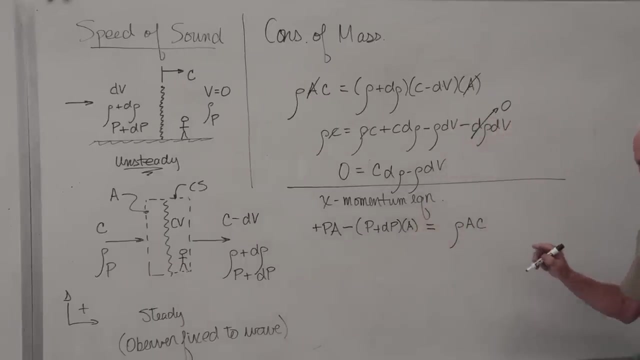 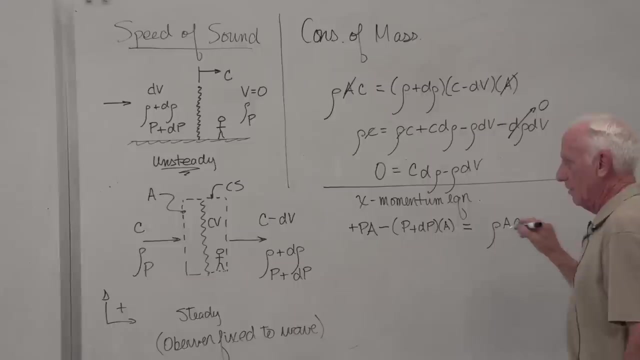 Negative Pressure: P plus DP Area A. Pressure force Equals the right hand side. Momentum flux: M dot times velocity. coming in, OK. Coming in M dot times velocity, OK. Rho A C, That's M dot. M dot is Rho times A times velocity. Rho times A times velocity. 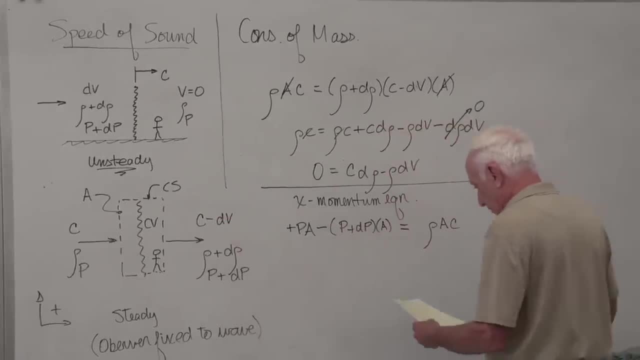 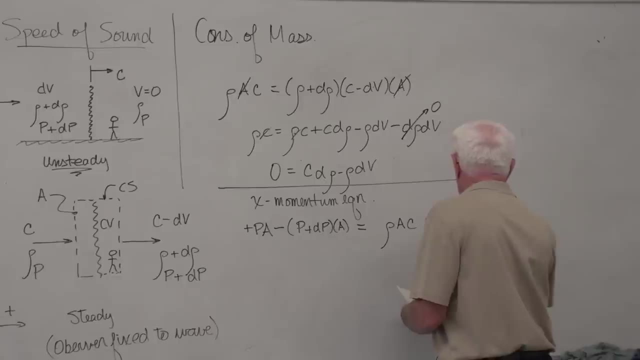 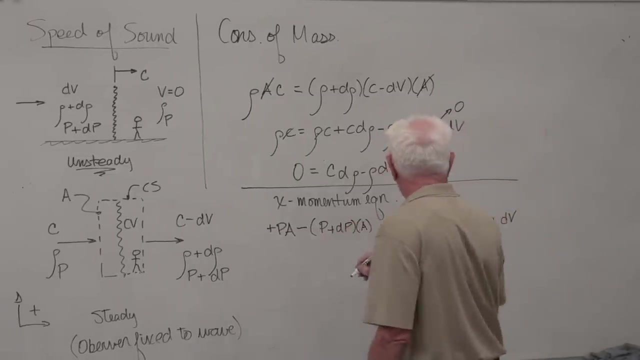 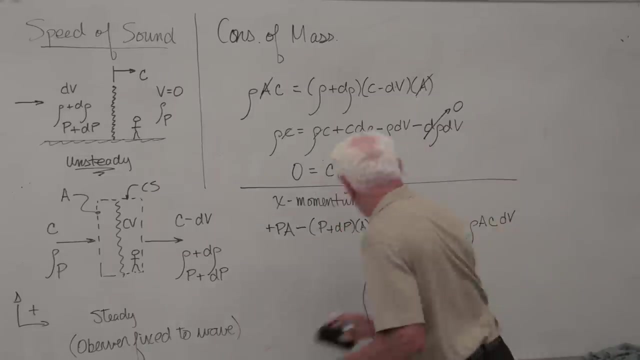 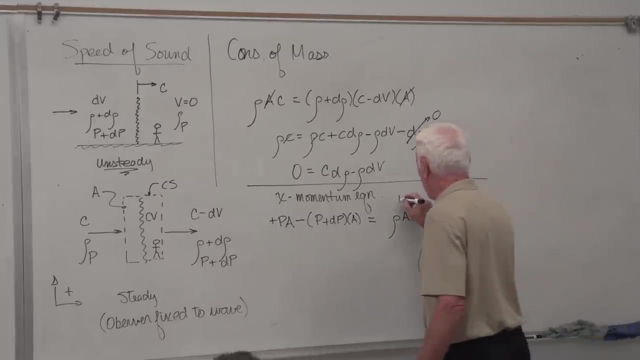 Going out. OK, Rho. of course changes Rho A C times the velocity Velocity DV. OK, OK, C minus DV. pardon me, This is M dot velocity in, M dot velocity out. OK, That's how you write. 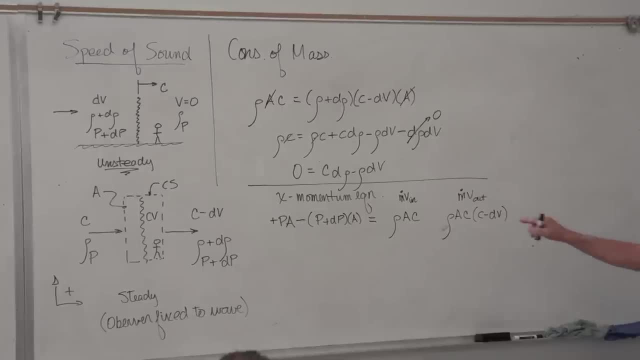 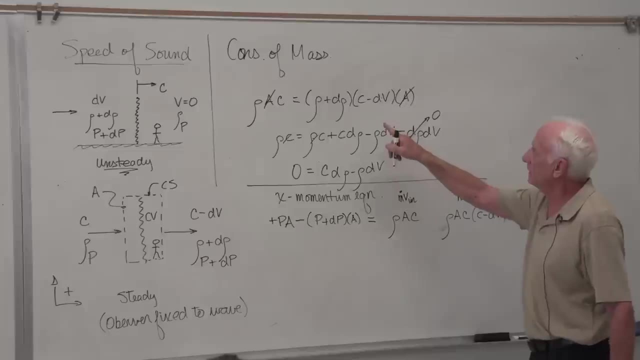 momentum. Why isn't this rho plus D rho And why isn't that the velocity C minus DV? Because It's right up here: The mass that comes in the left goes out. the right M dot on the left, equal M dot on the right. 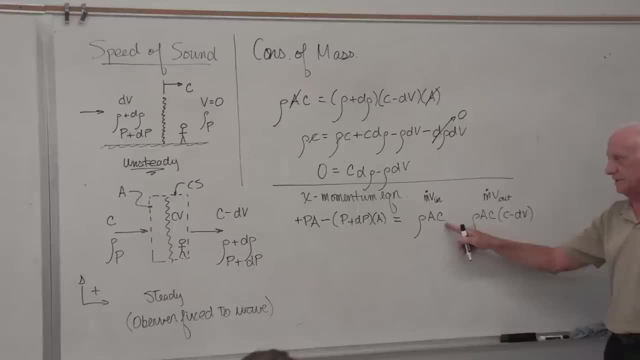 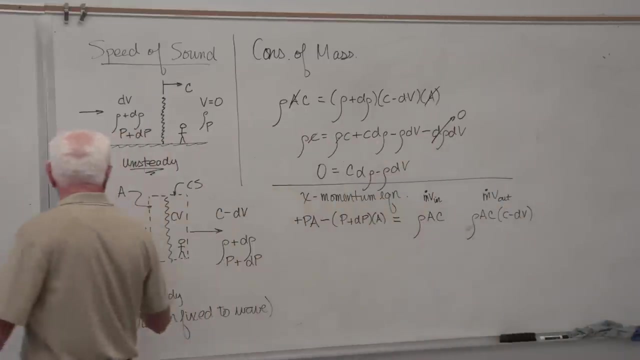 Take the easy way out. What's M dot in the left- Rho AC. What's M dot out the right Rho AC? Here's where people always mess up. What's the sign? Which way is the velocity vector to the right positive? 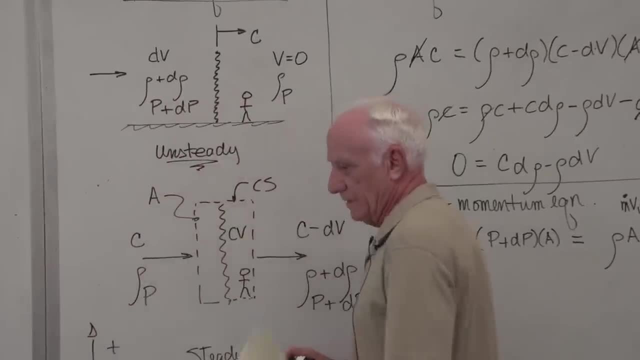 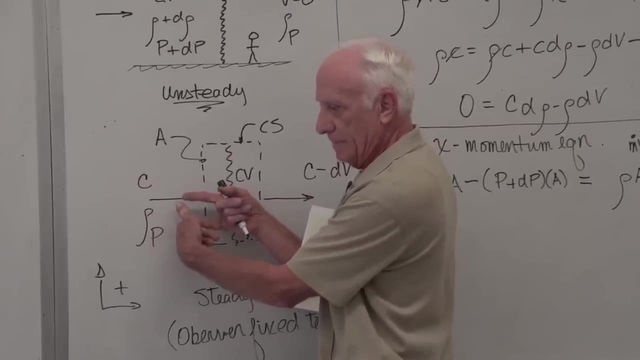 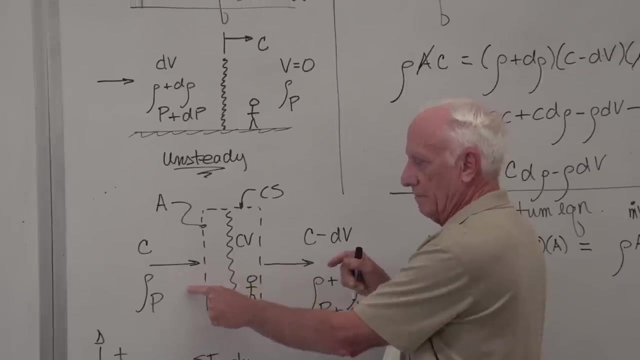 Which way is a dot product of the velocity vector and the area vector? The velocity vector points in the area vector. points out: minus sign dot product. minus sign Velocity vector. to the right: plus sign velocity vector. minus sign dot product. 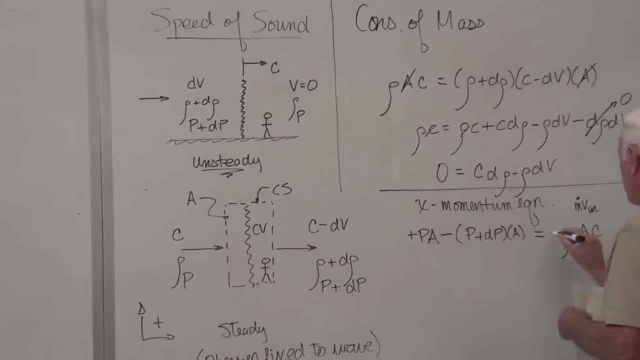 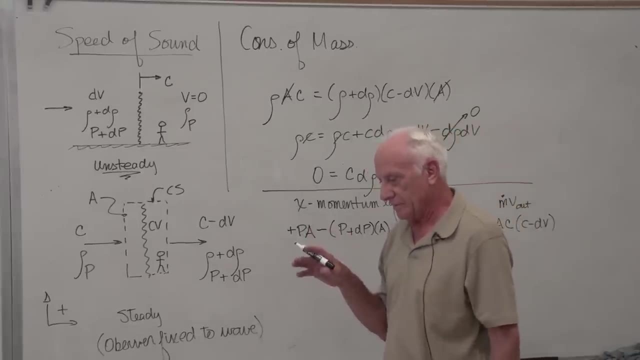 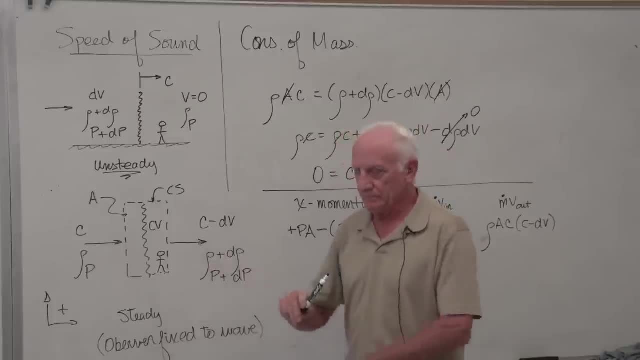 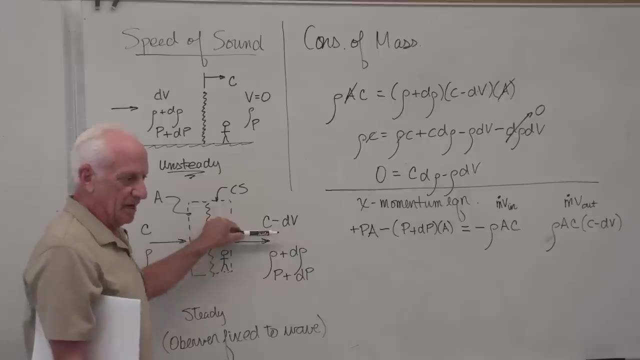 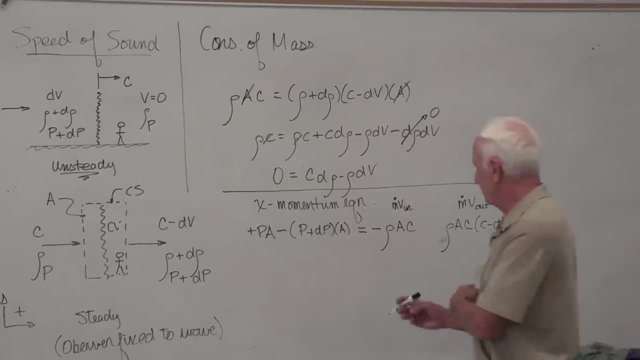 Which way is the velocity vector Plus sign? Which way is the area vector That way? Take the dot product. What's the angle between them? Zero sine cosine, zero plus one plus sign. Plus sign. Zero sine cosine, zero plus one plus sign. 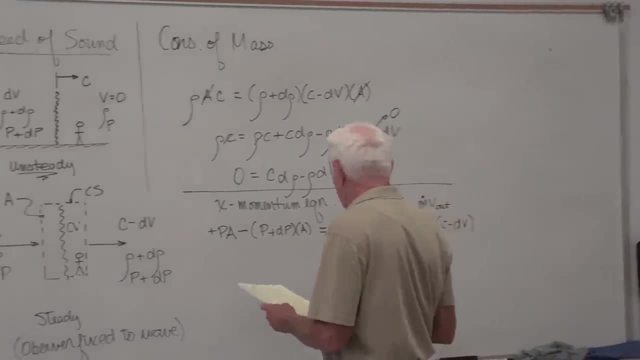 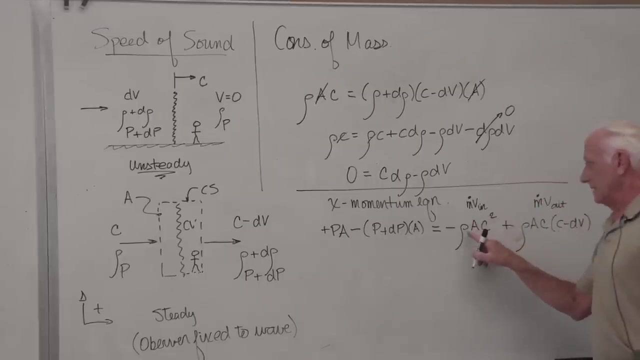 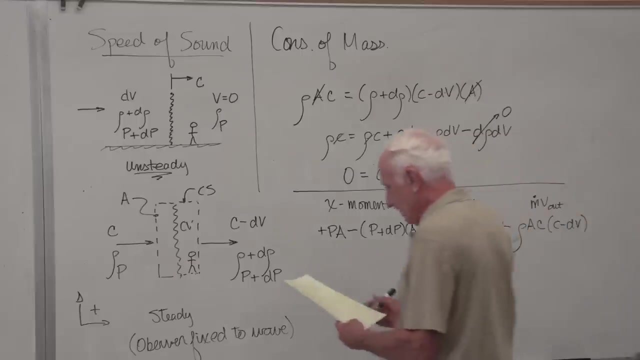 Okay, there it is. Obviously, some things are going to cancel out this guy. If I do it right, I'll get it right. M dot's row AC times the velocity of C. so it's squared. Okay, so we reduce this down. 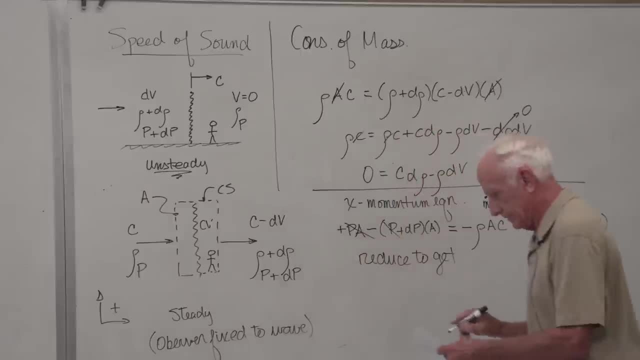 Here's a PA. there's a PA. Here's a PA, there's a PA. Here's a PA, there's a PA. They go out there. okay, They go out there. okay, They go out there okay. 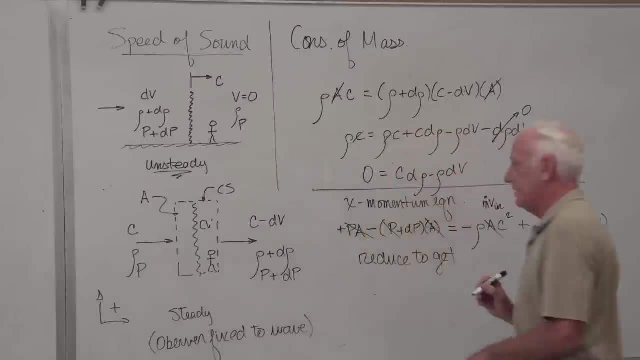 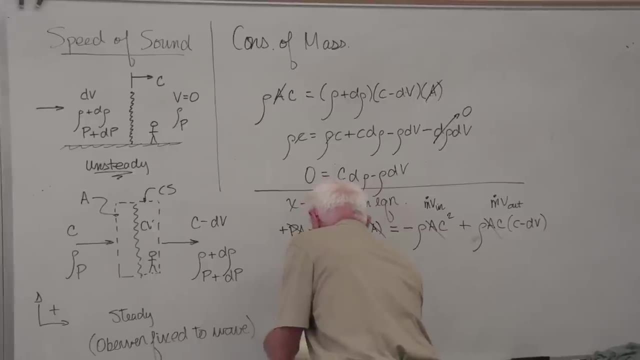 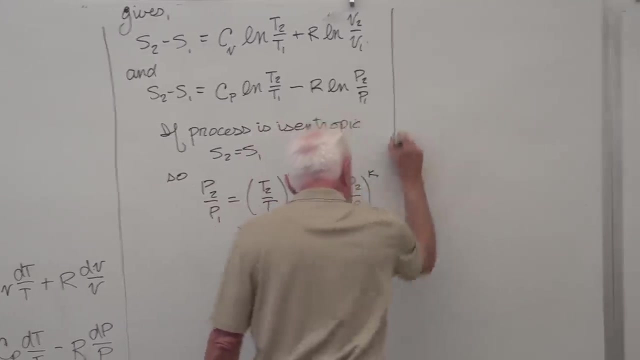 There's an area vector there. Area, area, area area cancels out all three terms. This simplifies. okay, About two lines. Simplify to get dP equal row C, dV. I'll do it right here, Okay. 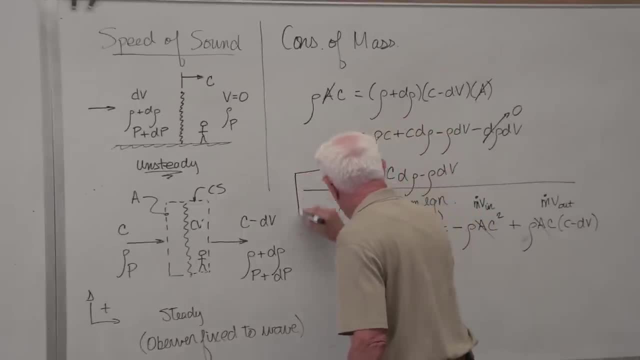 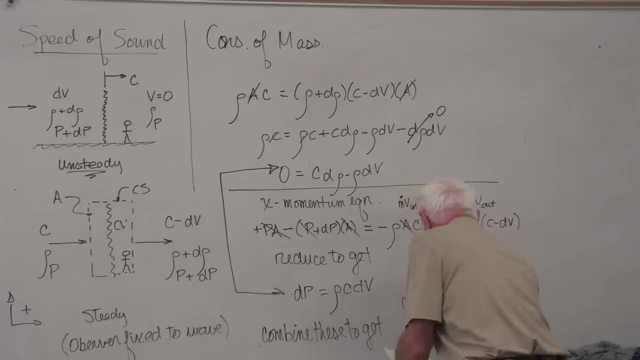 Combine these two get. this is what I get then, when I combine these guys: dP equals C squared dRho. dP equals C squared dRho, Or C is equal to the square root of d, dP- dRho. 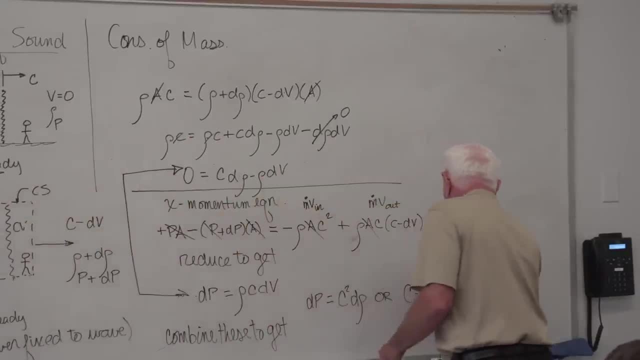 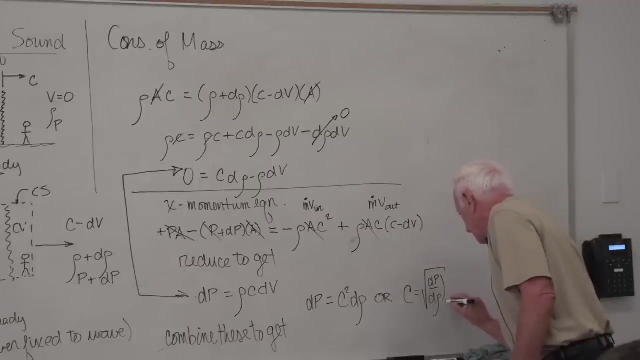 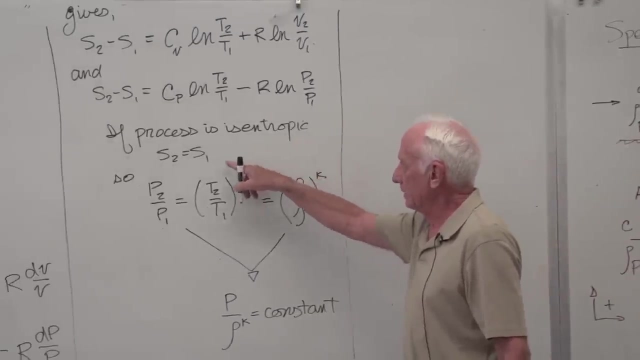 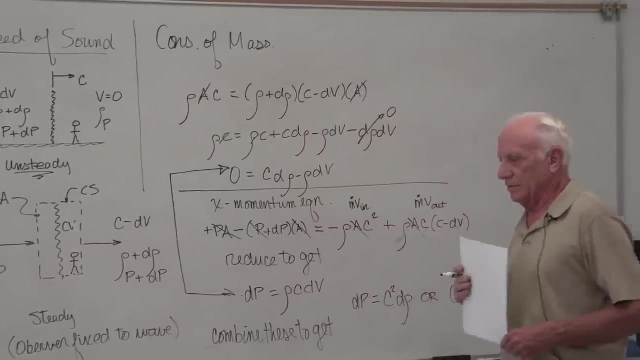 Okay, You put on here subscript. S mean entropy is constant. okay, Isentropic, isentropic. What's isentropic mean again from thermo Adiabatic, reversible. Is it adiabatic? Is there a lot of heat generated? 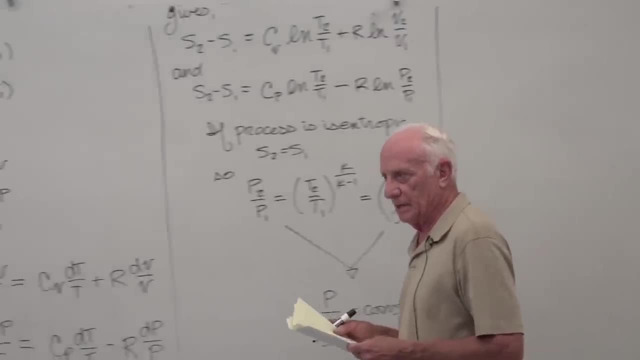 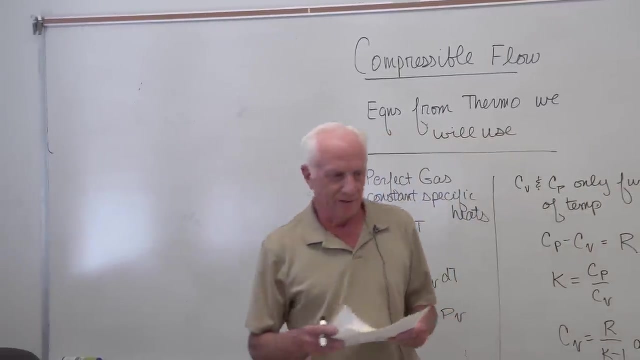 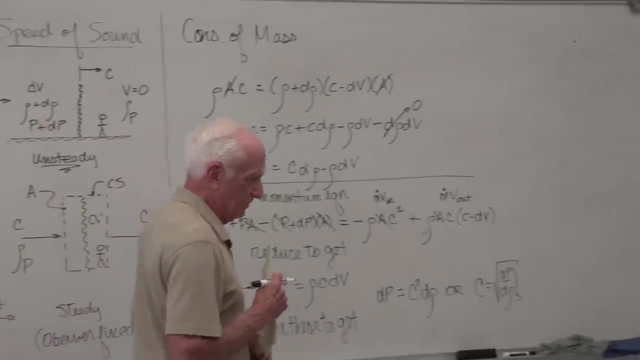 I don't think so. I don't think my voice is generating a lot of heat in the air. No, Is it reversible? No, Is it reversible? Yeah, kind of it's reversible. It's such a gentle wave Differential changes in properties that we treat it as if it were reversible. 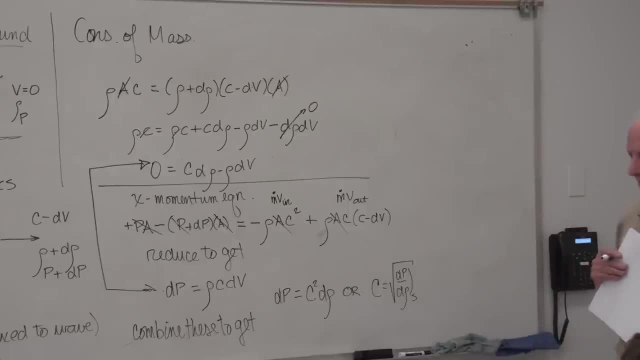 Is the shock wave reversible? Oh my gosh. no, It generates tons of heat, Tons of heat and lots of friction, so it's not reversible. No, no, shock wave is. it's a shocking thing, you know. 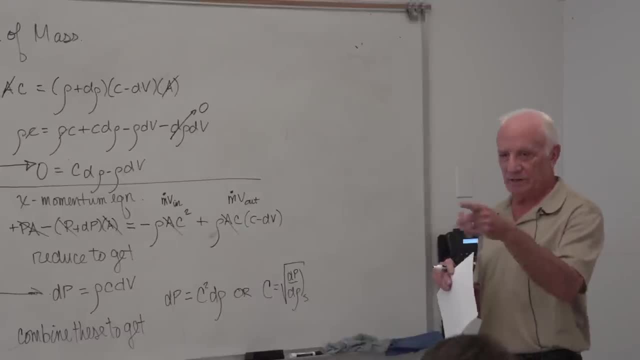 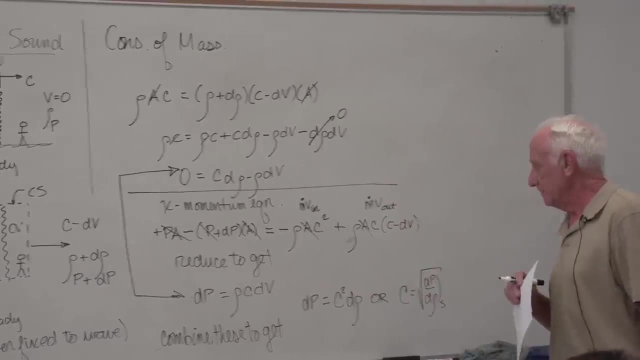 It's not isentropic. My voice in your eardrum is pretty much isentropic. I could scream it still wouldn't matter. I can't reach Mako in my voice, so okay, So okay. we put the S on there. 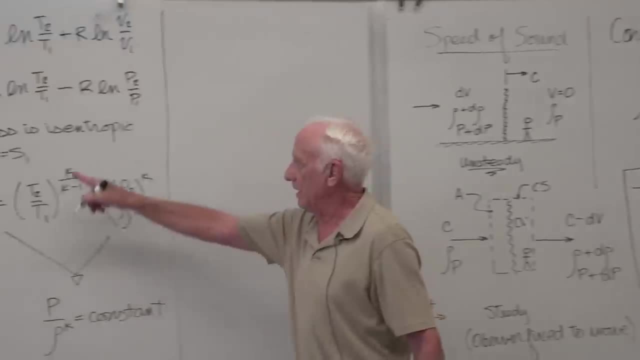 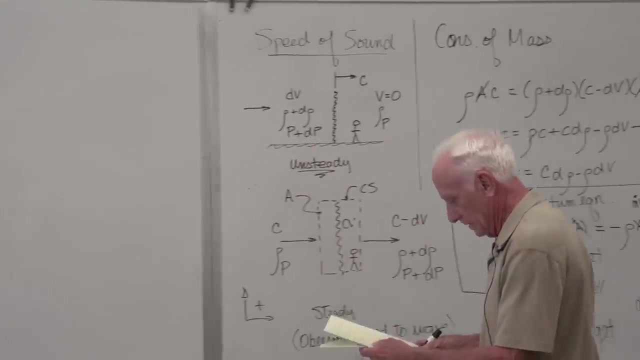 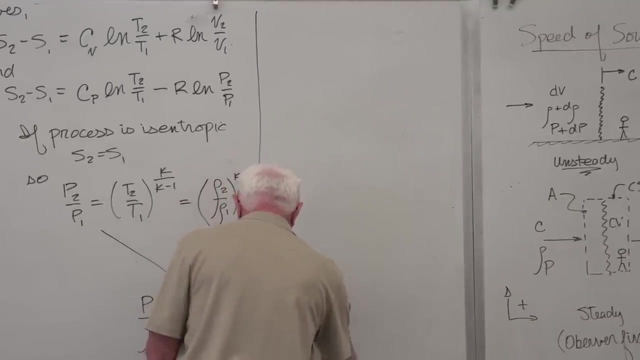 Why? Because we're going to use this guy down here. If the process is isentropic, that's true. If it's true, we can do this guy right here. okay. So we can take this guy right here and we can say dp, d rho. 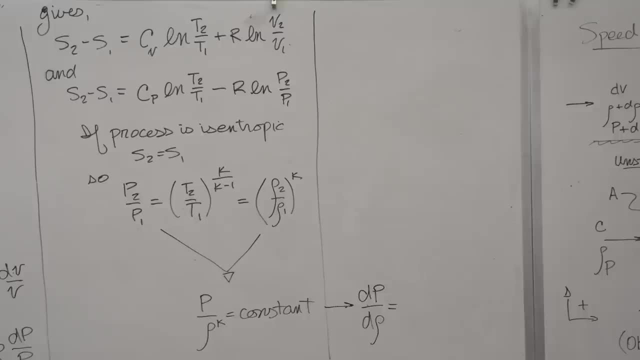 because that's what I need. dp d? rho. This is p? rho to the minus k? okay. So okay, you differentiate that guy. you can do that. You get k? p over rho. perfect, gas k? R T. There's two lines missing there. 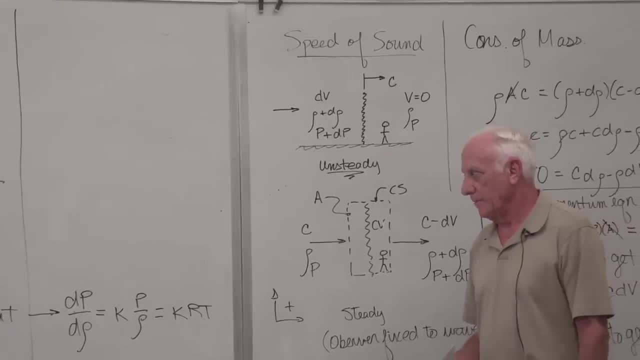 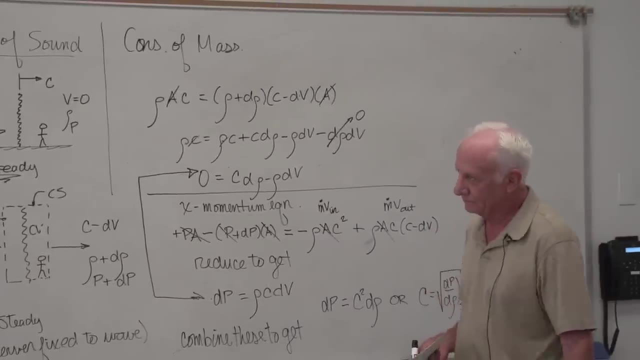 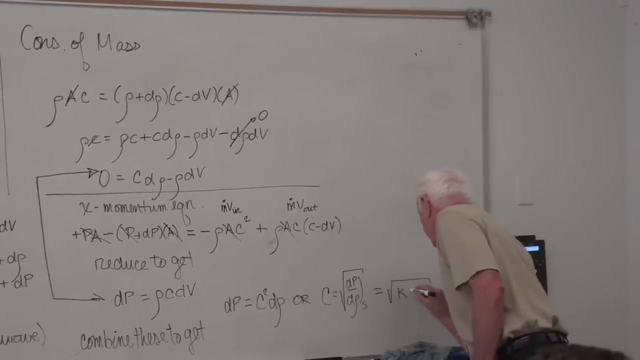 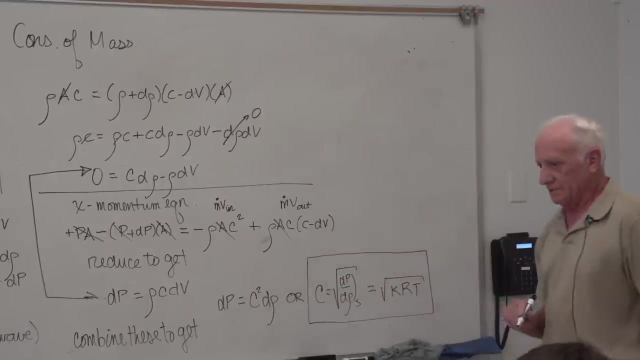 You can differentiate that guy though. Minus k p to the rho, to the minus k minus 1, that's it. Put that result into here. Okay, That's the speed of sound we're going to use. The speed of sound can be calculated as the square root of k times R. 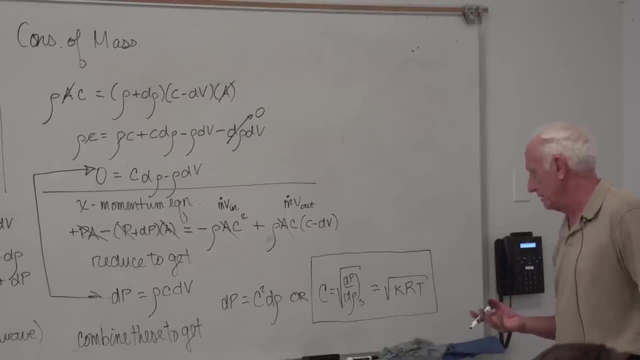 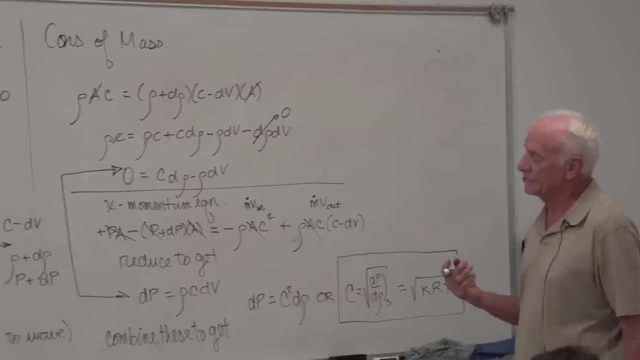 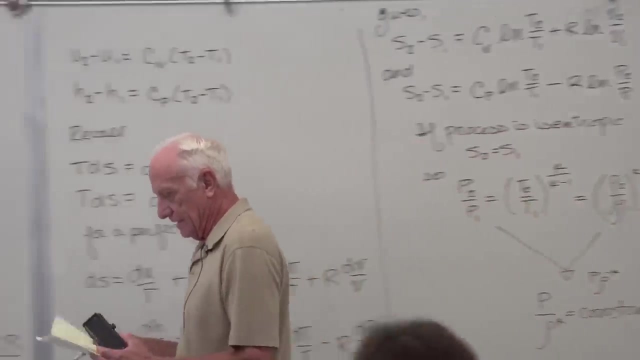 and those depending on the gas. Is it air? is it nitrogen? carbon dioxide times the absolute temperature of the gas. It's a perfect gas. Okay. the process is soon to be isentropic because it's a. it's a very weak pressure wave, Okay. so now we have an equation for the. 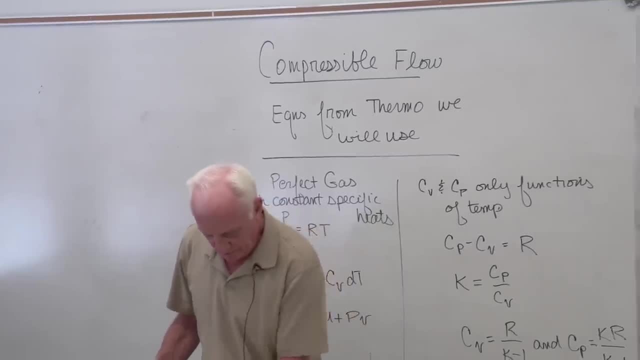 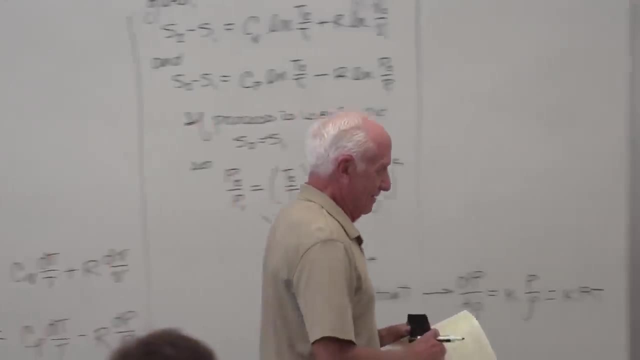 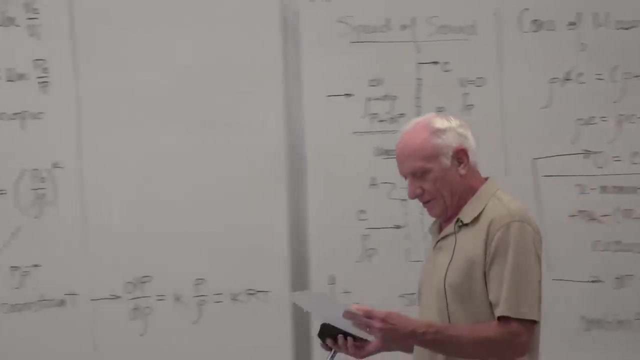 Speed of sound. and what is it a function of? well, it's a function of absolute temperature. What does that mean? The hotter the temperature, the faster the speed of sound. The colder the temperature, the slower the speed of sound. Okay, so let's then. 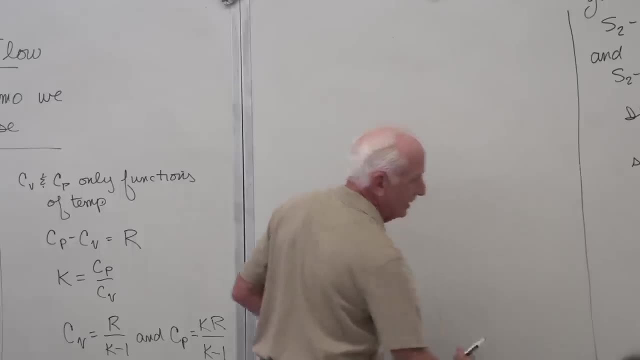 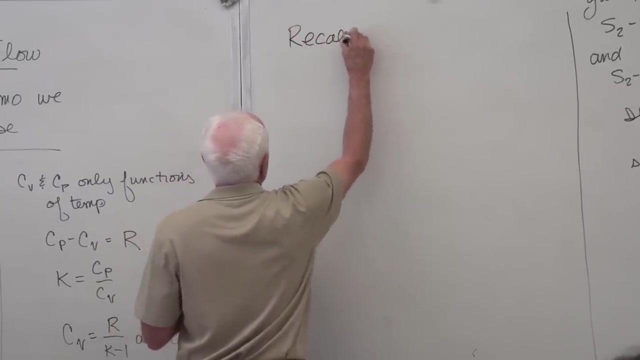 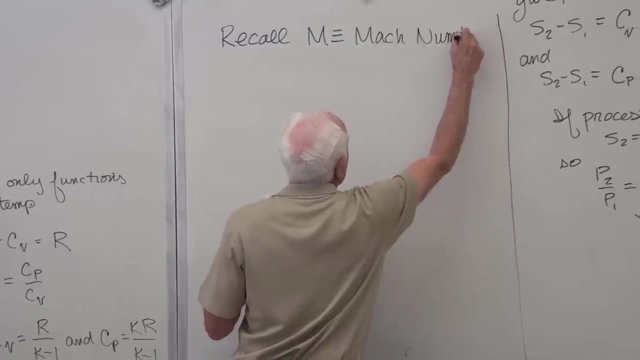 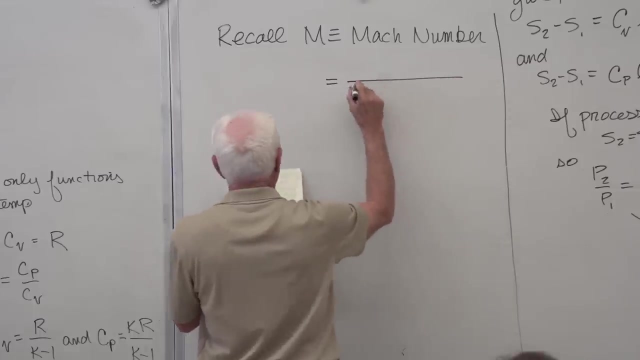 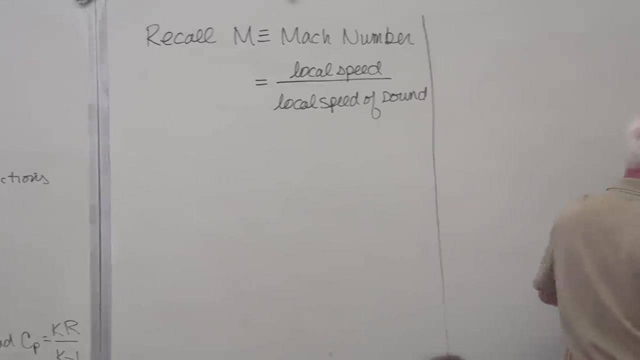 Define. go back, and we talked about the Mach number in the dimensional analysis chapter. so Recall the Mach number, And that was defined as the local speed Divided by the local speed of sound. So Let's do it a simple little problem. So here's the ground, and 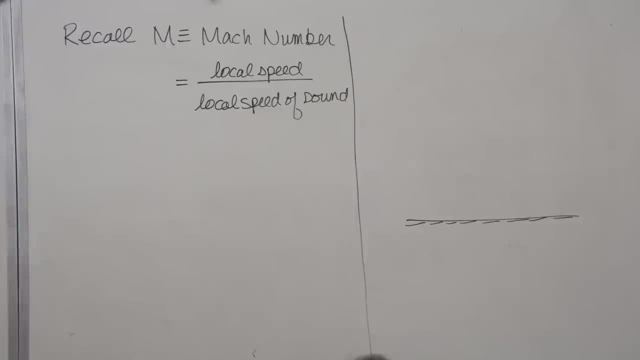 Let's assume that there's some aircraft that's flying. Let's see where you are. Let's see where you are. Let's see where they. okay, here it is sea level, So let me take sea level here and show this picture here: The velocity of that aircraft at sea level. 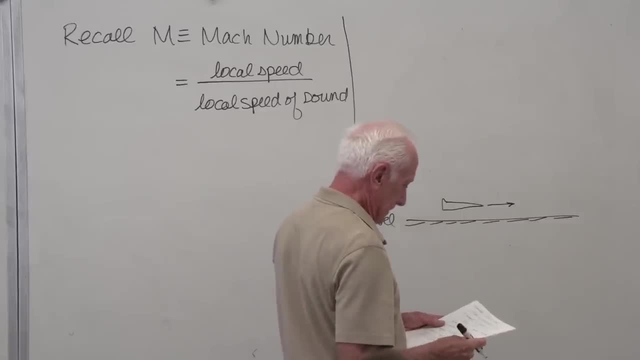 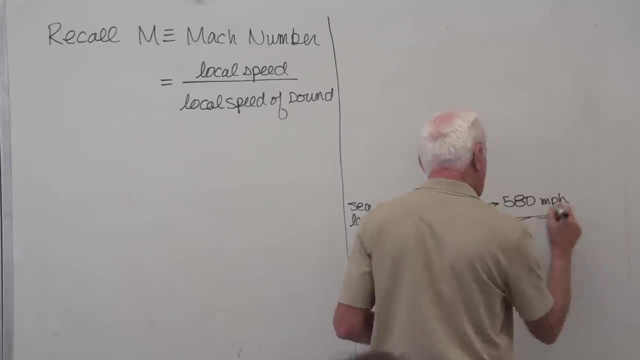 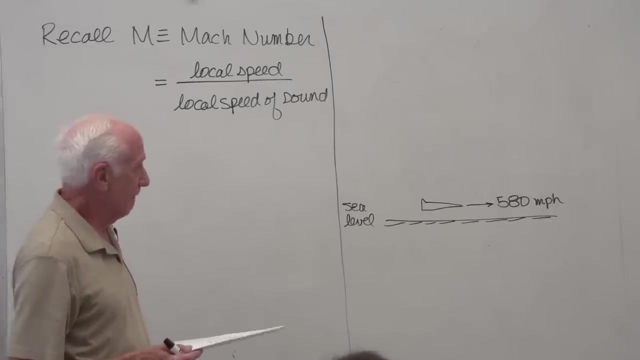 I'm gonna make something up. 580 miles per hour F-18 flying over the ocean, Don't sea level. I Want to find this Mach number: V over C. C is the local speed of sound, V is the velocity of the aircraft. I Can't use miles per hour. I'm going to convert to feet per second. 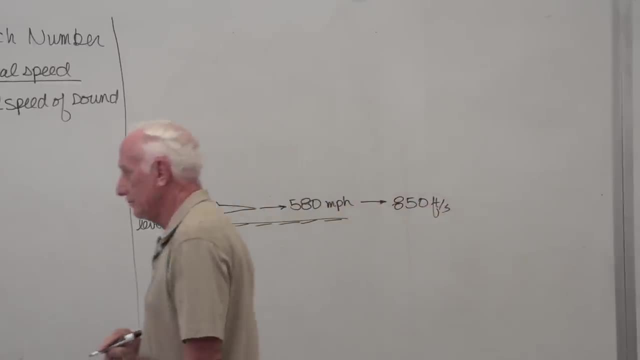 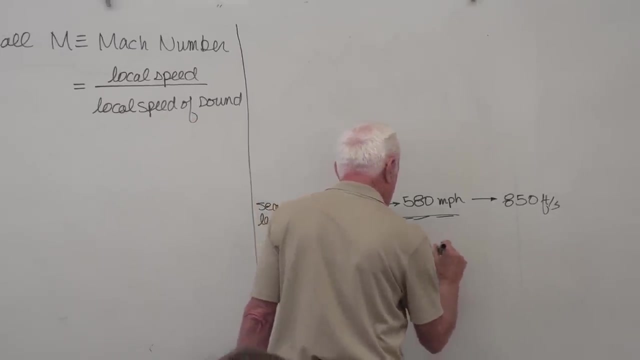 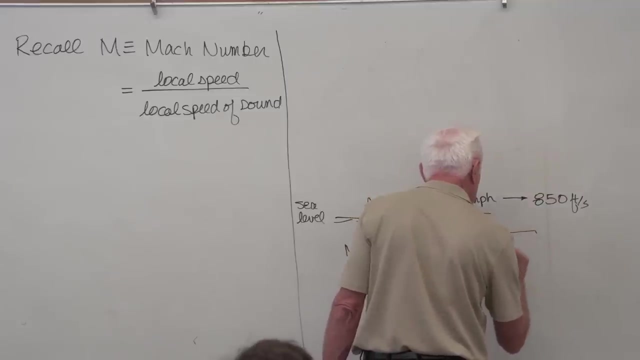 850 feet per second. okay, First thing I'm going to find see Two ways to find it. number one is: you can go ahead and take the square root of K RT load B, Pay is K is 1.4 For air, R is 17- 16. 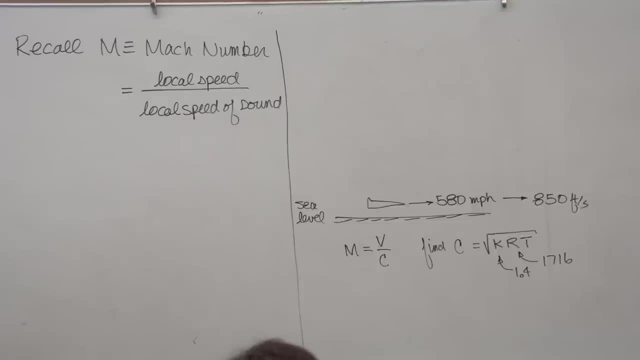 Okay, they came from properties of air in the back of the book. Let's go to properties of air. Oh Okay, yep, that's right, That's good know if they gave us that. oh yeah, wait here did I think maybe, maybe they did. 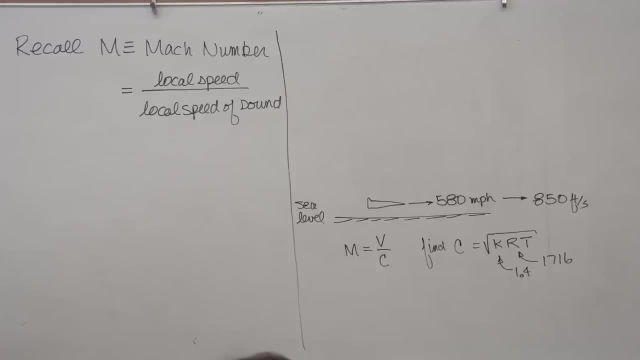 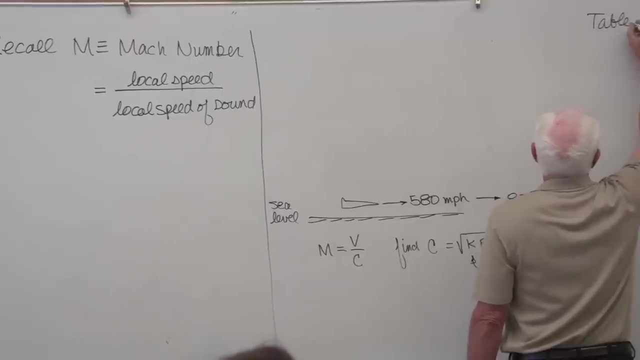 nope, they didn't give us the value in English units, SI, so that's what they are in English units. we have to find a temperature, okay. so we go to the back of the book and we say, mmm, table a6- properties of the standard atmosphere. table a6- properties of standard. 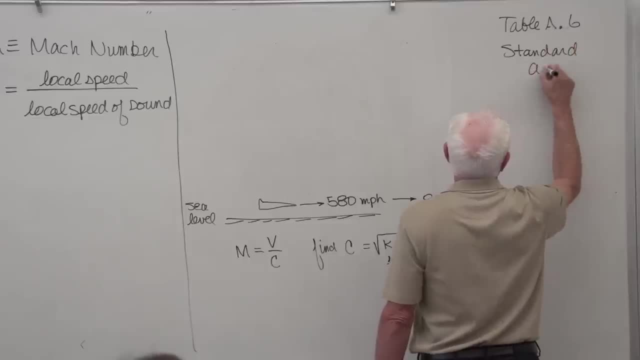 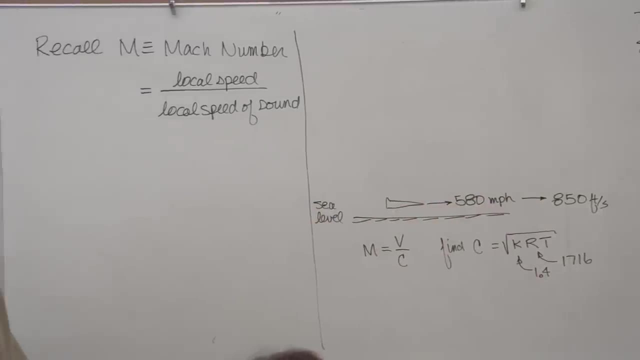 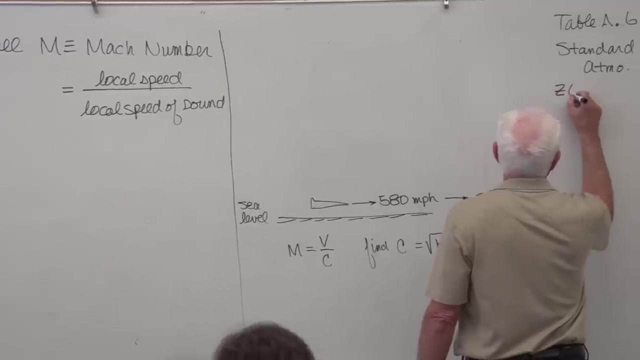 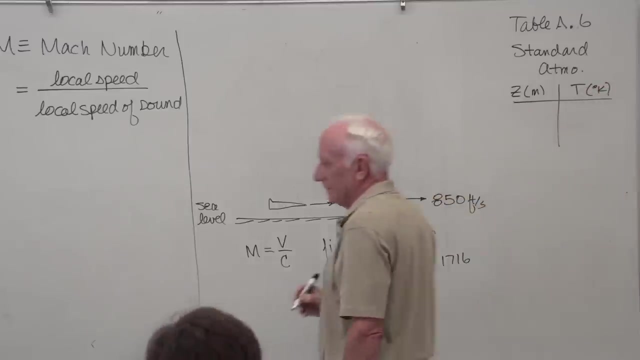 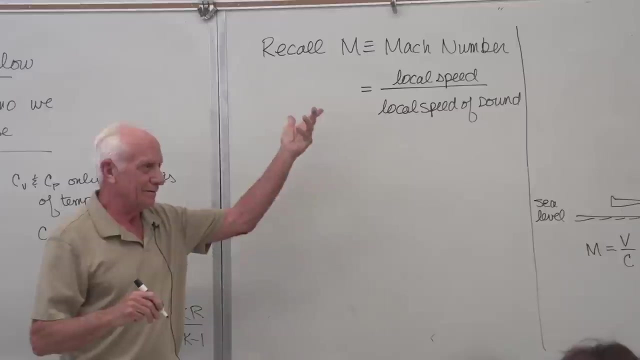 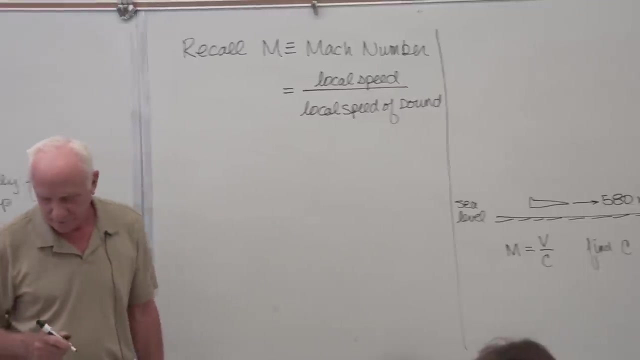 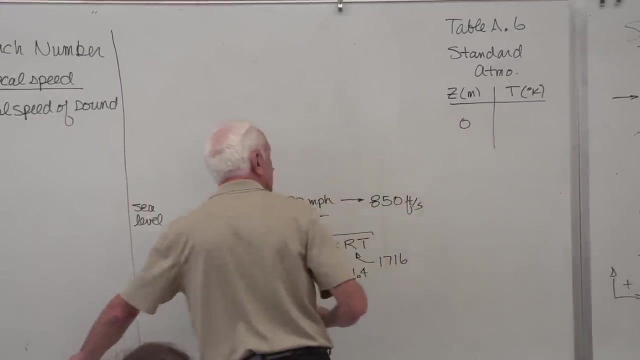 atmosphere: okay, T, Z is the elevation and then temperature in Kelvin, Z in meters and temperature in Kelvin. so that's the only table you've got. you've got to convert two feet two meters and Fahrenheit to rank into Kelvin, whatever, no big deal. sea level: okay, he's got it. he's got it. he's got a zero there, okay, I. 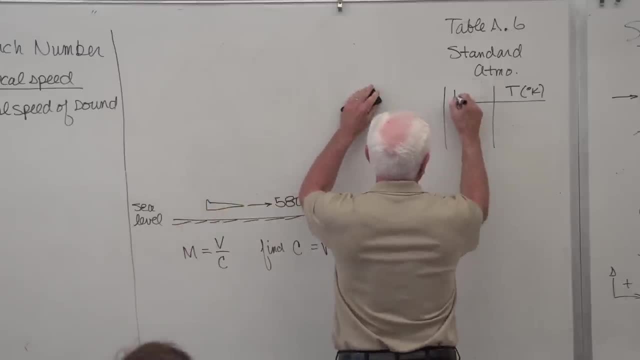 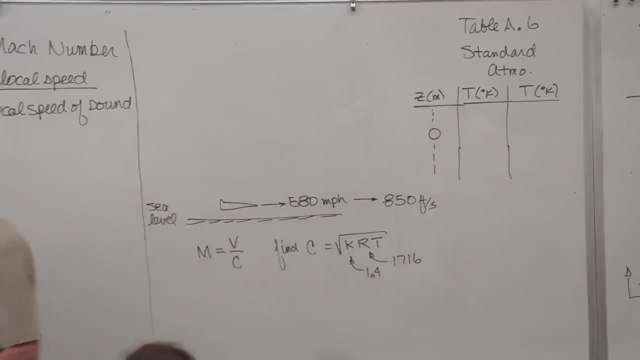 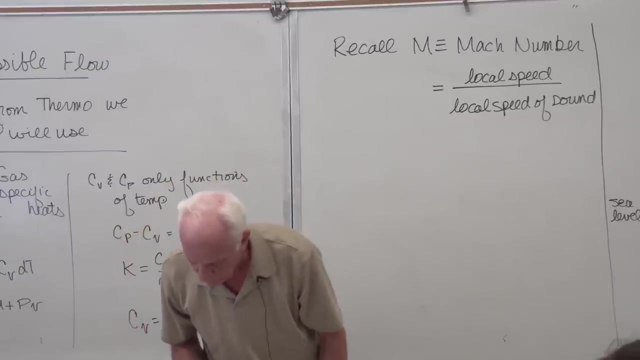 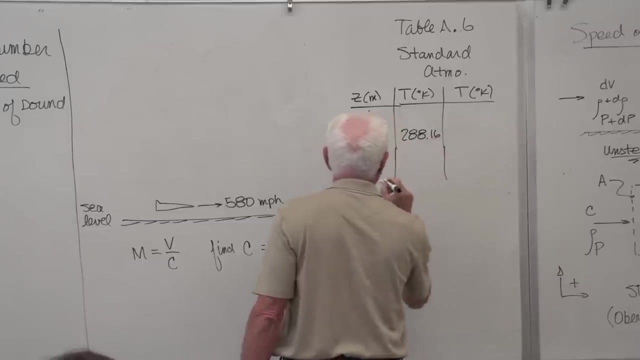 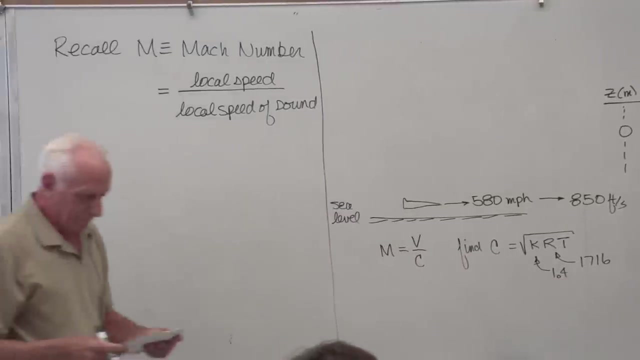 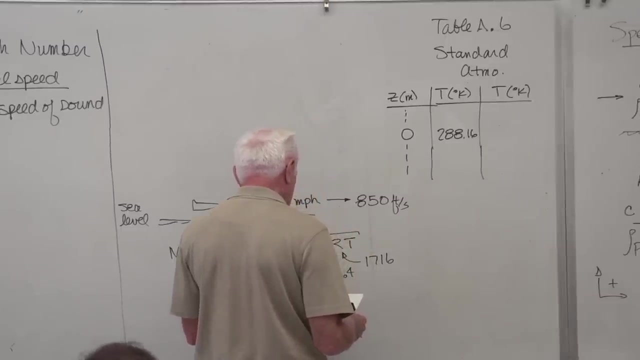 have to shift these things over. okay, there's their own. 288.16, 288.16. okay, so convert that guy. I did the temperature there, the dot. let's see there it is 59 degrees Fahrenheit. 519 degrees are 460 plus 59. convert to absolute. I'll. 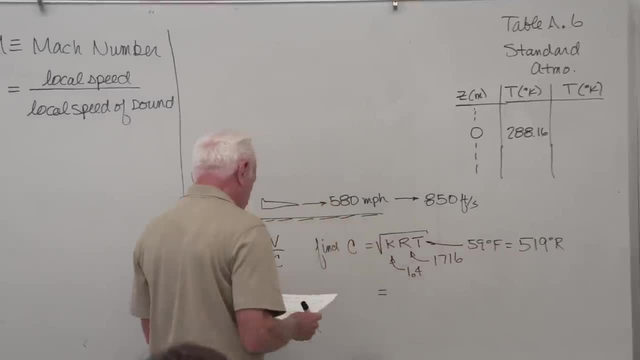 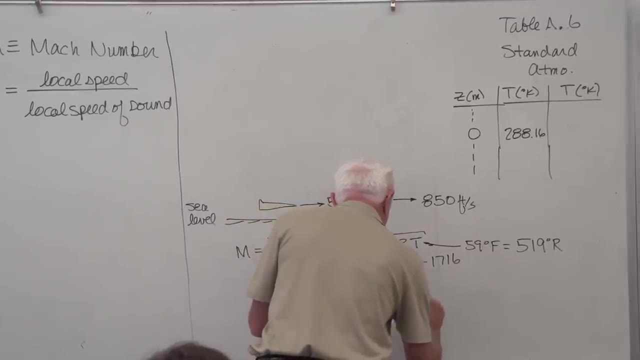 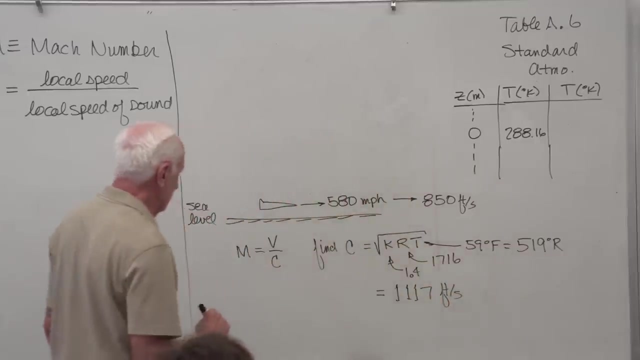 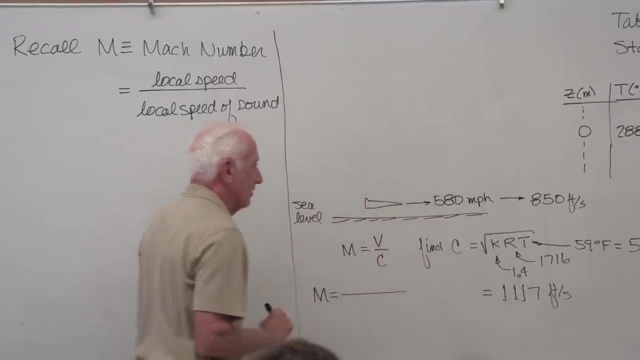 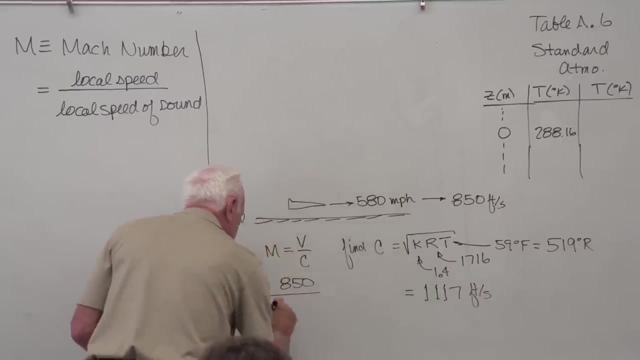 Put those guys in there. K our absolute temperature And the speed of sound at sea level for the standard atmosphere is 1117 feet per second, Got it? The Mach number is equal to the speed of the aircraft- 850. Divided by the local speed of sound, So our Mach number at sea. 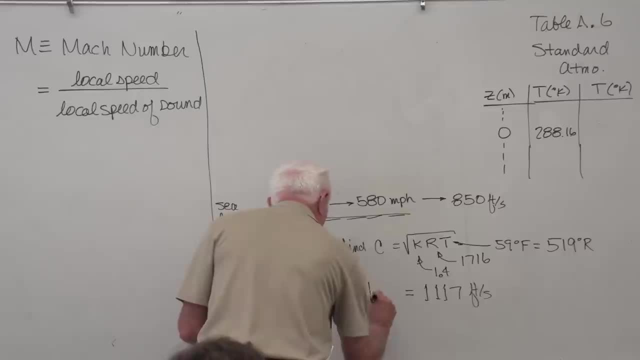 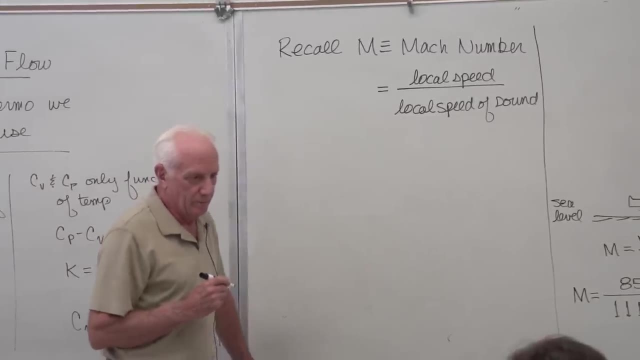 level is 0.519.. Is that a compressible flow problem? Oh yeah, If the Mach number is greater than .3, we've got to include compressibility effects. .519.. Is that a compressible flow problem? Oh yeah, If the Mach number is greater than .3,, we've got to include compressibility effects. 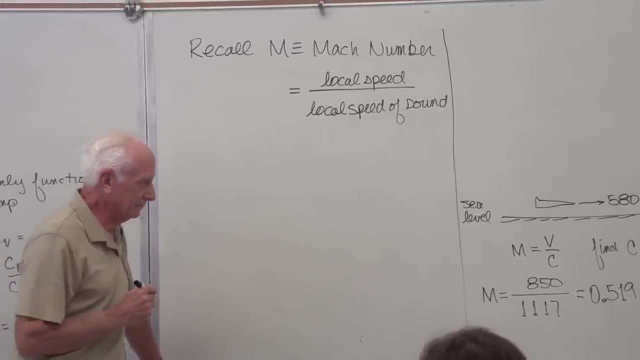 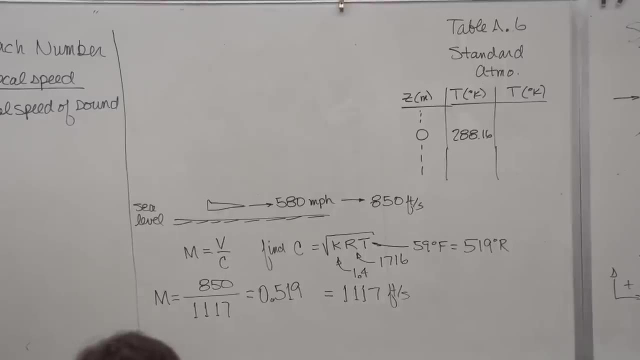 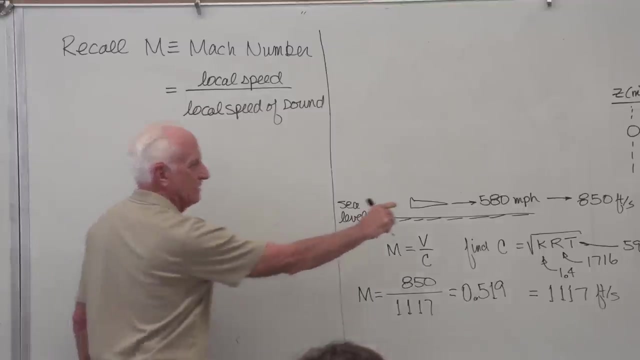 .519.. Is that a compressible flow problem? Oh yeah, If the Mach number is greater than .3, we've got to include compressibility effects. Yep, it is. What does the word local speed mean? It means the speed at the location where the aircraft is Okay, 580 miles per hour. 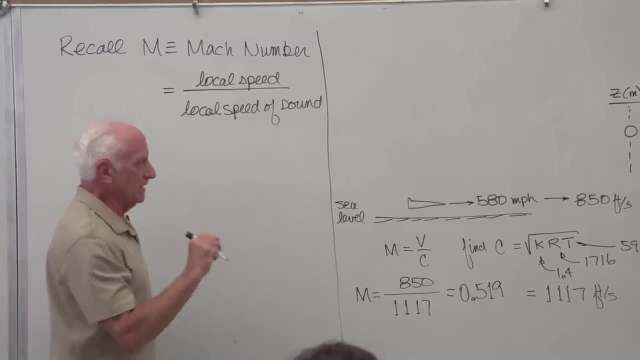 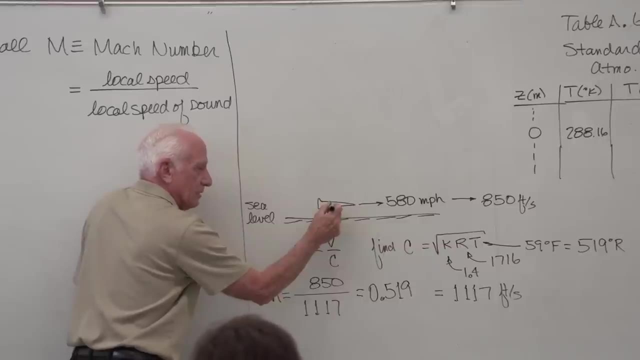 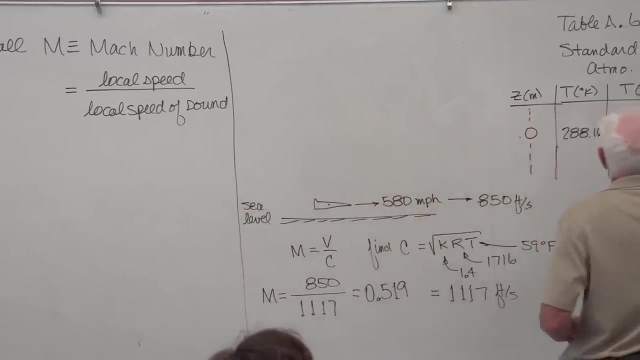 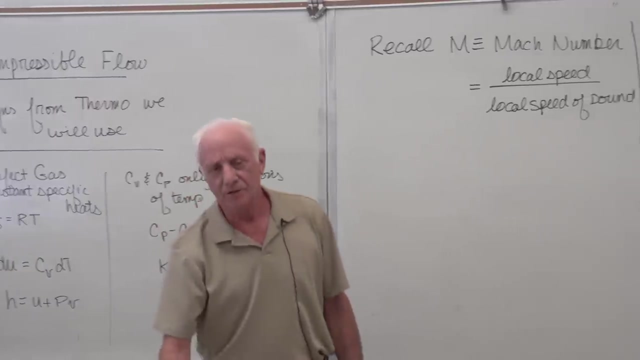 What does local speed of sound mean? That's the speed of sound at the location of the aircraft right there. What's the elevation level? Zero. Where do I go over here? Zero, Now, if you'd rather, there's another column in there called. he calls it A, I call it C. 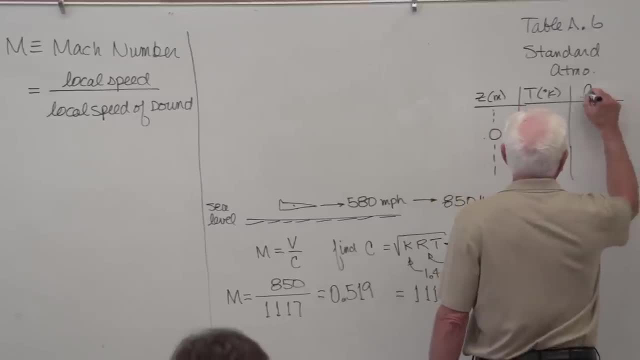 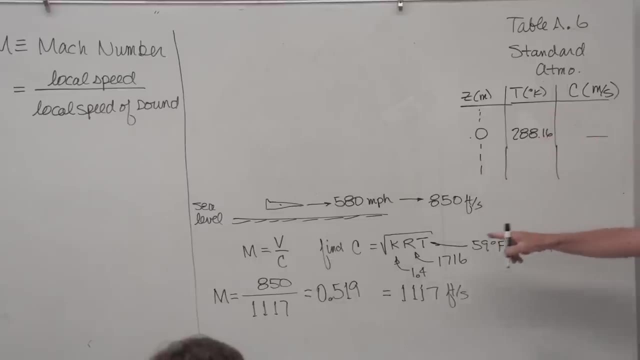 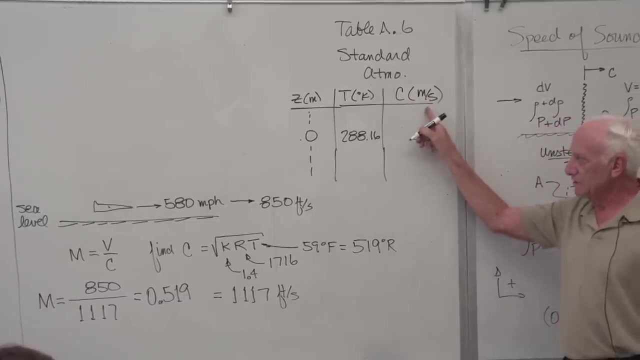 don't forget. Oh yeah, he gives it right in there. You don't need to go through here, because he tells you the speed of sound is the speed of sound at sea level is this number. Convert that number, meters per second, to feet per second and you would end up with 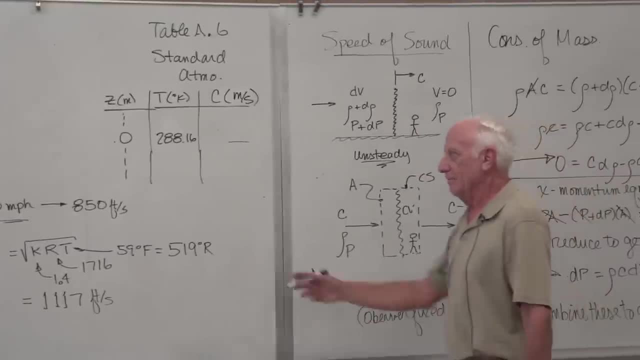 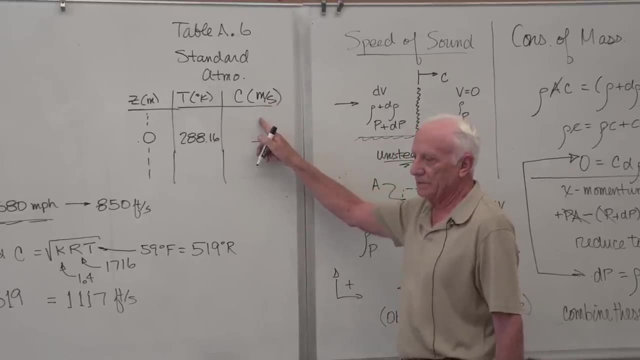 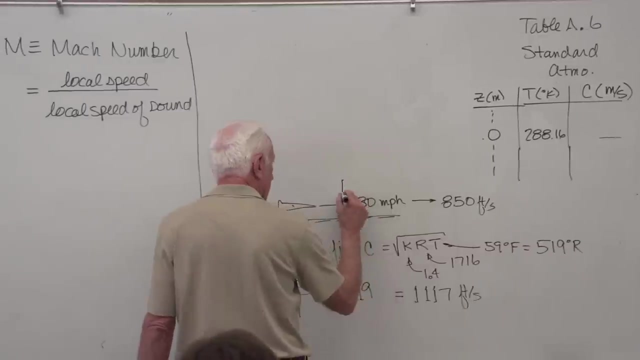 1117.. Okay, so two choices: Put it in the equation yourself and find it, or go to that table A6 and it's in the last column on the right-hand side. Speed of sound, depending on the altitude you're at above sea level. So his Mach number is about 0.52.. 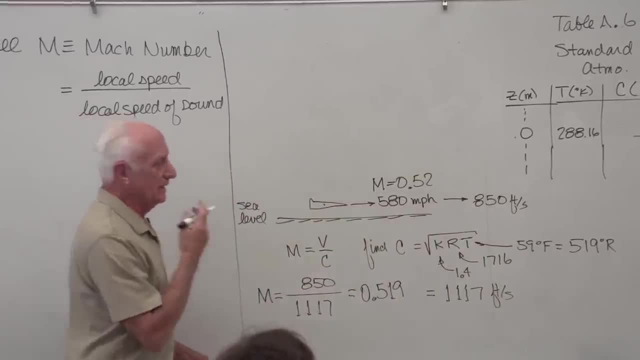 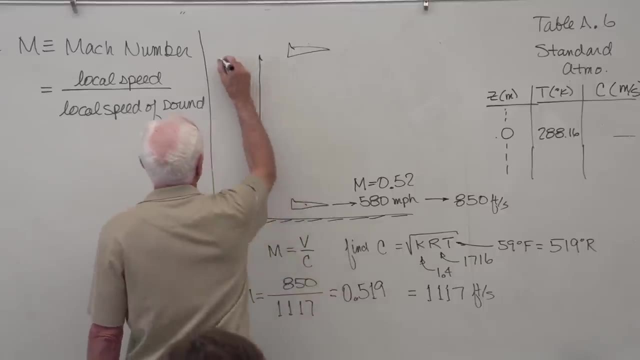 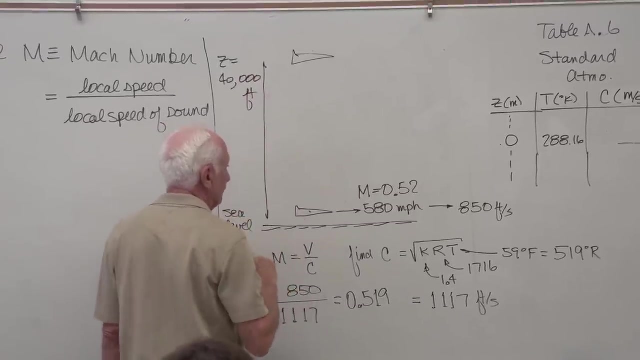 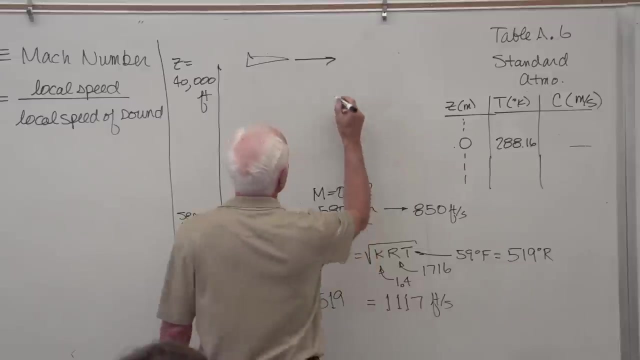 Now you take that same jet fighter and you go up to 40,000 feet. Okay, I fly at the same speed. It's a calm day. This is the ground. It's called the ground speed: 580 miles per hour. 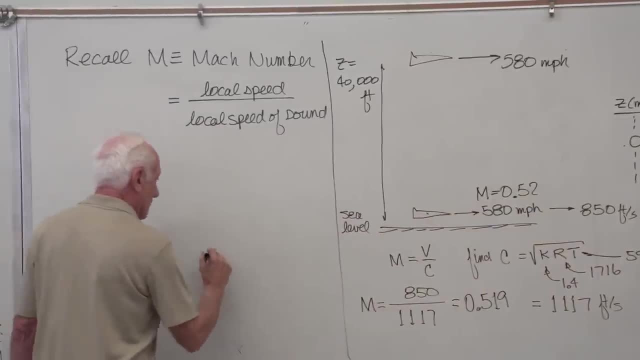 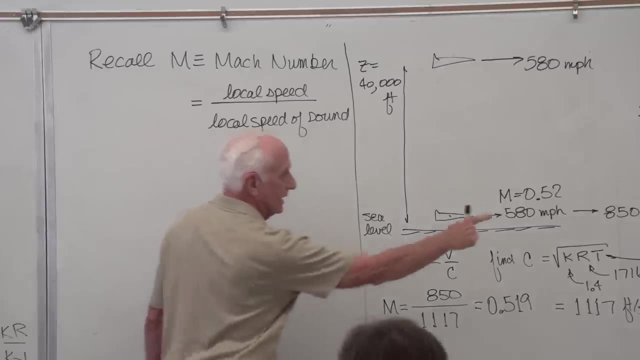 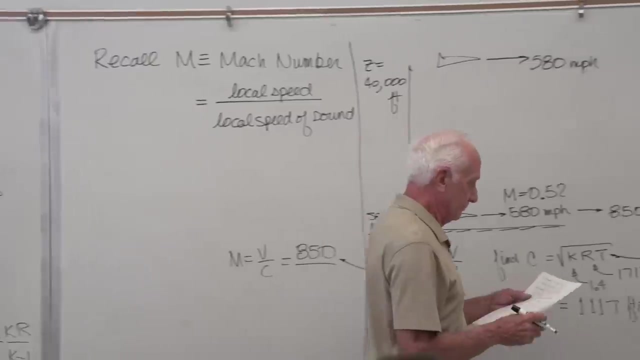 Okay, Mach number is equal to V over C. Mach number is equal to the velocity. It's the same 850 divided by okay, now it's got to be the speed of sound at 40,000 feet, Just so you know. at 40,000 feet. Okay, Okay, With the standard atmosphere. the temperature up there is a mighty cold: 67.6 degrees Fahrenheit, Absolute, 392 degrees Rankin. Of course it is, You know, at the outside of aircraft flying at 30,000 feet. you know it's cold out there. Yeah, you go up to 40,000 feet, it's. 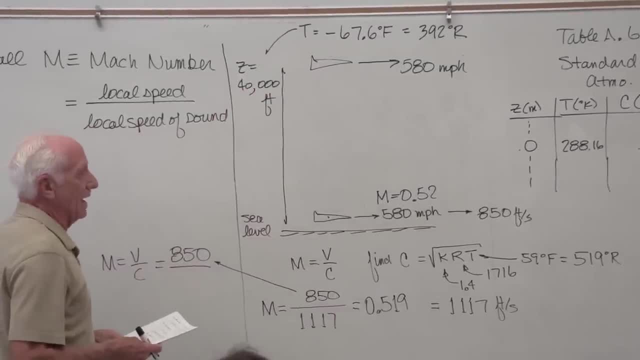 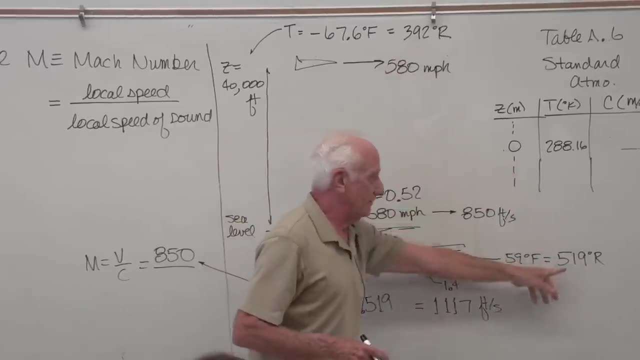 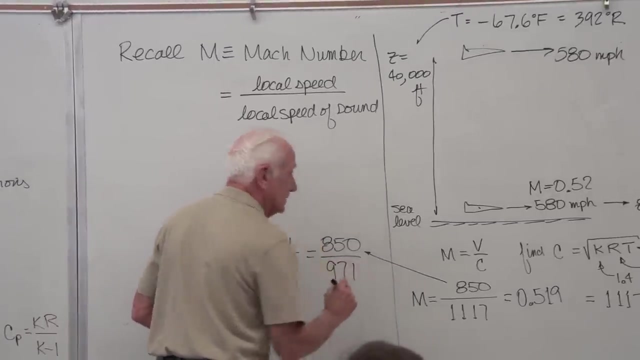 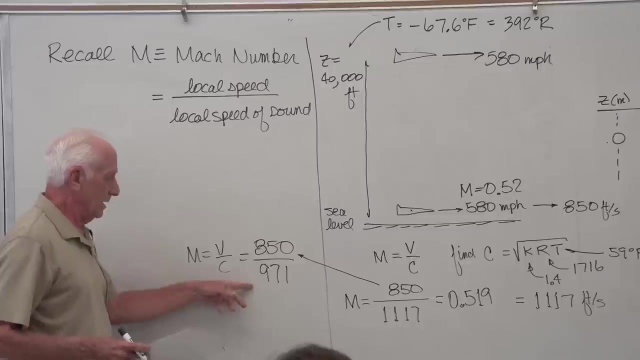 really cold out there the air. What happens? Oh, here you go, You plug it in there. Now you've got 392 compared to 519 sea level. So now your denominator here. what does that mean? If it's colder, lower temperature, speed of sound goes down. speed of sound went down. Aircraft velocity still the same: 580 miles per hour. 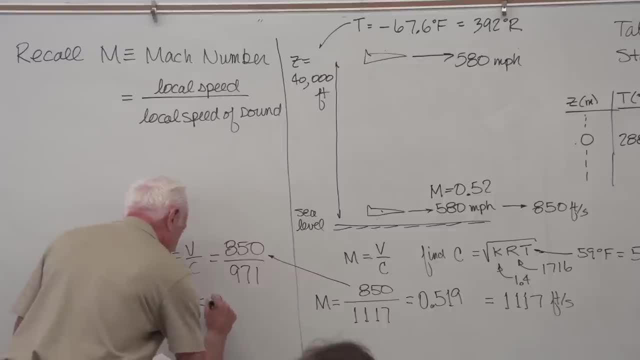 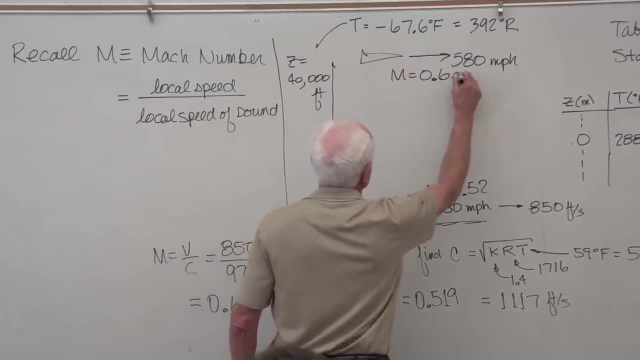 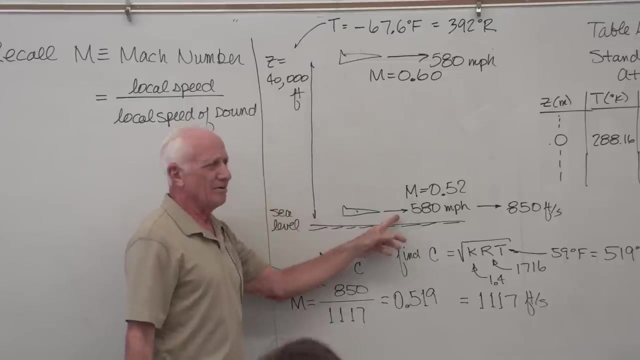 The Mach number at 40,000 feet 0.60.. This guy says: hey, Joe, down there at sea level, guess what? my Mach number is 0.6.. Joe says: oh no, mine's only 0.52.. You're going faster than I am. 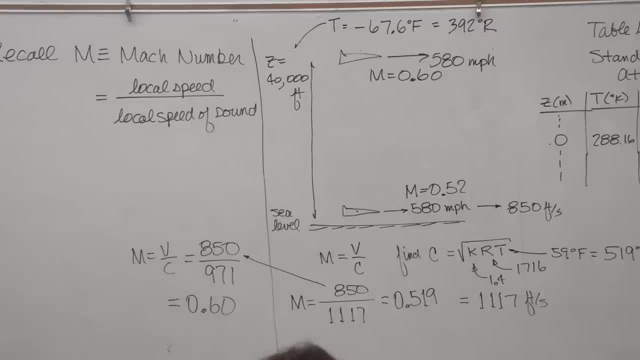 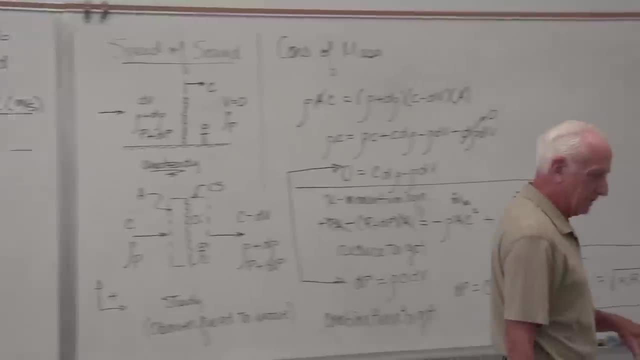 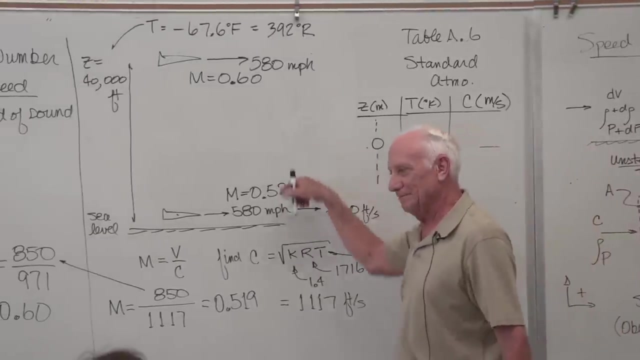 No, you're not. They're both going the same speed. The Mach meter isn't giving you a correct indication. The Mach meter is giving you the Mach number, But your actual ground speed is the same for both aircraft. So it changes. The velocity is the same, but the Mach number is different because the temperature of the air is different at those locations. 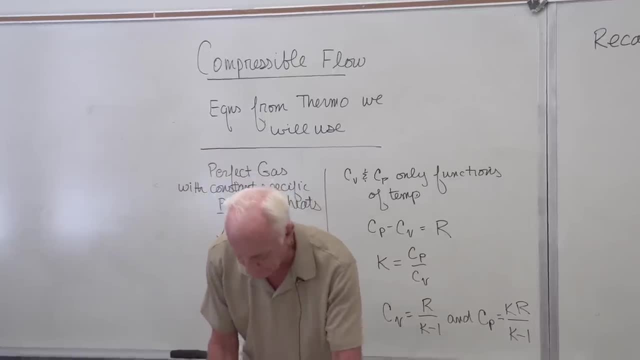 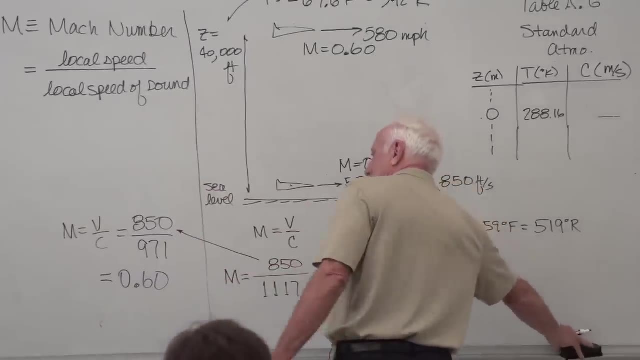 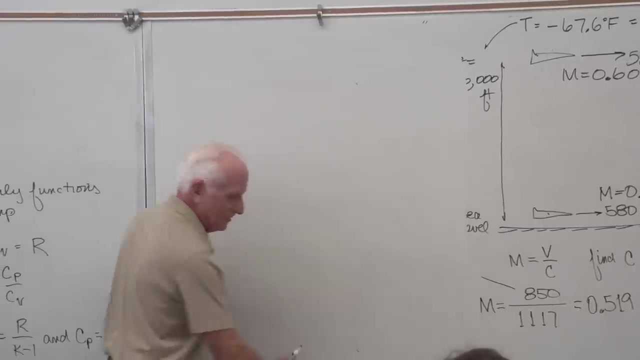 Now let's go ahead and take another. That is what we need now to get the speed of sound and Mach number. So let's take a look at one more thing before we go into our review. Maybe we're in party mode right now. 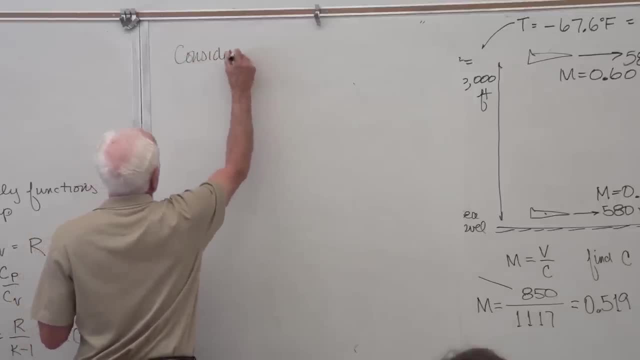 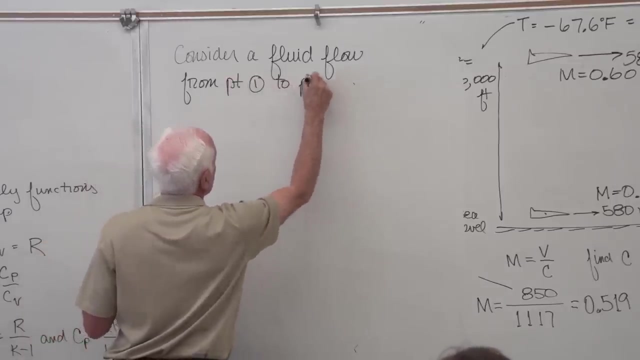 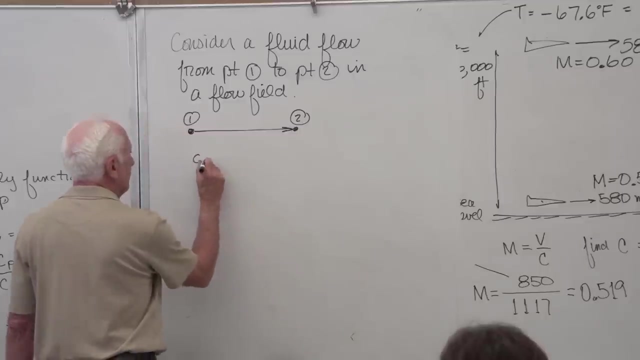 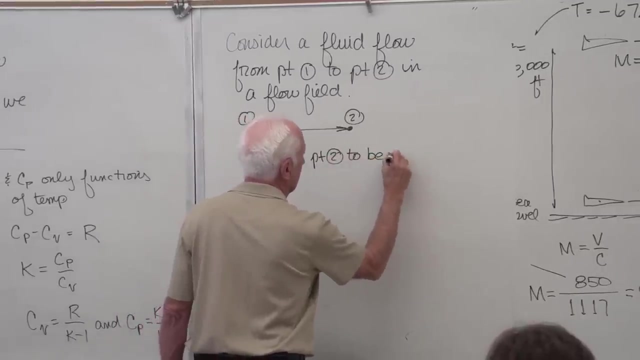 Ok, Give me a moment, We're in good shape. Consider a flow From 0.1 to 0.2 in a flow field. Okay, Here's point two. All right, we're gonna consider point two To be a stagnation point. 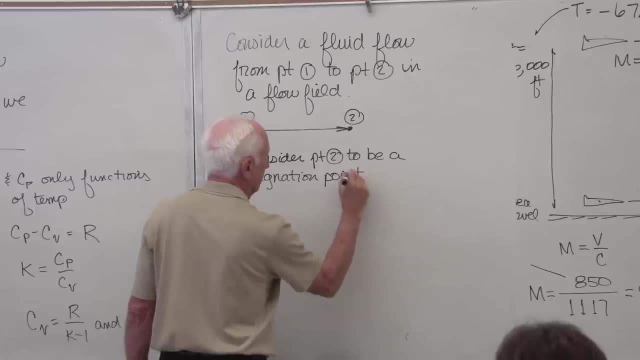 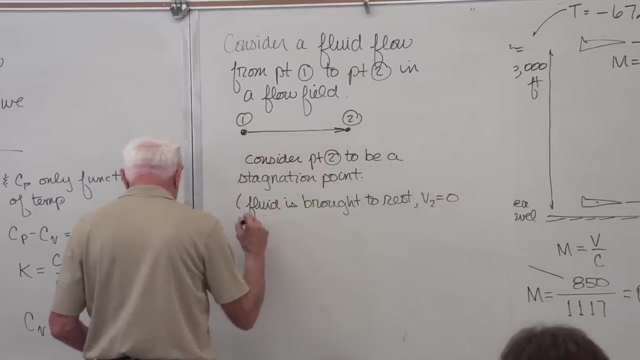 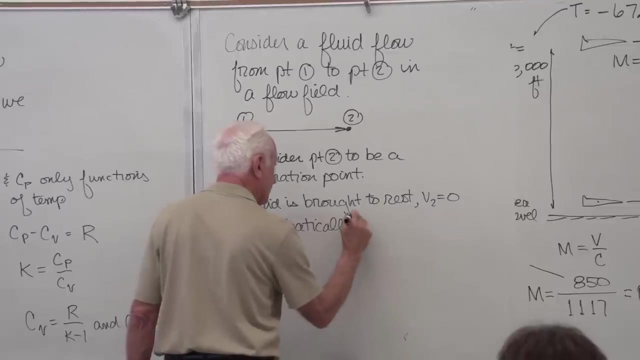 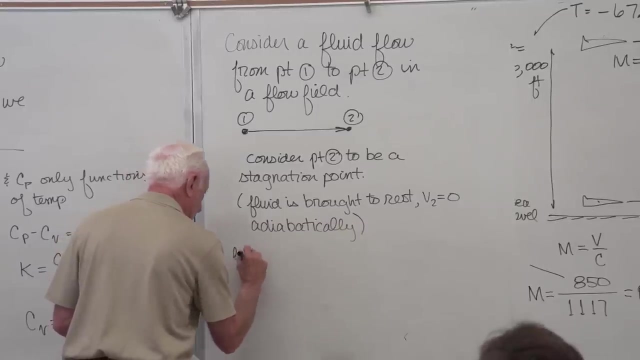 This Was covered in flu is one. a Stagnation point is a point where the velocity comes to rest at zero. so Fluid is brought to rest. V, 2 equals 0 Is brought to rest. adiabatically, No heat transfer. The equation we get, It's equation 923 in the textbook. 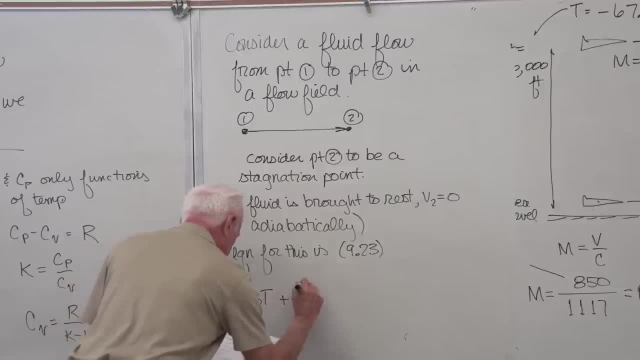 C sub PT plus V squared over 2- and That's the temperature at 1, but just call it general- is equal to C sub P Times T naught Plus. I guess we should Stagnation point the velocity. in my picture here T and V are at any point in the flow field. 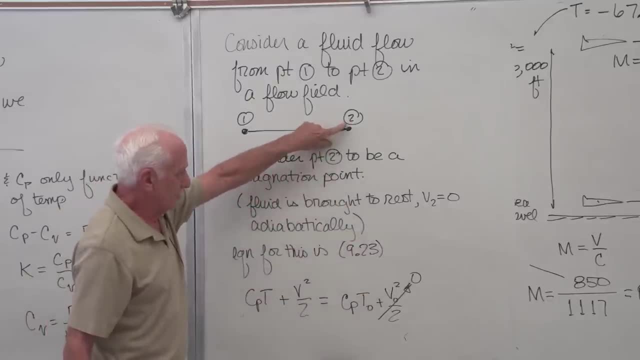 T naught and V naught are at the stagnation point At point two. so point two corresponds to the subscript zero stagnation point. This guy's general corresponds to point one. Where'd this come from? This is energy. I'll just give you a real quick. 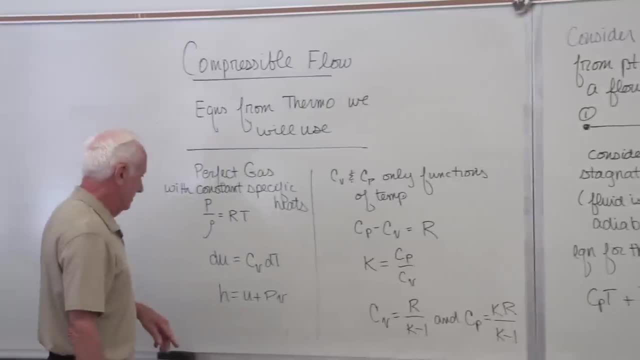 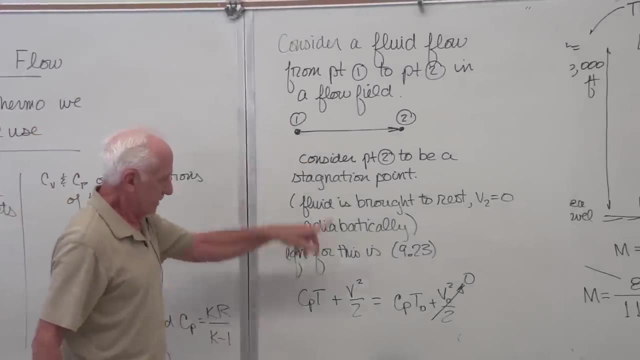 C sub PT. I probably erased it, Maybe I didn't. C sub PT is a change in in enthalpy. This is the enthalpy at that point. This is the enthalpy at that point. Okay, this is a kinetic energy. 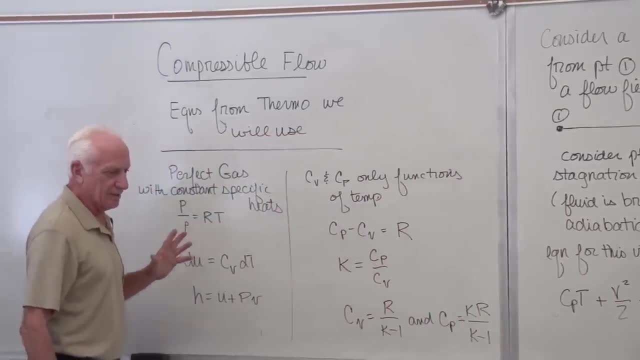 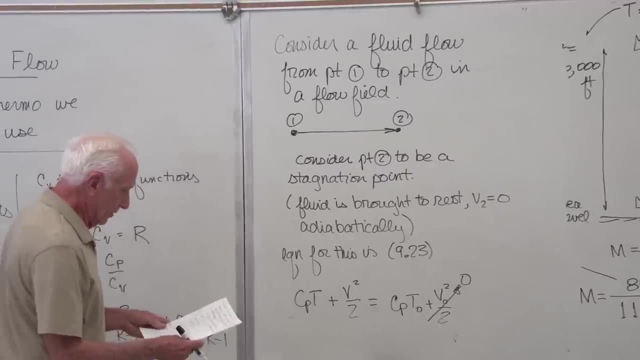 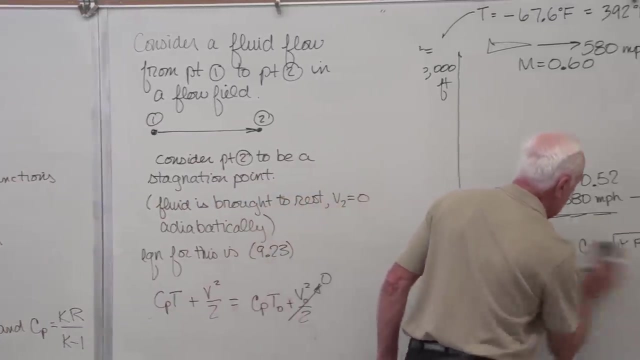 We it ignore the change in Z. Okay, so there's a number of assumptions in here. It comes from the energy equation of the fluid, but we're going to Solve that for stagnation point. So, okay, Let's go ahead and do that. 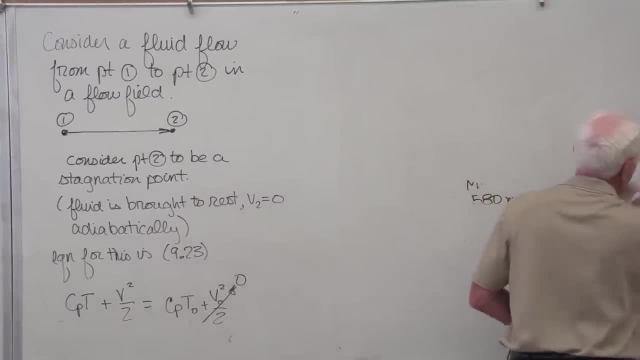 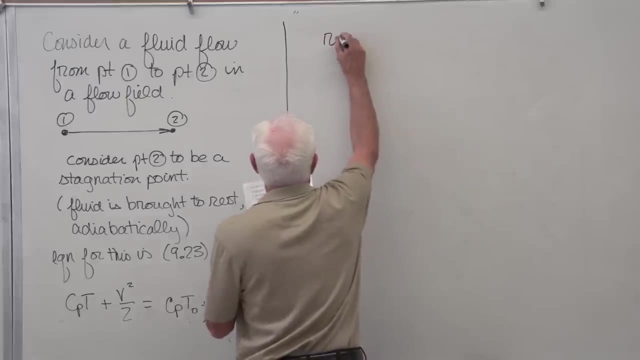 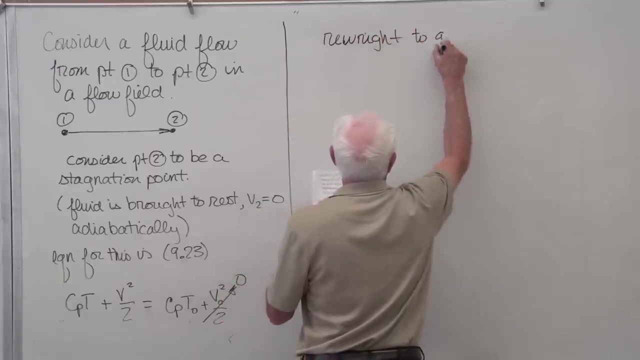 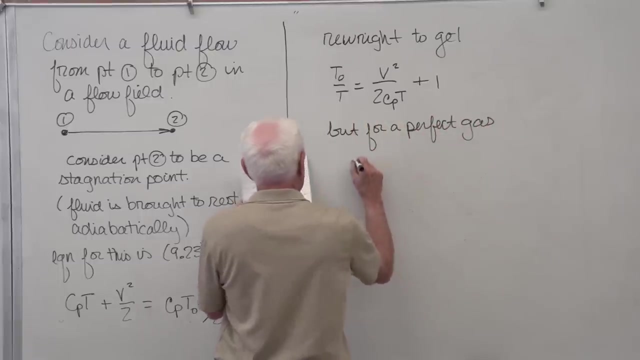 You, You, Okay, rewrite, and we get, if we rewrite this, T naught over T, V squared over 2, C sub PT plus one, But for a perfect gas, I'm gonna do it this way- Which is C. I'm gonna do it so that I'm going to writeanny. 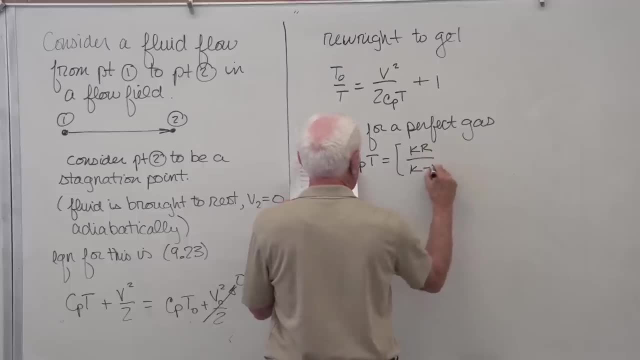 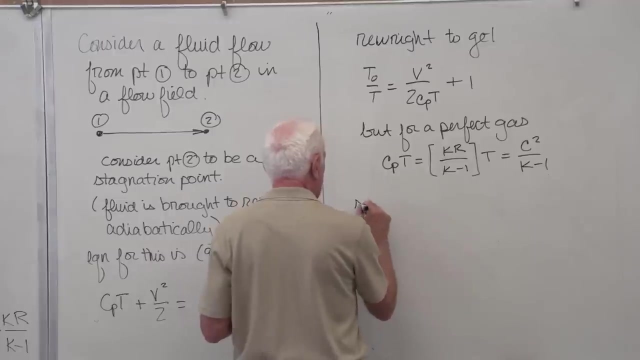 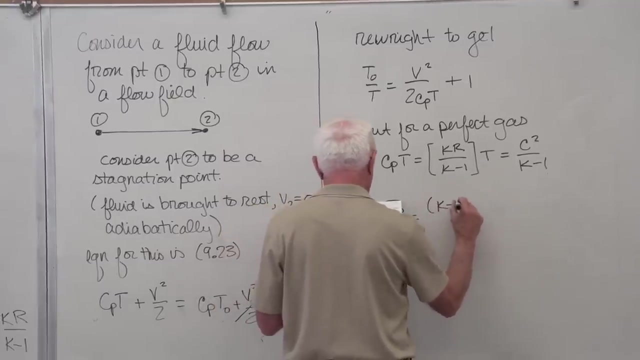 The value of T naught over T, V squared over T, V squared over 2, V squared- V squared over 2. therefore, Of T naught over T, V squared over T, V squared over 2, V squared over 2. I'm going to put this down here, then. 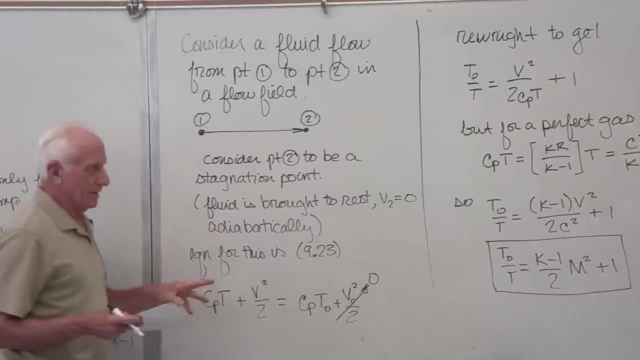 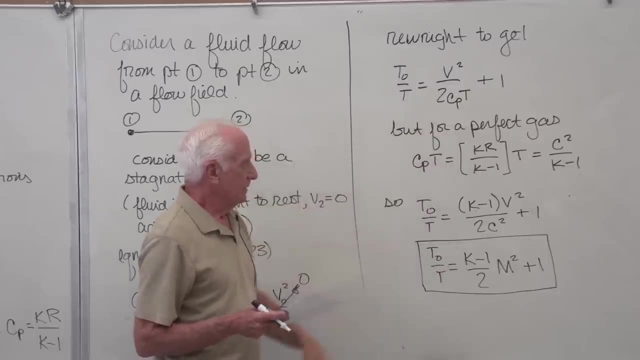 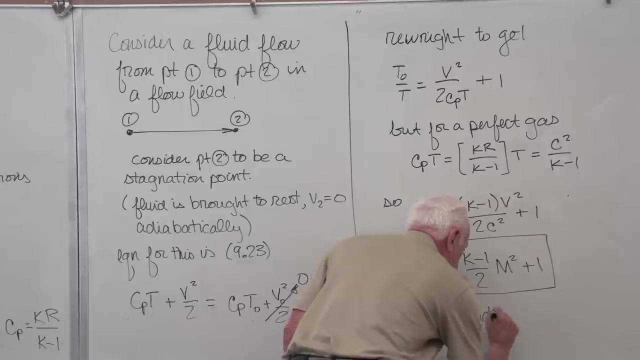 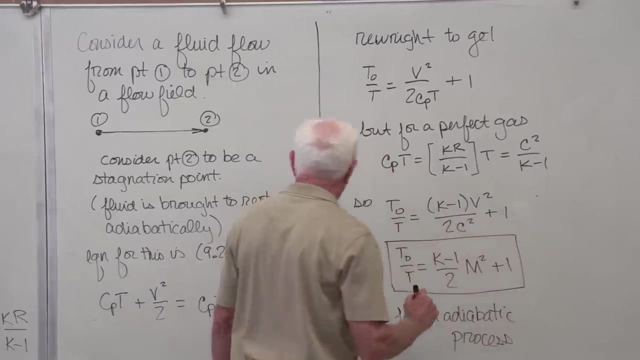 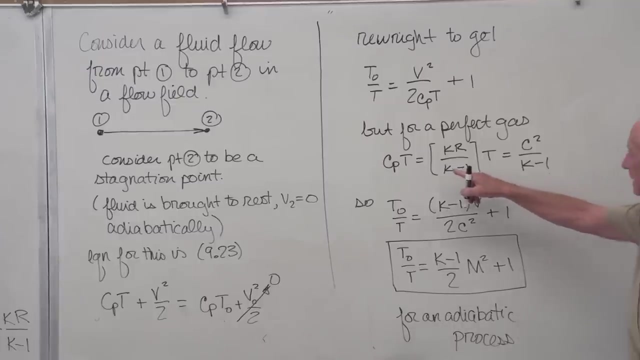 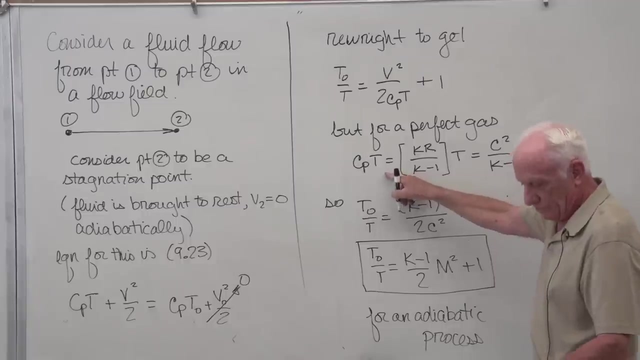 So I took the energy equation, I worked on it and I assumed a perfect gas and I end up with that guy. This is for an adiabatic process, This guy here. Let me show you where that guy there came from. 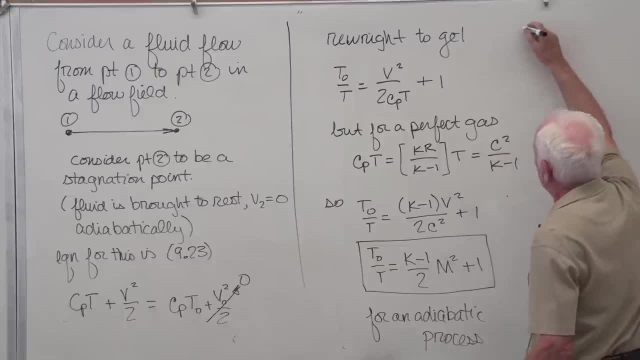 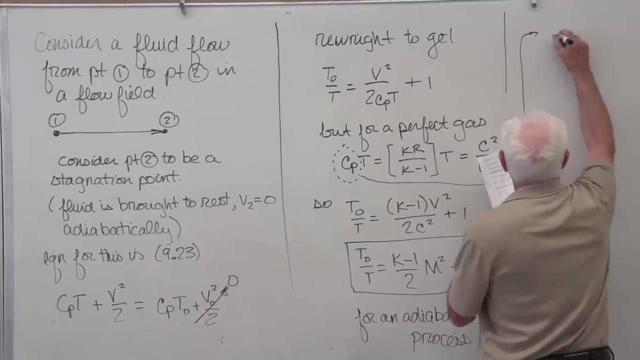 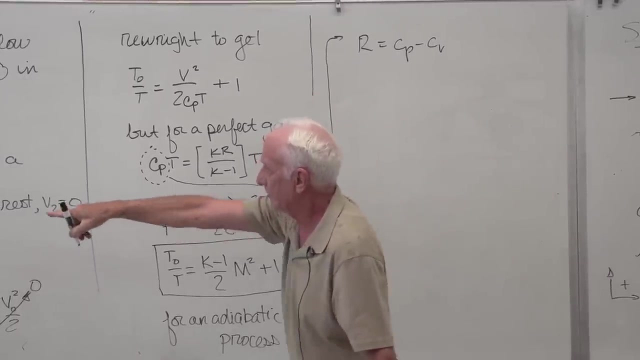 There it is. I'll put it up here. I'm going to get that C sub p R equals C, C sub p minus C sub v. Got that That's earlier on, probably over there somewhere. Yeah, right there. 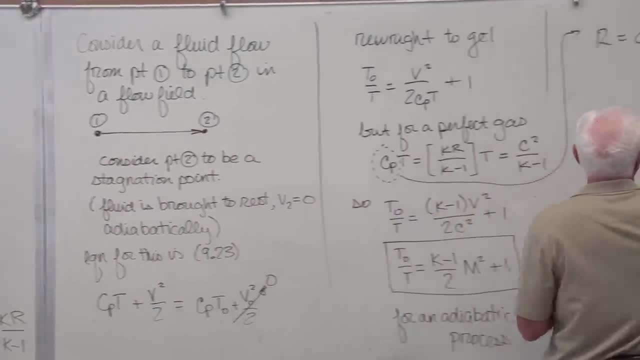 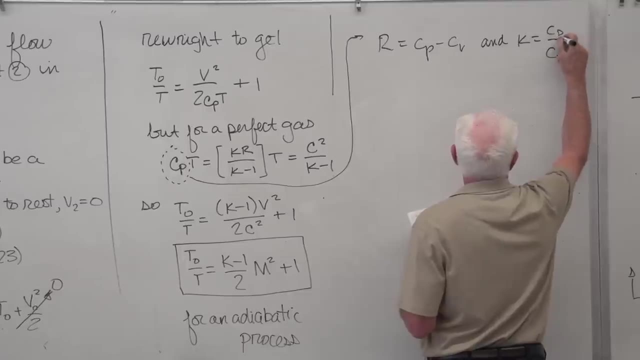 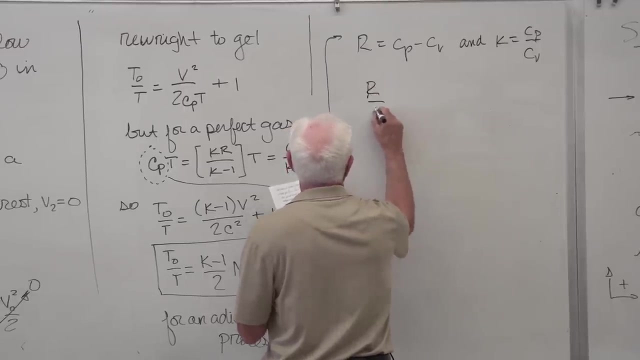 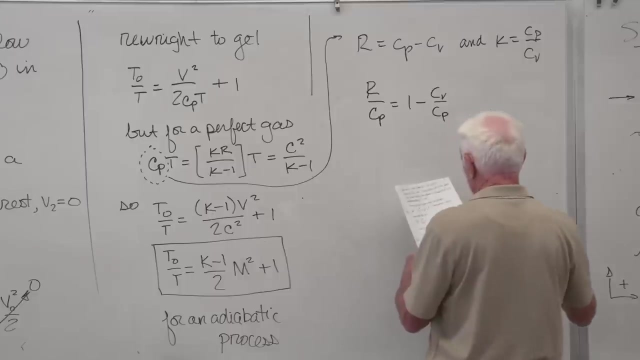 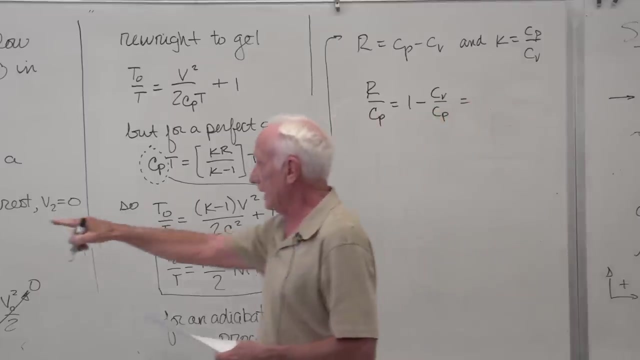 K is C sub p over C sub v. So take that R, divide it by C sub p, One minus C sub v over C sub p. This is equal to- and there's my K- C sub p and C sub v. 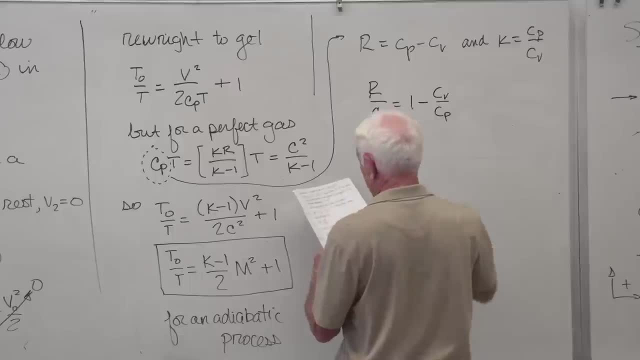 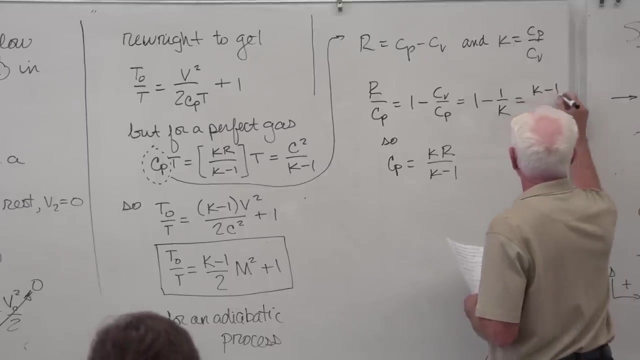 So when you bring in the value of K, you solve this guy for C sub p, K R over K minus one. This is one minus one over K. This is K minus one over K. So what is C sub p? Put C sub p over here. 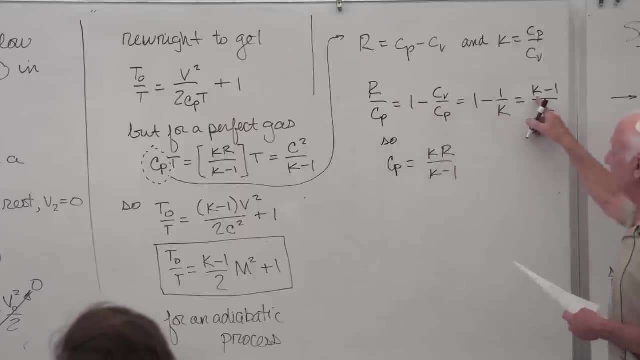 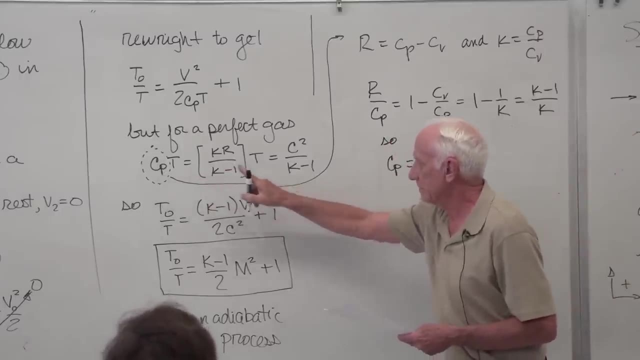 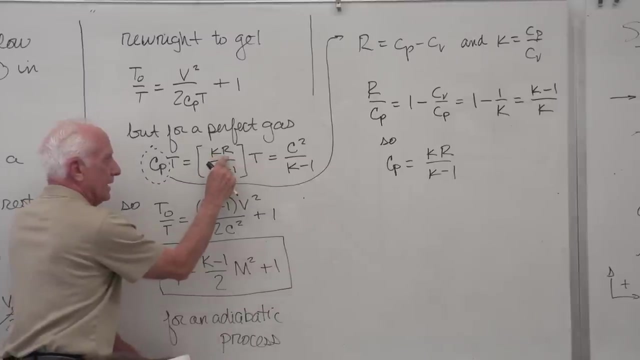 C sub p is K times R, Got it. Divided by what, K minus one, Got it. That guy goes in there and you get this: Okay, What is K times R times T? Oh, it's over there, probably. 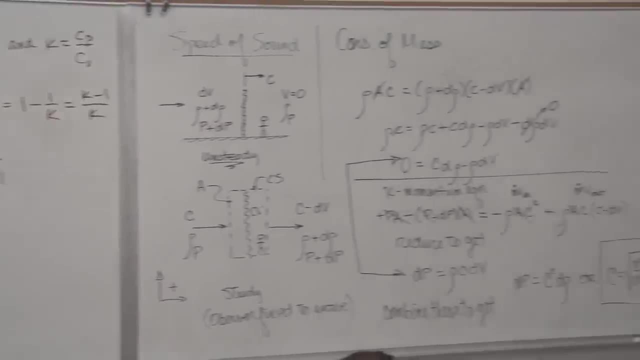 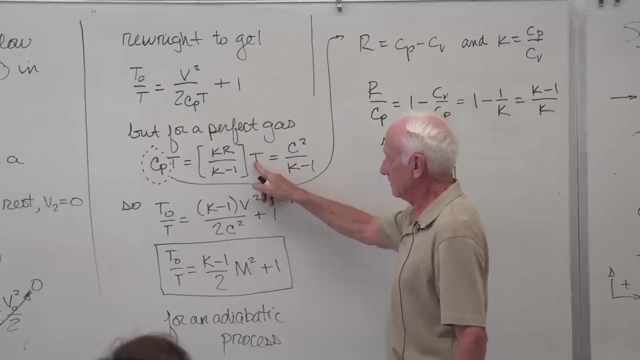 Speed is up right there. There it is Square root of K R T. This is the square root squared. so it's C squared. Okay, K minus one. K minus one. Put it in there. You have to go through all that. 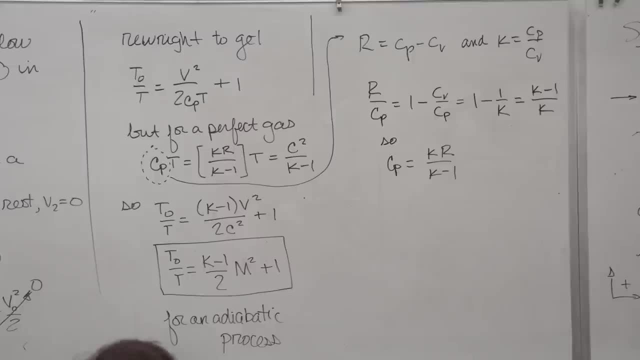 thermal stuff to do it. I'm just touching the surface. I'm just telling you. That's what you got to do. Compressible flow is very mathematically oriented. but that's the proof of that guy, in case you want to know. 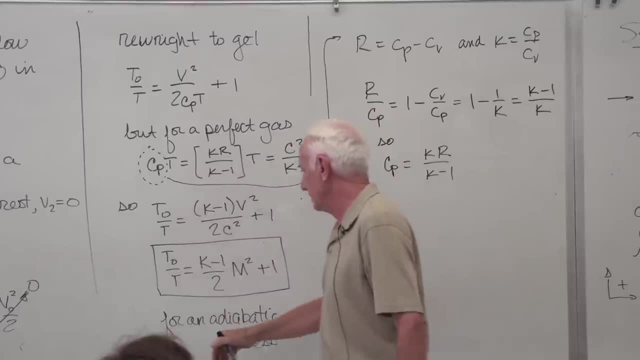 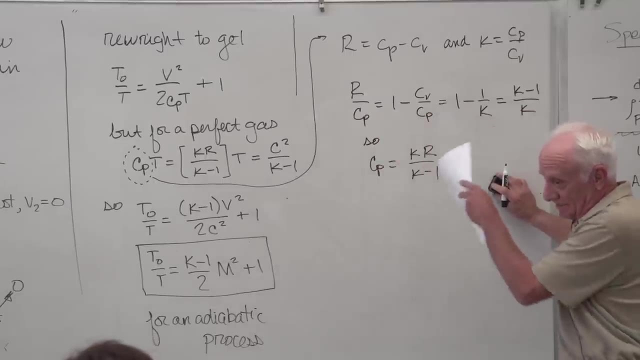 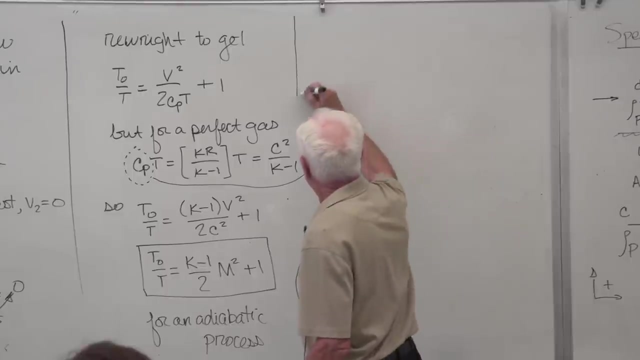 how you went from there to there. There, it is Okay. Now I'm going to erase this because I need this space right here. Okay, And I probably erased what I needed. Yeah, I think I did. Yes, I did. 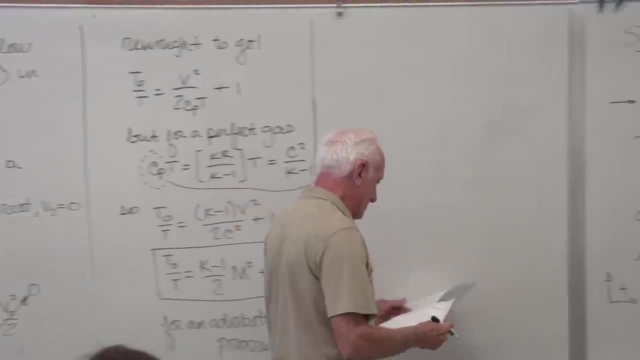 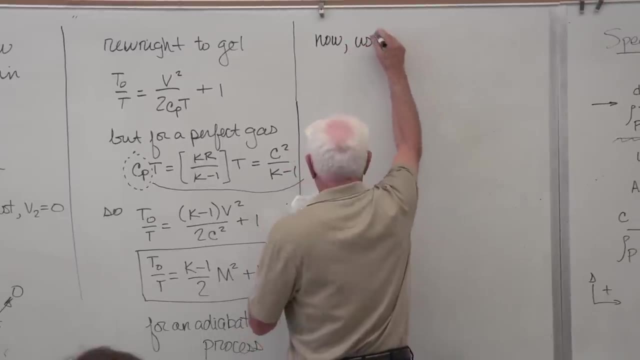 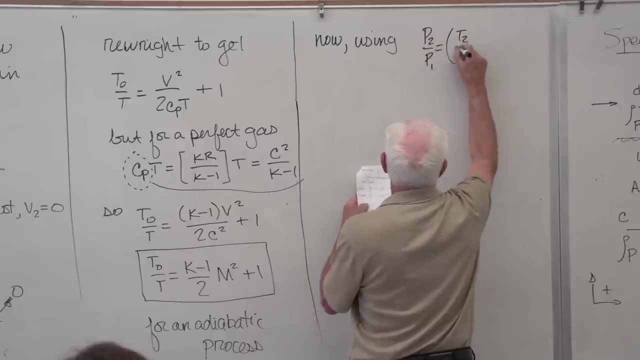 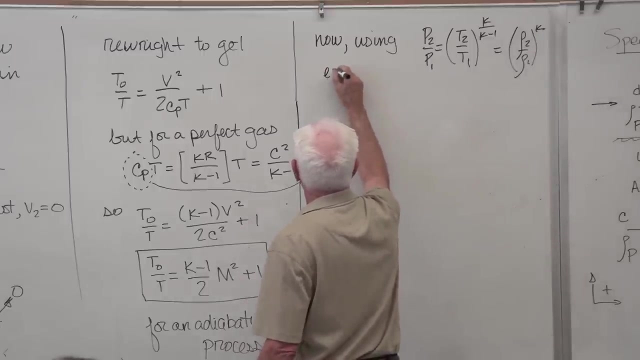 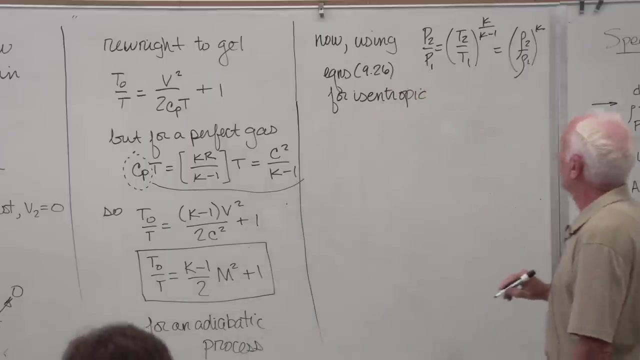 But over here I had those equations, I'll write them again. Okay, Equations 926.. What are they for? Isentropic, Got it? I'm going to get rid of that. T naught over T and I'm going to replace that. 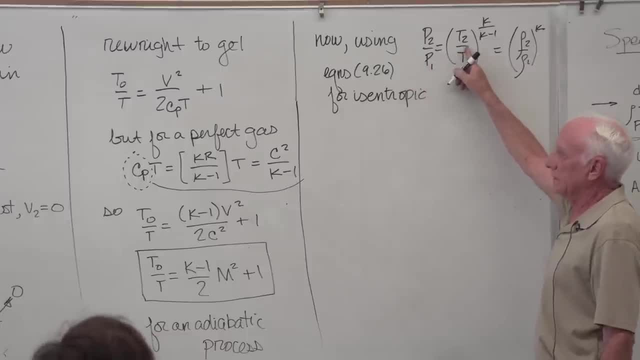 with a P naught over P. There's a T, What's point? two, T, naught. What's T? one T, T, naught, T, T, naught T. There it is. Take that guy right there and change that guy. 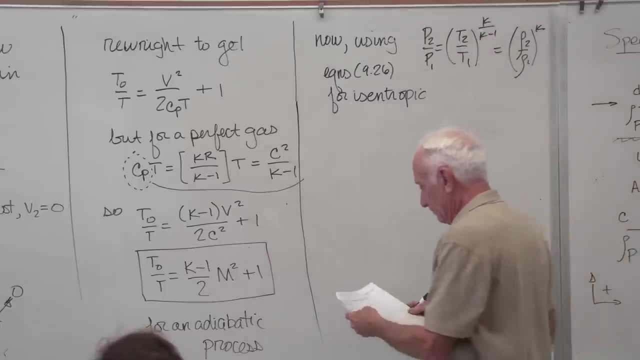 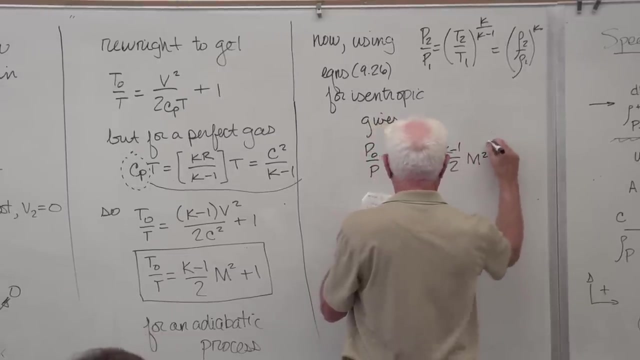 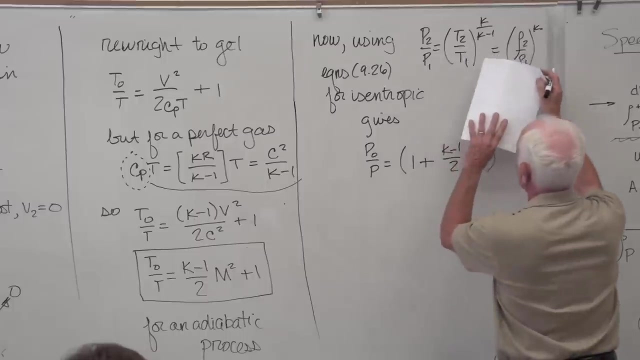 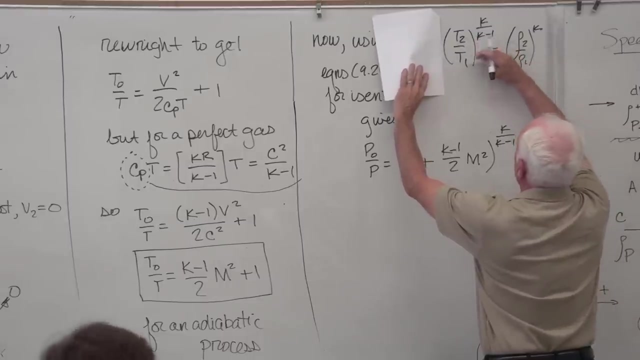 so it becomes P naught over P And there's a Rho naught over Rho. This is a T naught over T. This is a Rho naught over Rho. Convert that guy to Rho naught over Rho. 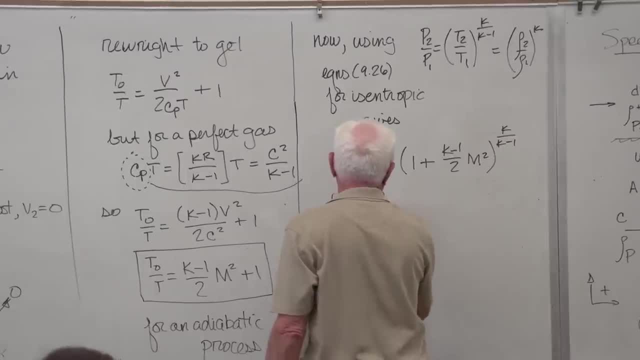 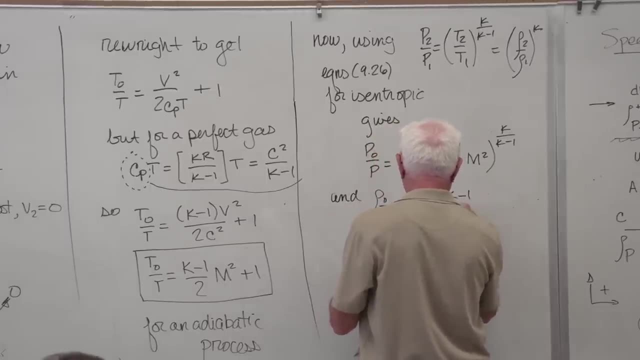 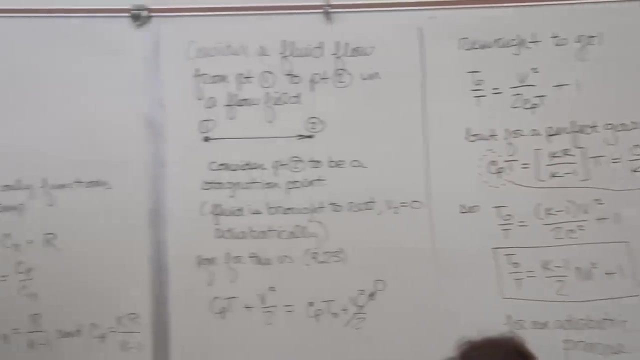 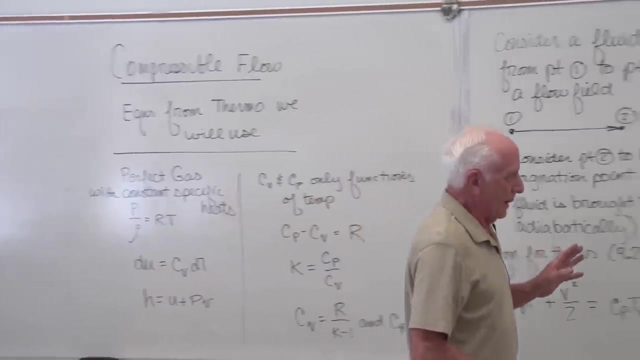 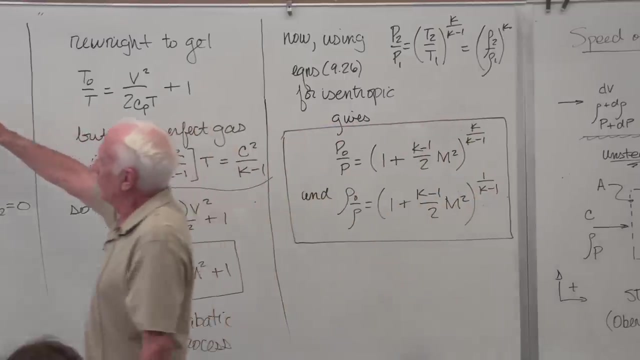 Those are the three equations that we will be using later on too. Okay, And what are they supposed to give you? Okay, Here's what they give you In a flow field from any point one to a point two, where point two is a stagnation point. 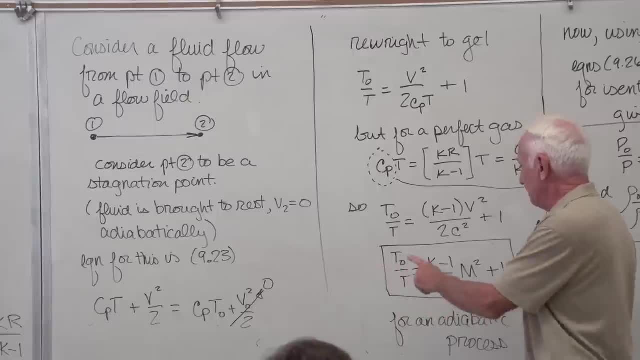 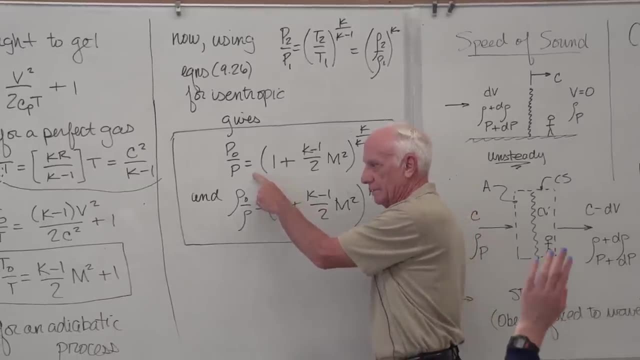 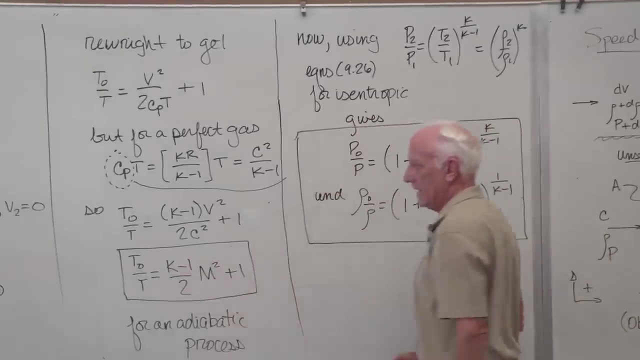 if you want to find the stagnation temperature, use this equation. If you want to find the stagnation pressure, use this equation. If you want to find the stagnation density, use this equation. K depends on the gas Air 1.4.. 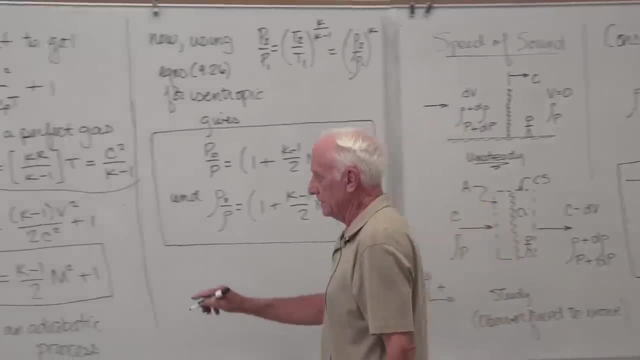 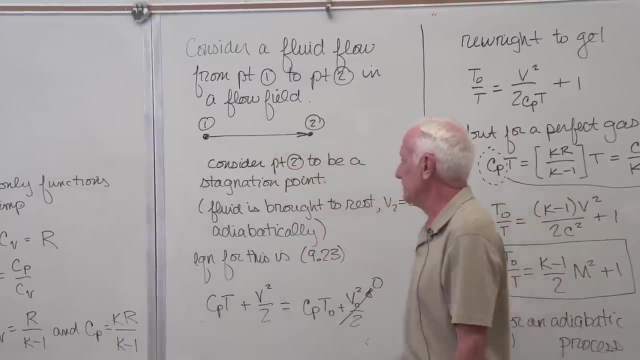 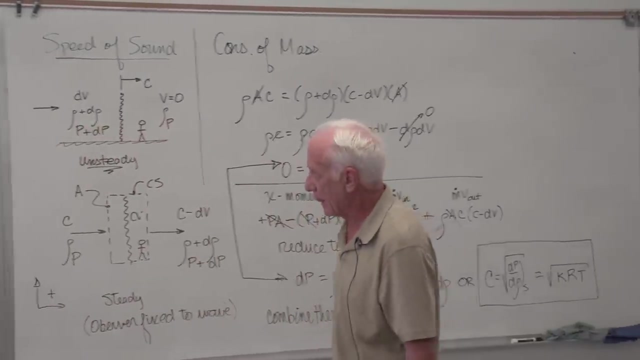 M is the Mach number, T is the temperature, P is the pressure, Rho is the density at some other point in the flow field, 0.1 in my picture. Okay, Professor, for the Rho equations, the last one. 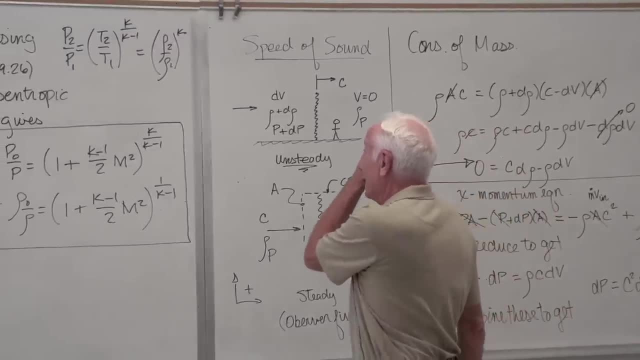 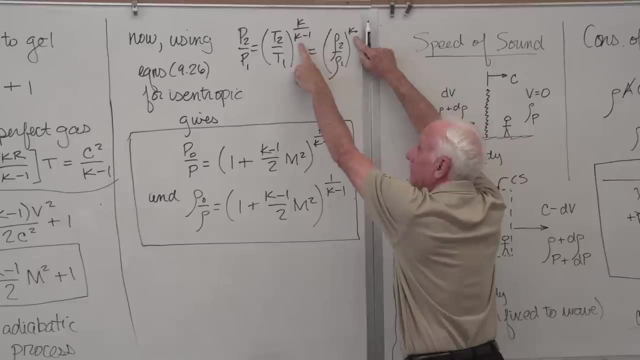 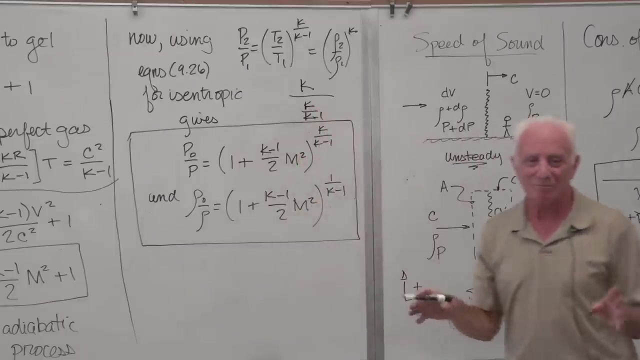 why is it that it's to the power of one over K? Yeah, See these two guys here. What if I divide one by the other? Do the Ks cancel out? That's the game, The little math game in there, you know. 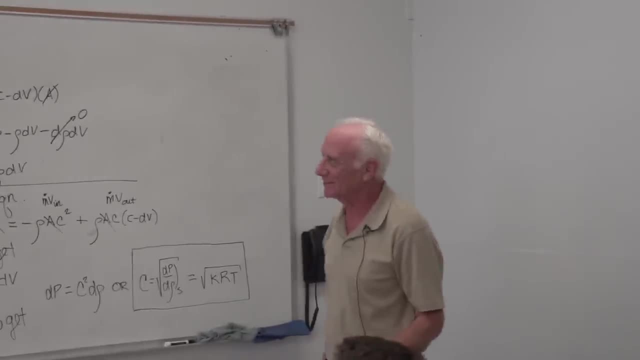 You're going to find out when you do that that you're left with K minus one, only One divided by K minus one. Yeah, Like I say, there's a lot of math between the lines to go through every gory detail which we don't have time. 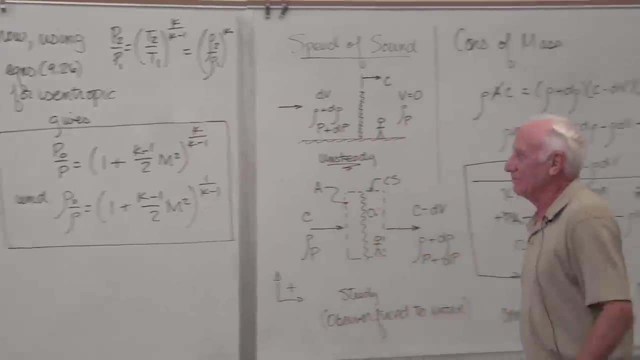 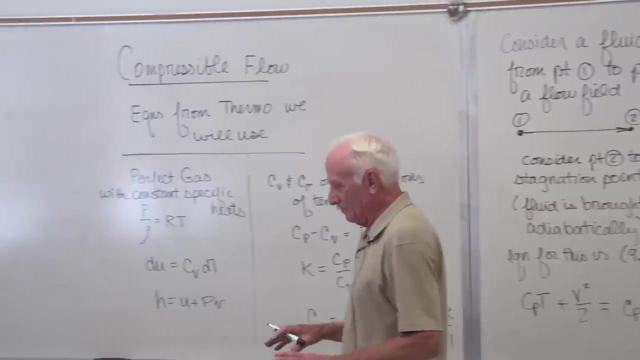 to go through every gory detail, But that's a good point. Thank you, Okay, Good. So this is going to give us a good starting point and we're ahead of the game on compressible by almost a week, which is great. 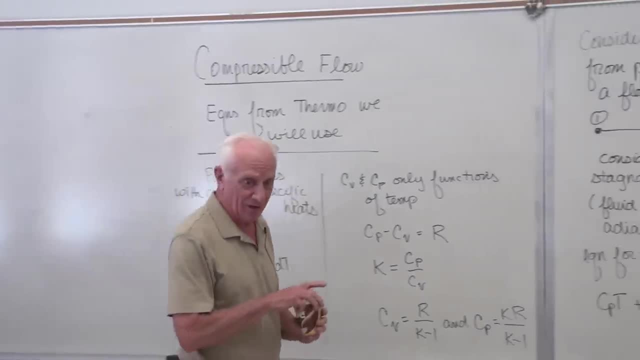 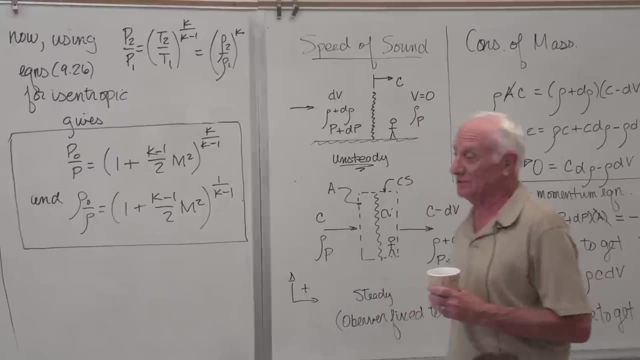 We need that time at the end because we've lost two holidays in a 10-week quarter. So we're going to be moving fast in the last five weeks. We moved pretty fast in the first five weeks too. Okay, So let's talk about 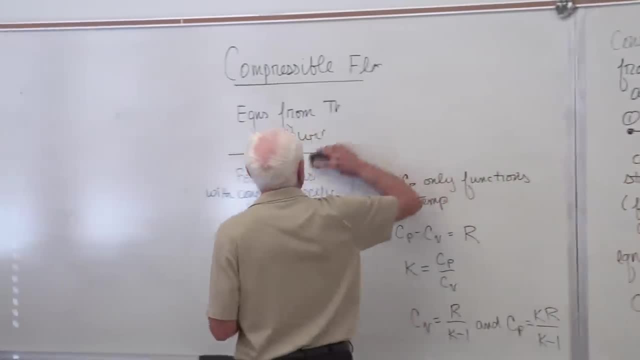 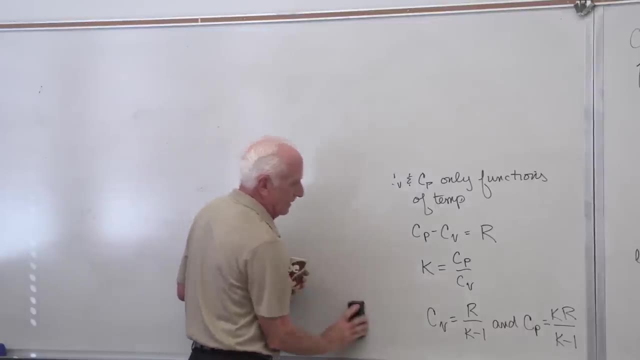 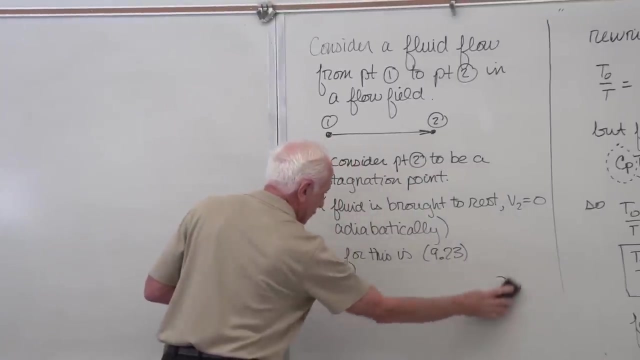 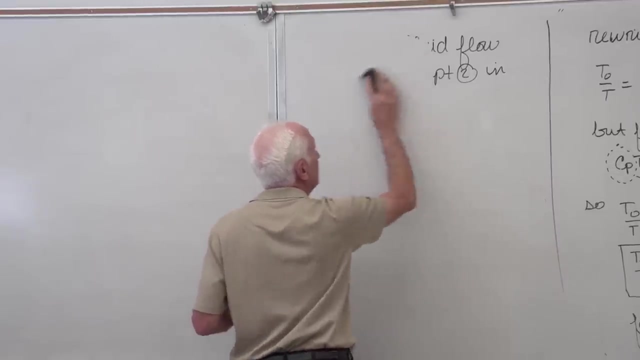 the midterm coming up on Wednesday. Okay, It will be the full 75 minutes. Okay, There will either be three or four problems, depending on how long they are. three or four problems. You'll be given a data package when you come in for the midterm. 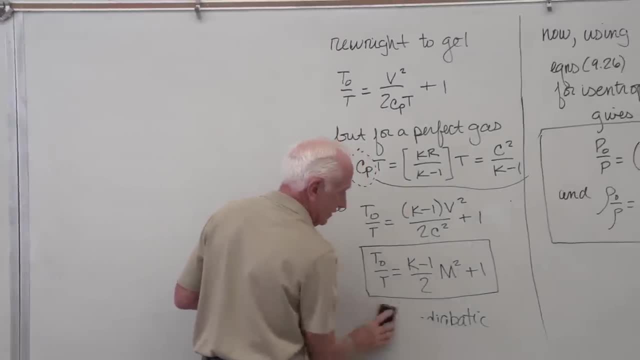 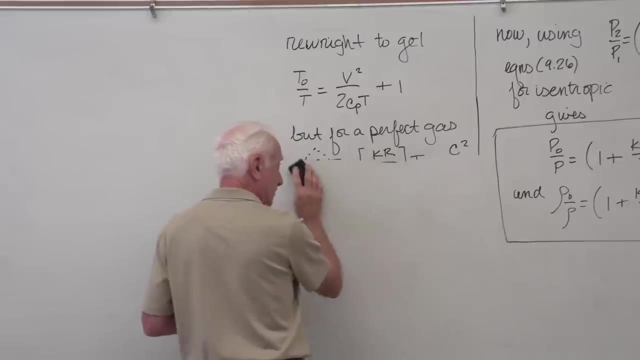 You'll put your name on the data package. You'll turn it in at the end of the test with your exam. Keep the data packages. I turn it back to you for the second midterm with your name on it. You turn it back in. 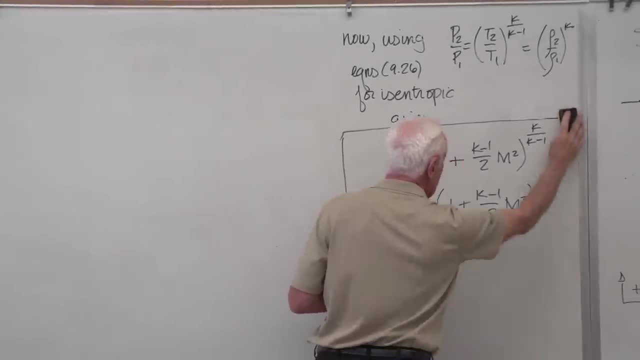 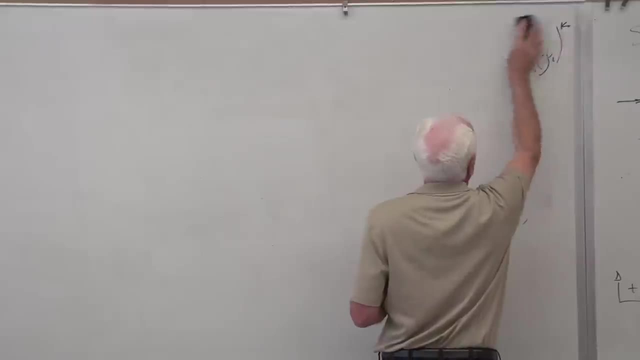 at the end of the exam And then I give it to you before the final exam in class time And you use it and you turn it back in when you're done. So it'll be your data package. You can mark it up if you want. 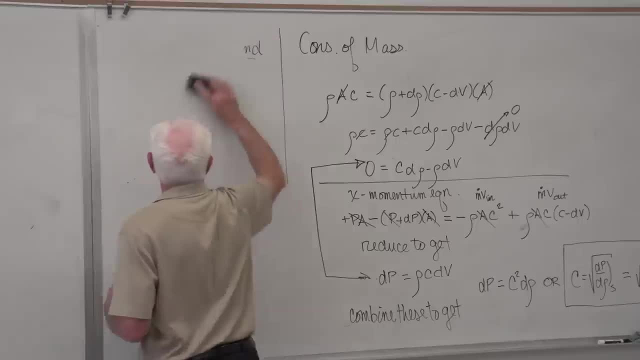 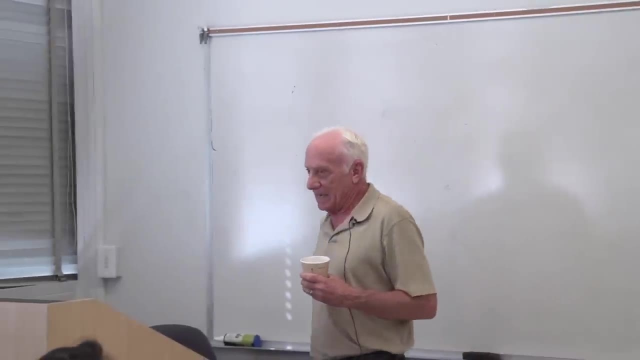 You'll get it back for the first midterm, the second midterm and the final. The one on Blackboard website is almost correct, but I had to add a Moody chart, So the one you'll get for the exam has a Moody chart attached to it. 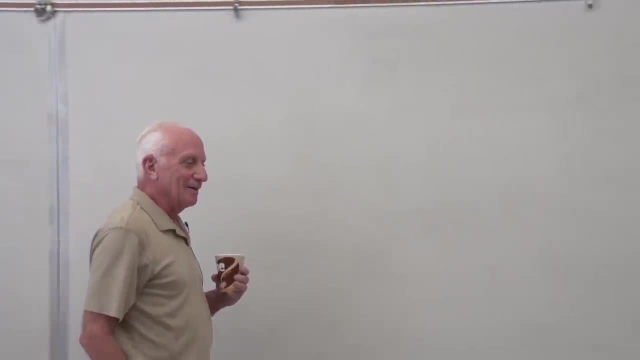 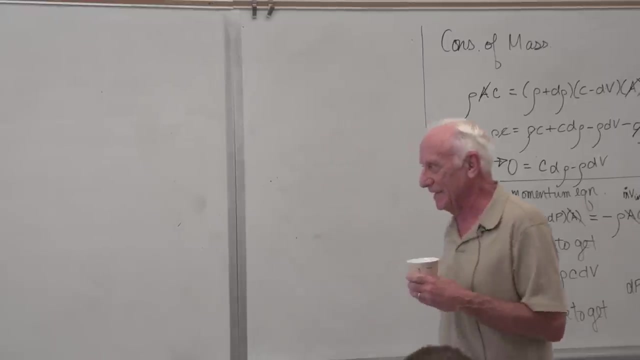 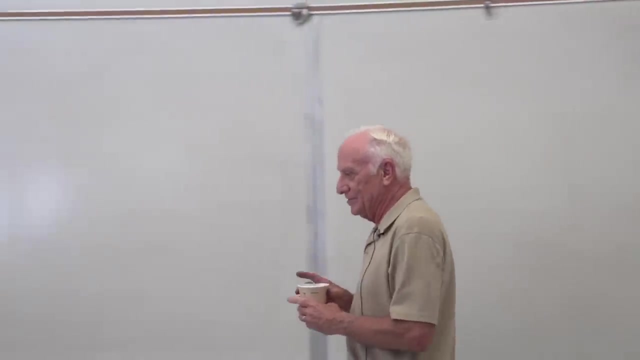 because it's not what's on Blackboard. So the only difference is there'll be a Moody chart attached which is not on the Blackboard. example of the data package: You're allowed to bring in with you one equation sheet, both sides. 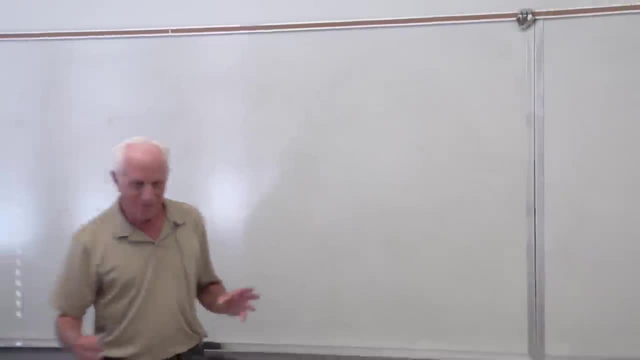 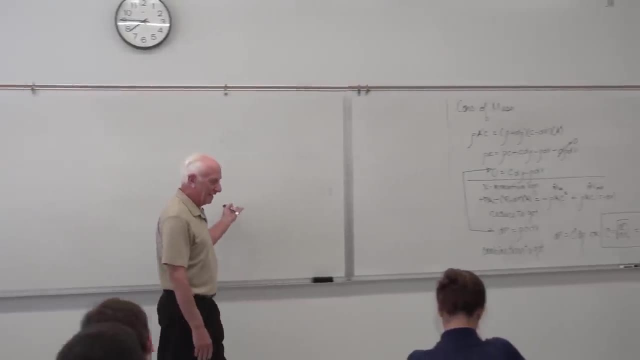 eight and a half by eight by 11.. Anything on that is legal. Anything on it is legal. Homework problems. example: problems from the textbook stuff I had in class. You should, of course, try and put all the equations I boxed in class on there. 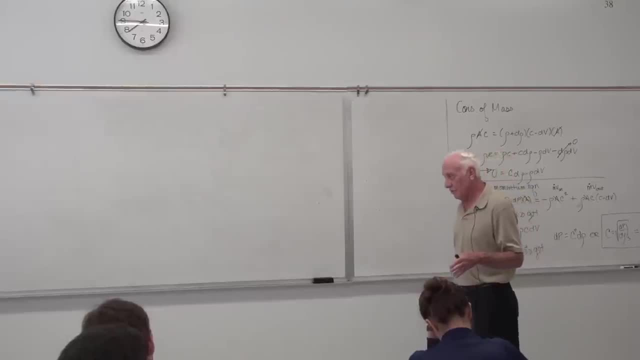 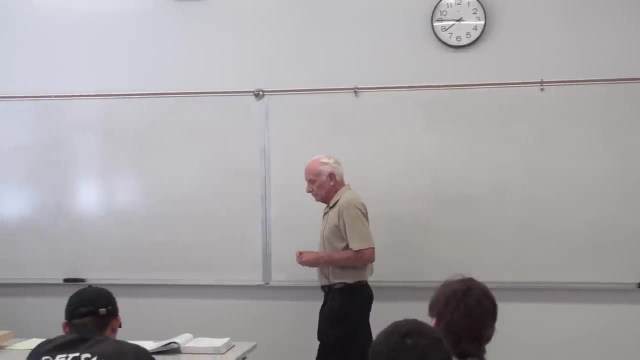 plus whatever else you might have used for homework. Any equation used for homework- or I used up here to solve a problem on the board, as example, should be on that equation sheet. Let's see What did I miss Anything? I don't think so. 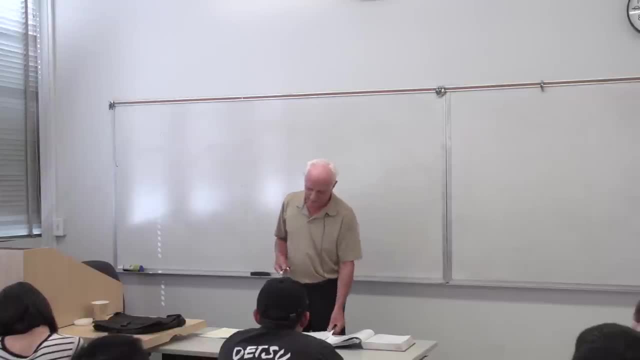 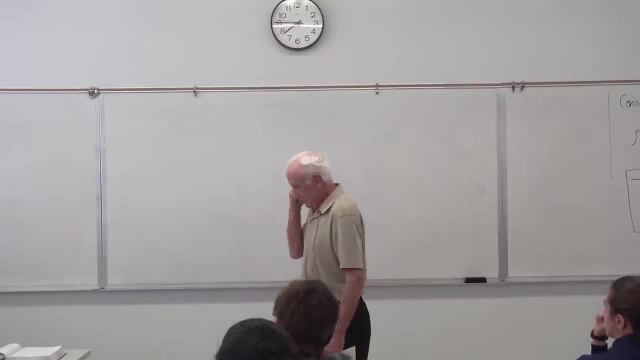 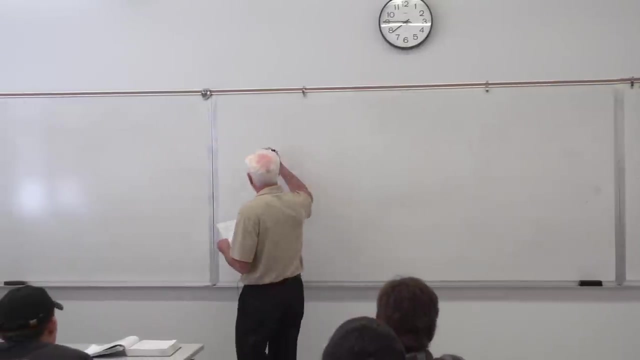 So here again, this stuff should be pretty fresh in your mind. You went through the example that the first midterm from the fall quarter, so you know what I asked there. But here's kind of you know what we're covering. 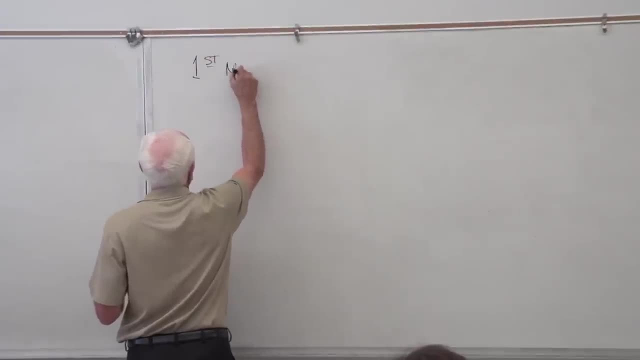 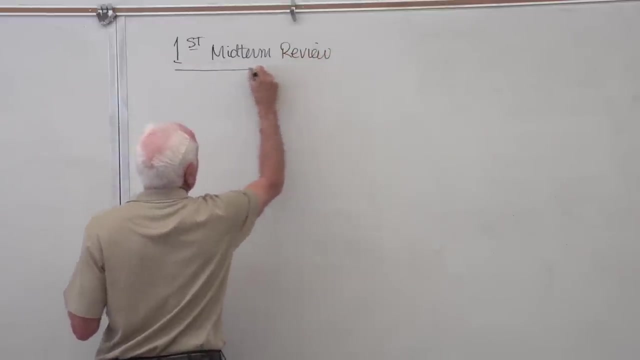 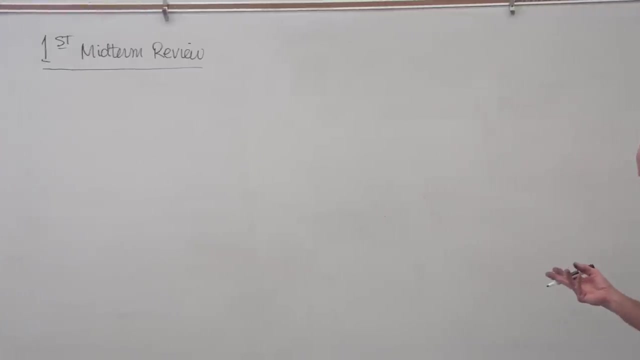 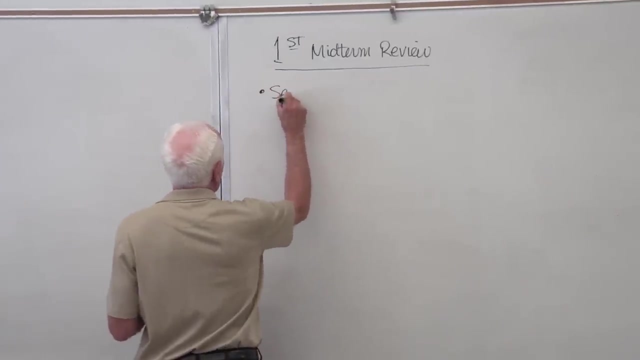 So first midterm review And if you have any questions, I've got a two hour office hour tomorrow. I've got a one hour office hour on Wednesday. Okay, so three hours. you can come and see me with questions. Obviously, series pipes. 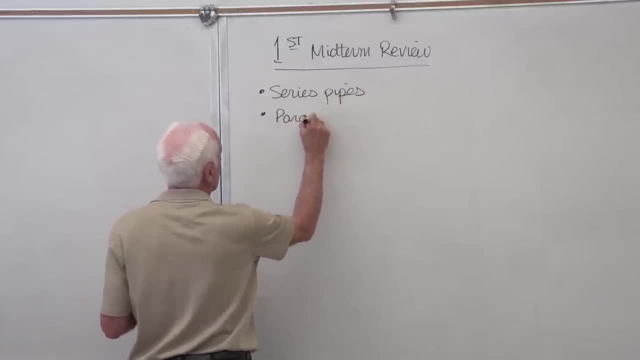 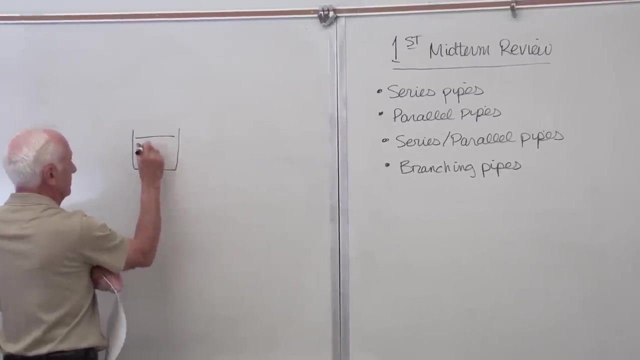 parallel pipes, a combo problem series, parallel branching pipes. So we worked one of each of those in class and you had some for homework. We looked at two configurations about the series in parallel. Here's one and the water flows down in pipe one. 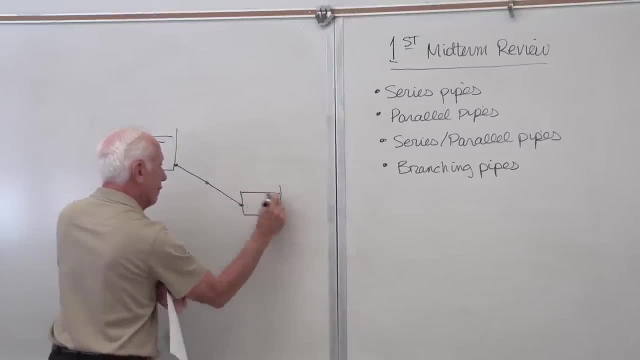 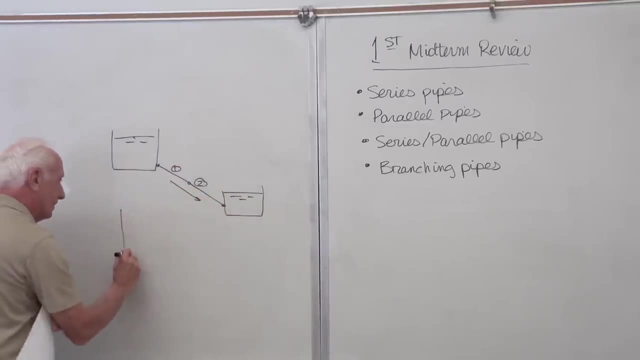 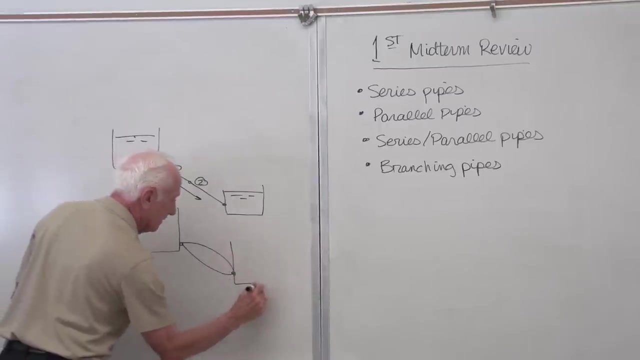 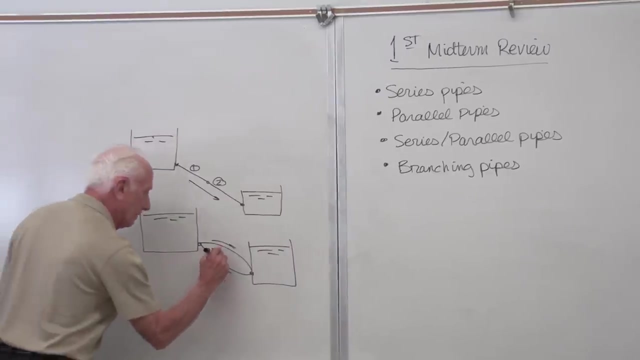 and the water flows down in pipe two. This is pipe one, This is pipe two, Then we have one here and here and here. Water flows down there. Water flows down there, Here's pipe one, Here's pipe two. You can carry it on and on. 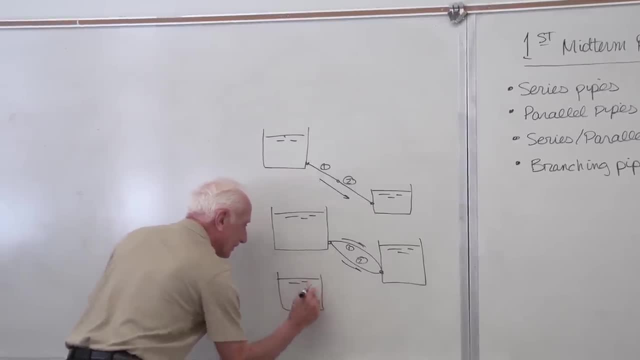 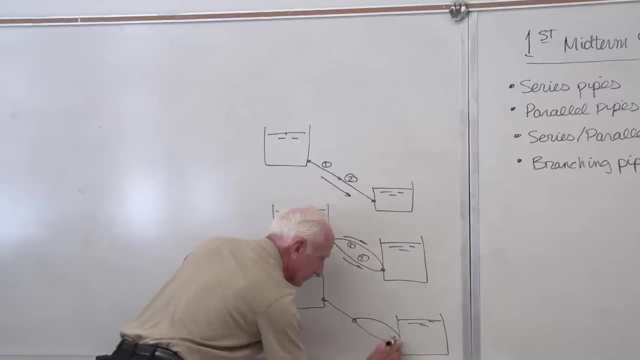 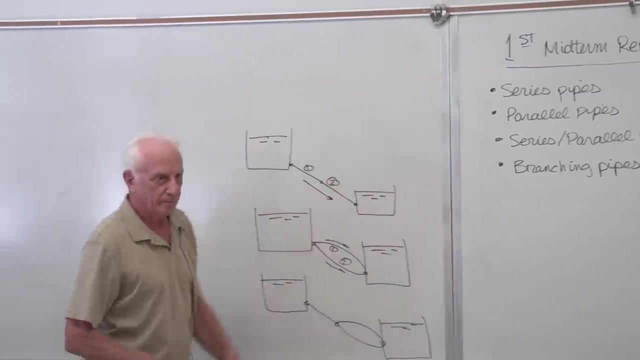 I'm going to get. I'll do one more for you. Here's one here, Here's one here. Comes down here, branching pipe. You get the point: Series pipe, parallel pipes, series parallel pipes. one of each, It could be. 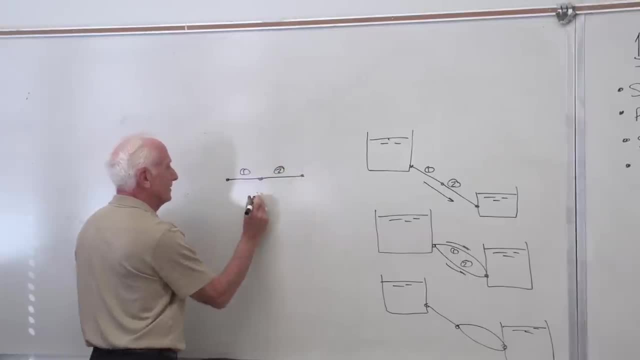 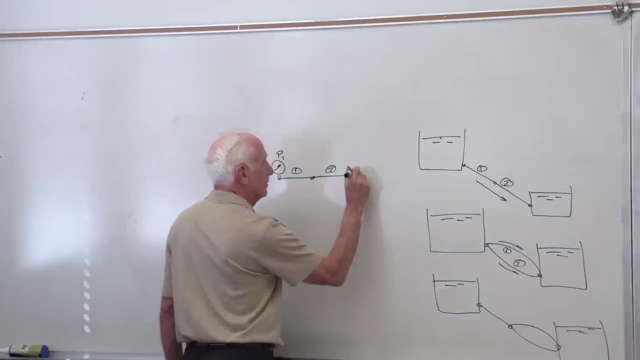 I guess I'll go through them. Why not One? two: Put a pressure gauge here, P1.. Put a pressure gauge here, P2.. Okay, Given P1 and P2, find the flow rate Q, Given Q. 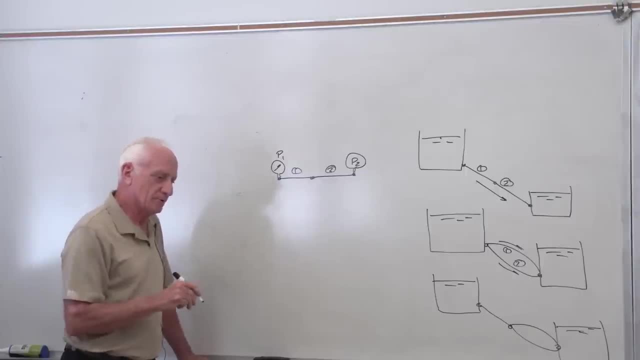 find the pressure drop across pipe one. Find the pressure drop across pipe two, Given Q. Here's a pressure gauge here. Here's a pressure gauge here: Pipe one, pipe two: Pressure gauge here: P2.. Flow rate comes in here. 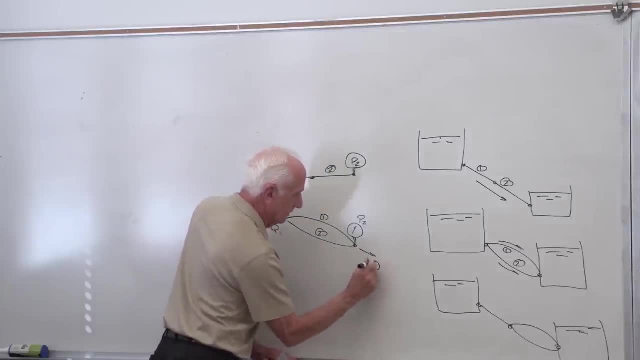 Q1, Q Flow rate goes out here: Q. This flow rate: Q1.. This flow rate: Q2.. This flow rate: Q1.. This flow rate: Q2.. Flow rate: there's Q Flow rate. 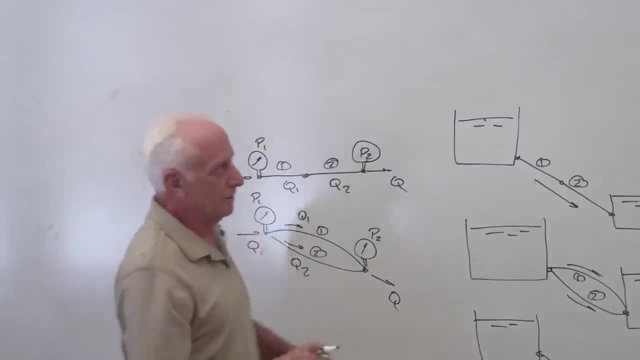 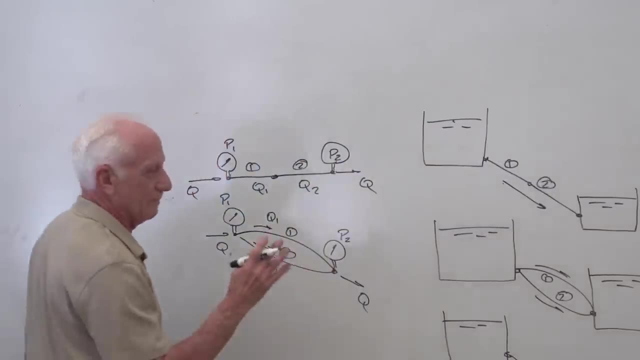 there's Q, This kind of problem, that kind of problem For what? Series pipes, parallel pipes, all pipes, Now the branching pipes. I'm not going to go through that. We did a problem in class. You had a problem. 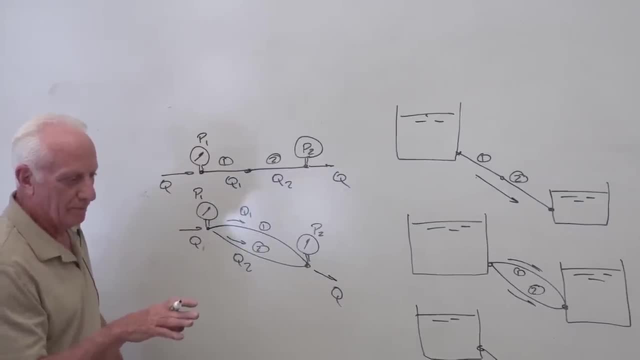 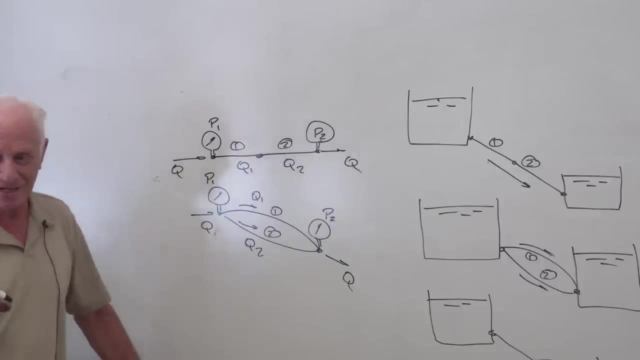 in homework, like that, But there won't be more than three reservoirs. okay, You could have more than three reservoirs, But for homework you only had three. For the exam, the max you can have is three. I won't do any more than three. 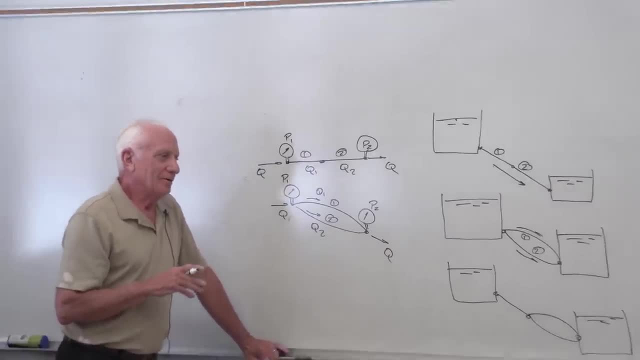 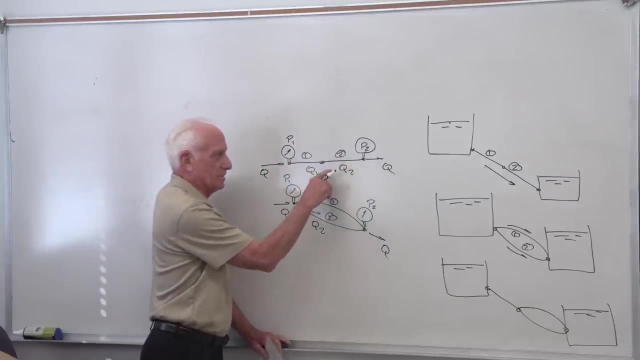 so three pipes. I'll just tell you one more time If you don't know Q when you start. if somebody gives you the pressure drop here and says what is Q? Somebody gives you the difference elevation and says what is Q1 and Q2?? 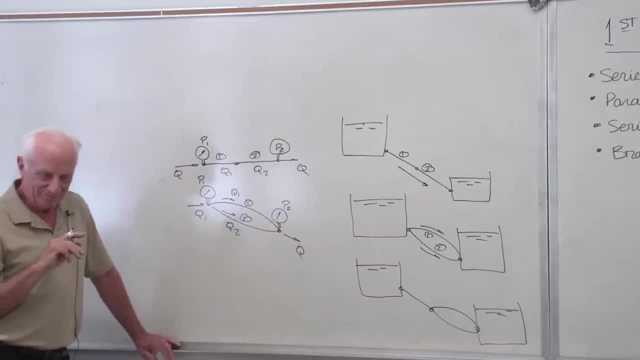 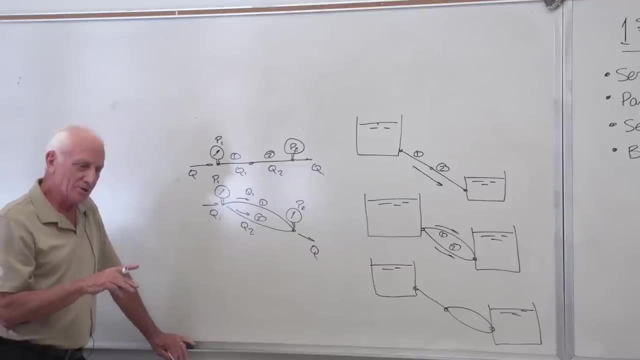 You guess the friction factors. You go through it and you get the velocities in the pipes and then you get the Reynolds number in those pipes. Go to the Moody chart, see if the F value from the Moody chart is what you guessed. 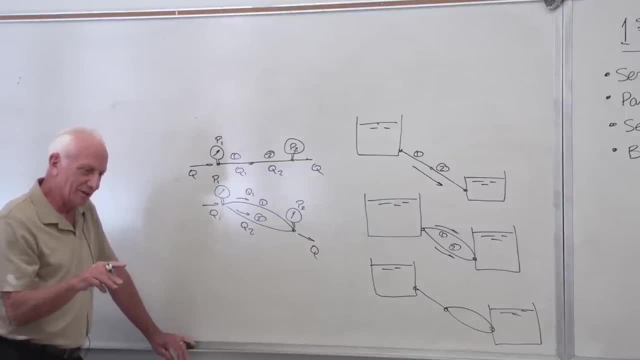 If not, you say in words: I would repeat the above calculations with these new F values: F1, new- equal fill in the blank. F2, new- equal fill in the blank. but don't do any more work. 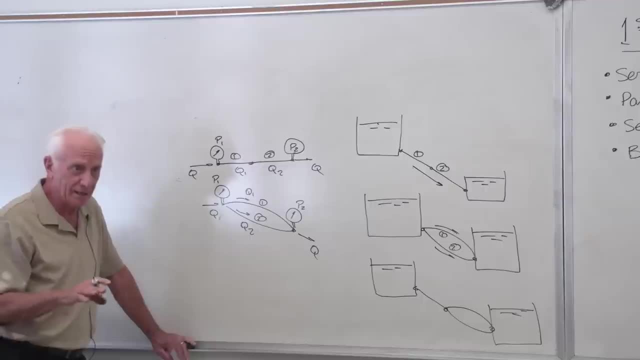 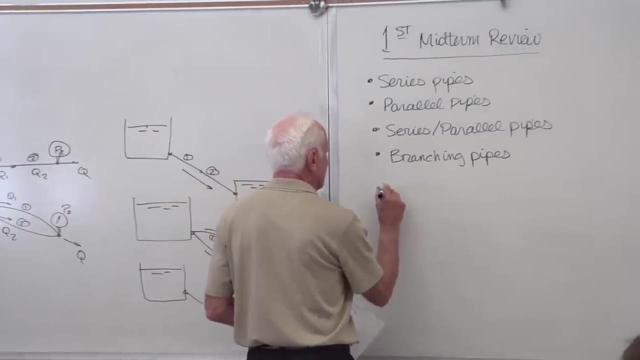 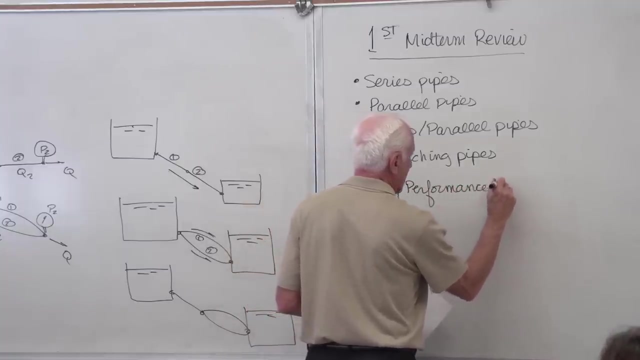 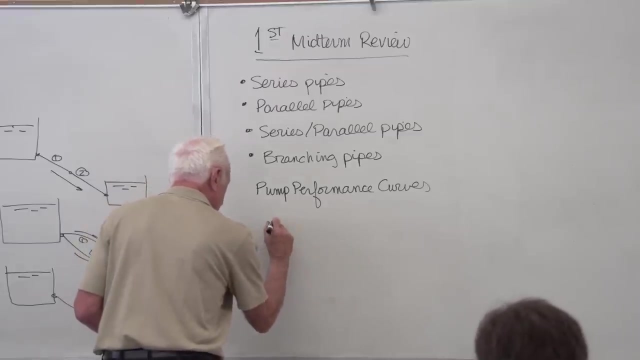 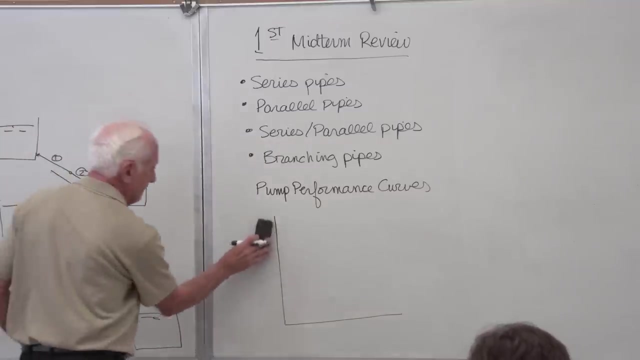 Don't iterate. Go through it one time and tell me what your next F guess would be. Now let's go to pump performance curves. We talked about typically centrifugal pumps. It would be centrifugal pumps. This could be, for instance: 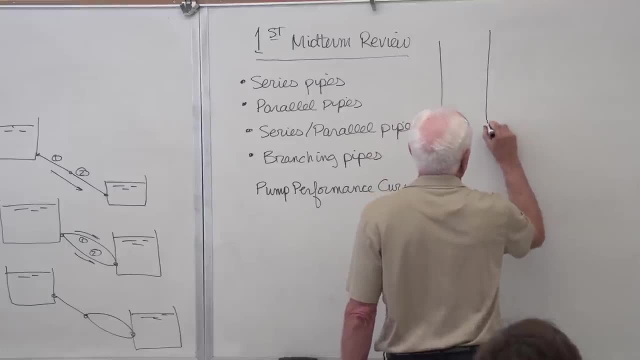 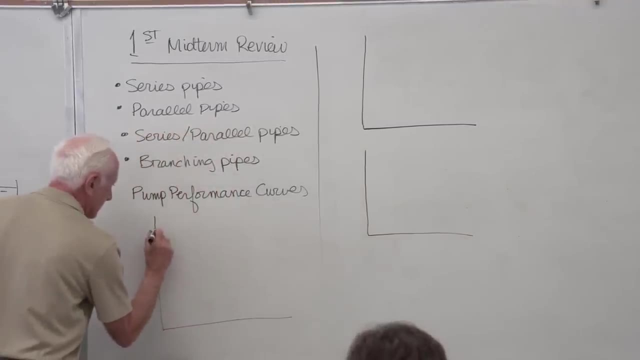 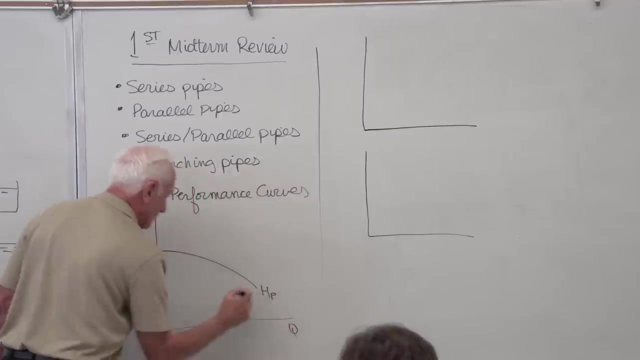 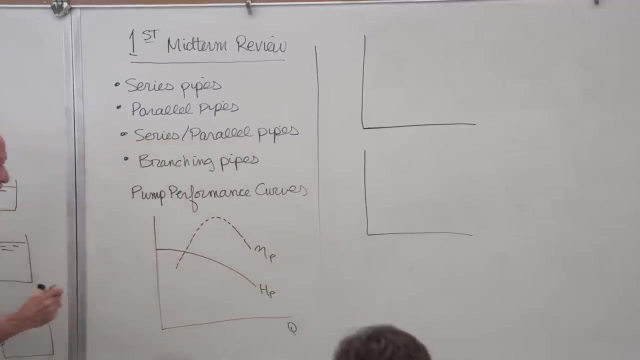 let me do it this way. Okay, let me just show you. I'll do one over here. You can be given the pump head, curve Q versus the pump head, and you could be given the pump efficiency curve. Okay, that's a pump. 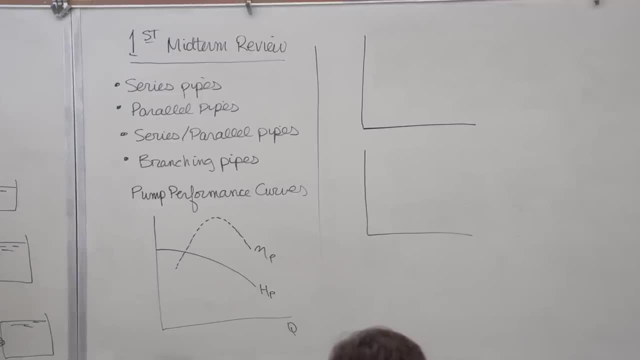 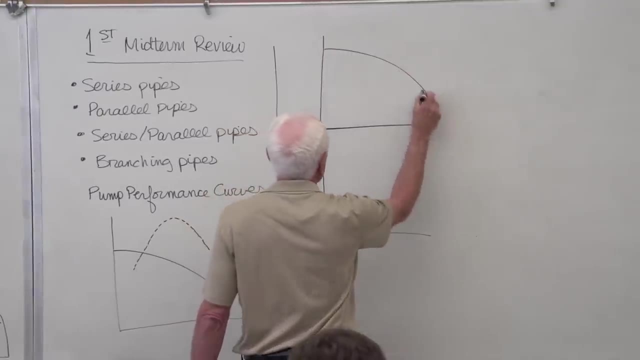 performance type graph: Pump head versus flow rate, efficiency versus flow rate. or you could be given one, like I had before, where this is the pump head and these are the efficiency lines here. Okay, and then down here is the power into the pump. 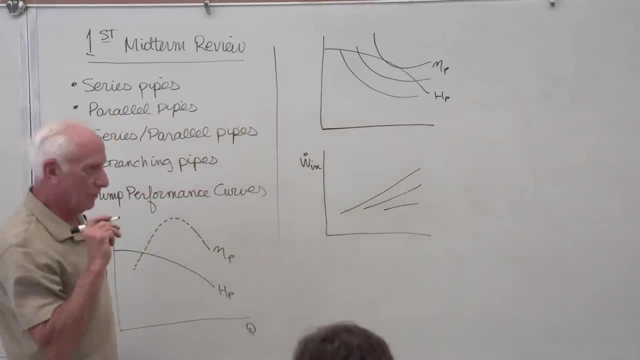 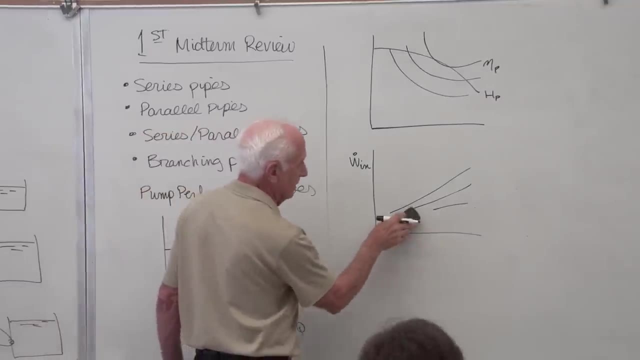 from what a motor? Yeah, power into the pump. There were different pump impeller diameters, but I'm not going to get that. It looks like that. And then down here is the NPSH. Okay, so again. 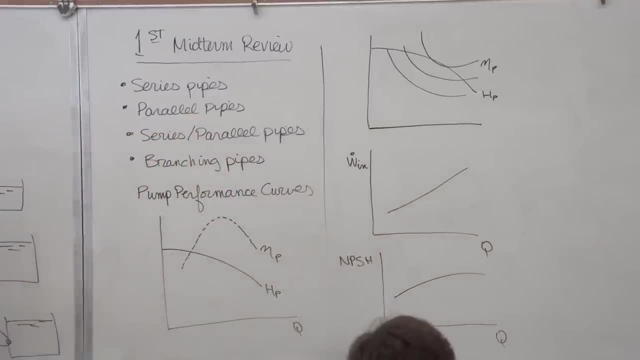 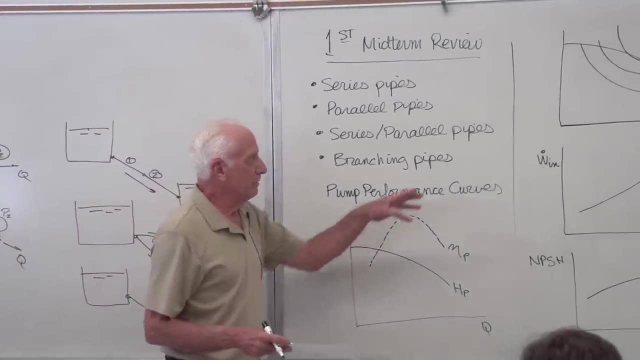 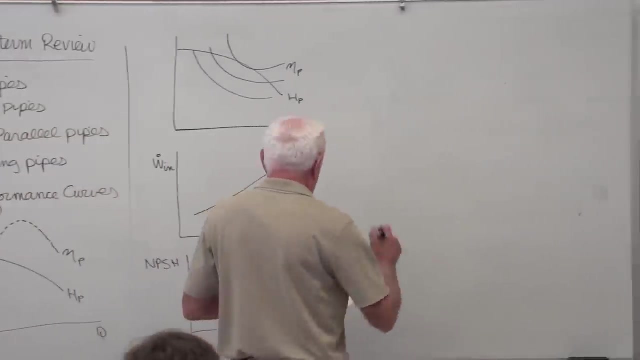 one curve there, NPSH. Those are all pump performance curves, So just be aware of the different ways that pump performance can be given to you. A graph like that with efficiency, or maybe a graph like that with efficiency. Okay, Obviously fine. 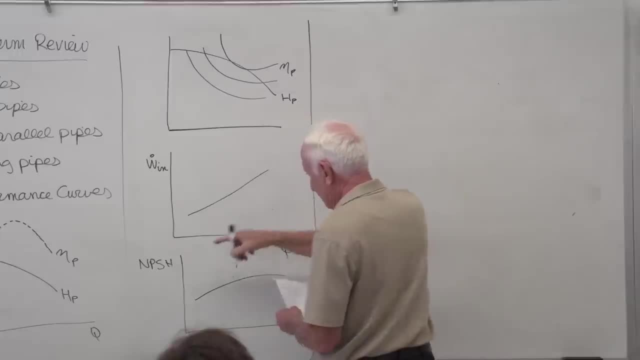 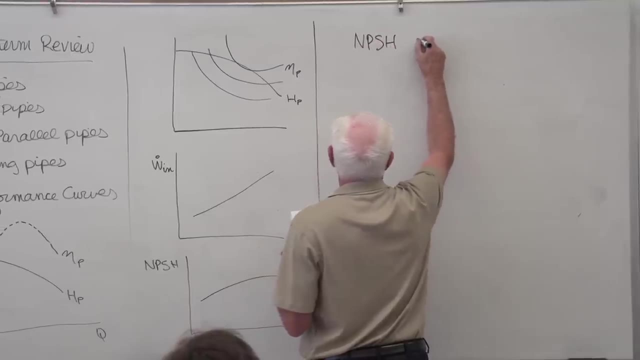 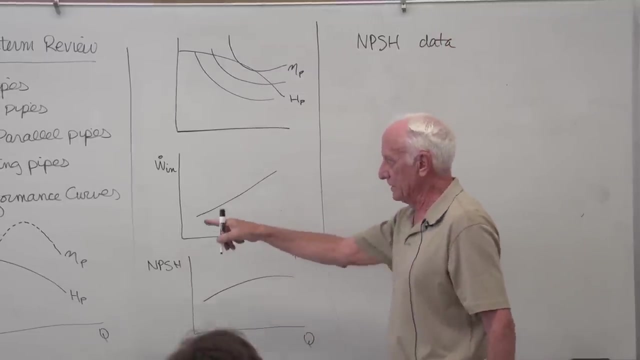 let's just stick with the pumps. All right with the pumps. know how to operate with NPSH. So NPSH data and we have that given. It's on here, It's on most of these guys on this graph here. 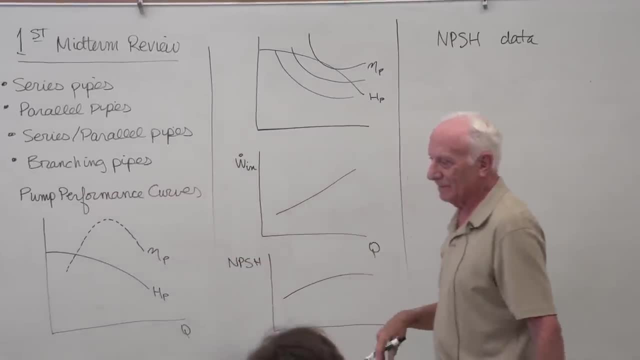 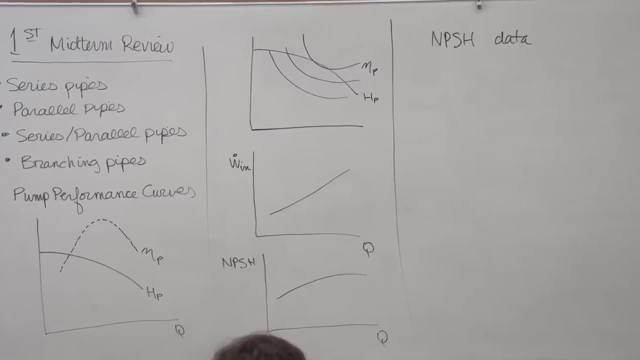 It's stuck up here at the top so it separates it out of the way, But the graphs have NPSH on. What is that supposed to give you? Well, if you're worried about cavitation, then you better use NPSH. 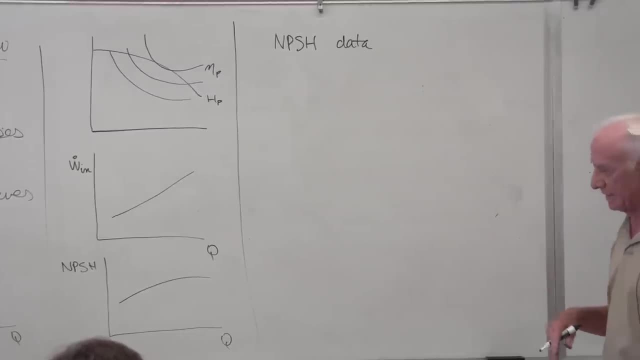 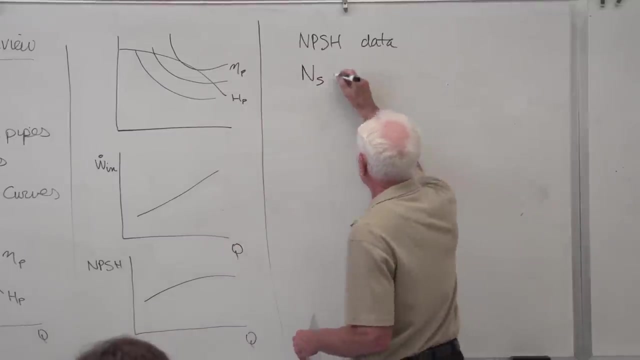 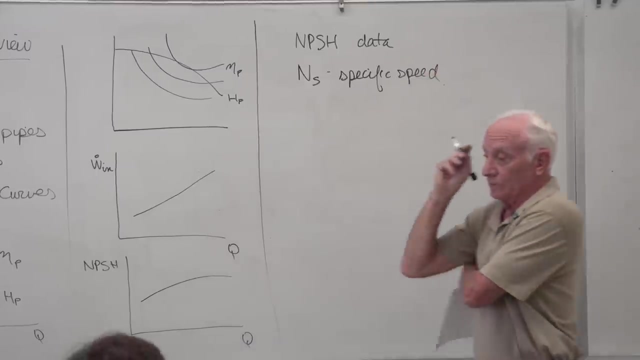 And you saw the practice midterm idea. I did ask that You might be asked to find the pump-specific speed, which tells us what kind of pump should I select for a given job. Should I select a radial pump, a centrifugal pump? 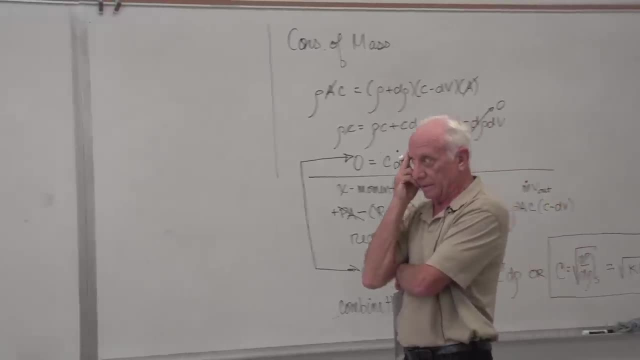 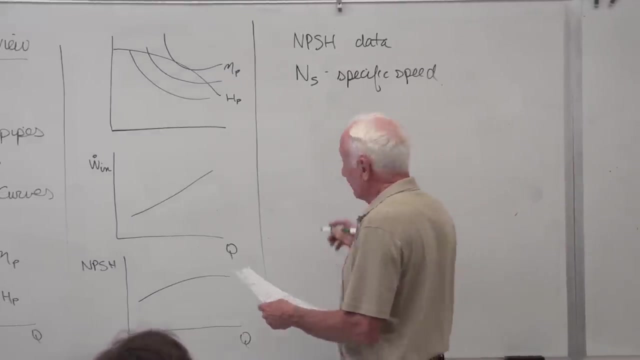 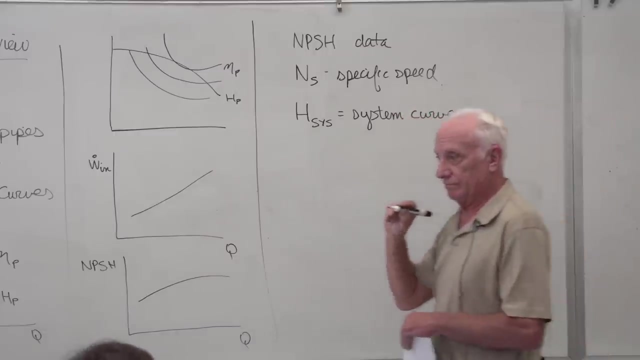 an axial pump or maybe a MEX flow pump. Okay, It depends on the value of that N sub S, which pump you're going to maybe select. And then you want to know the system curve. How do you find it? Well, you write the energy. 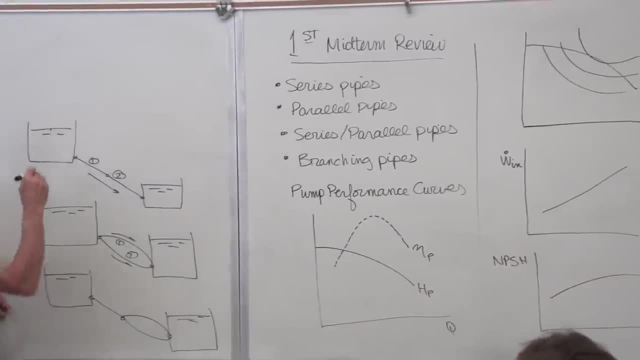 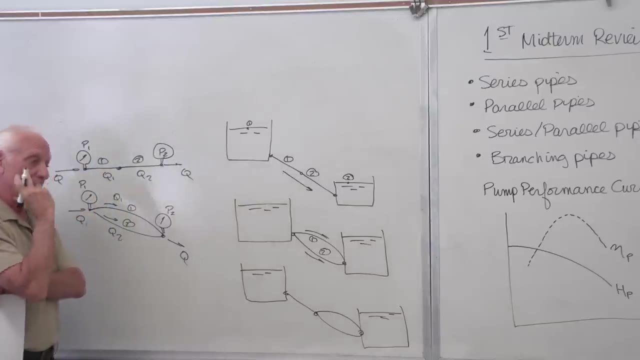 equation from point one to point two. Here's point one, Here's point two. Velocity at point one: zero. Velocity at point two: zero. Pressure at point one: zero. Pressure at point two: zero. What's the difference? 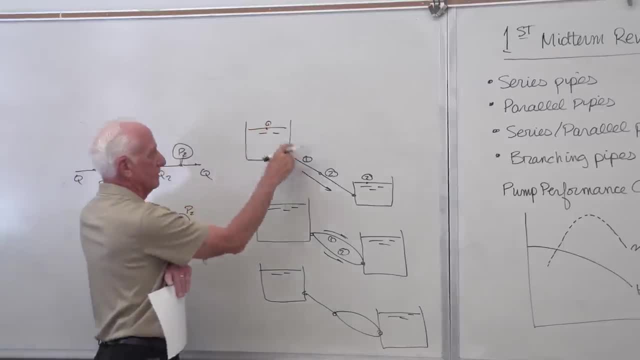 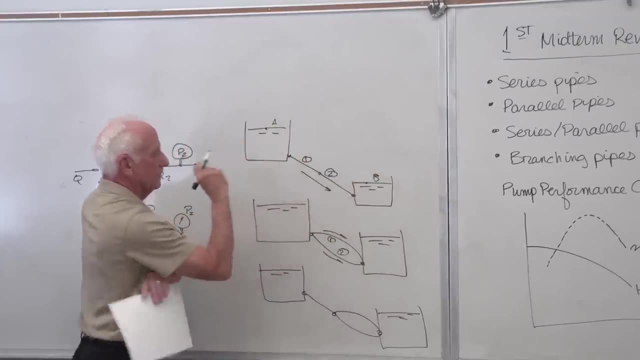 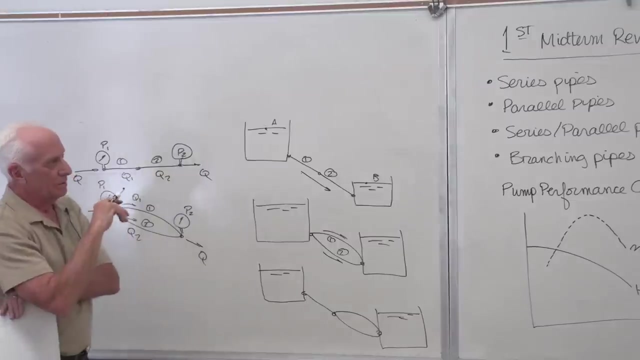 Elevation. I call it A and B, That's one and two. That's A, That's B. What drives the flow? The difference in elevation of the free surface, ZA minus ZB. Okay, That's the system curve. 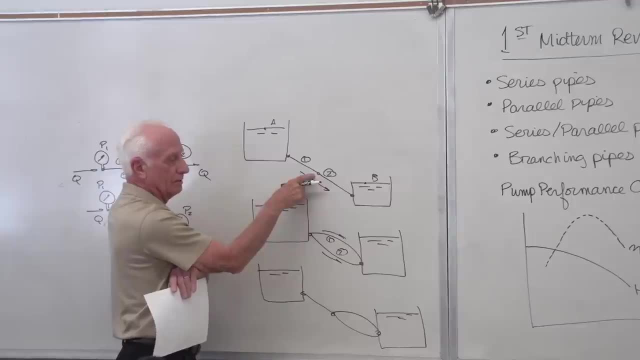 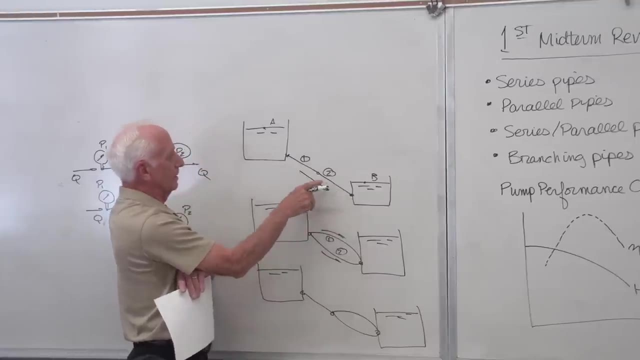 Is there some friction in that pipe? Oh yeah, That's HF1.. Is there friction here? Yeah, That's HF2.. Do the HFs add: Yes, they do. Do the HFs add: No, they don't. 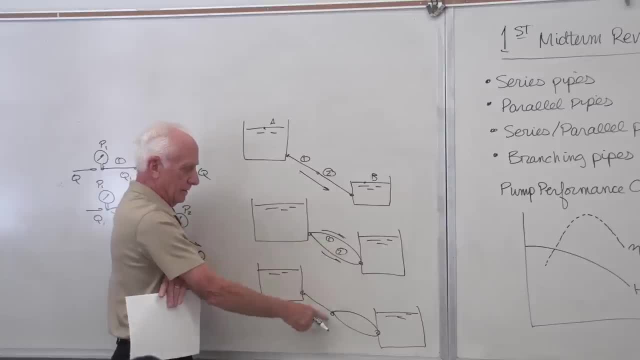 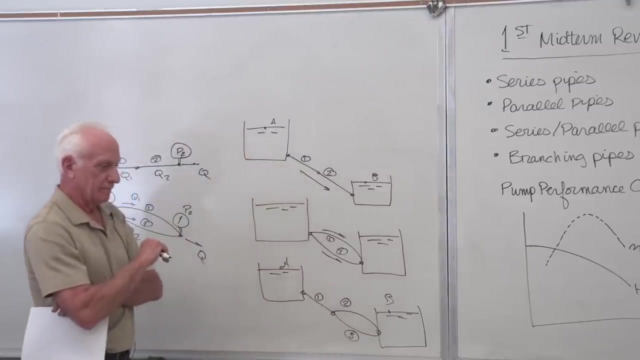 HF1 equal HF2.. What's the friction loss here? from point A to point B? HF1 plus HF2.. Don't use HF3.. Or you could: The friction loss from A to B: HF1 plus HF3.. What isn't it? 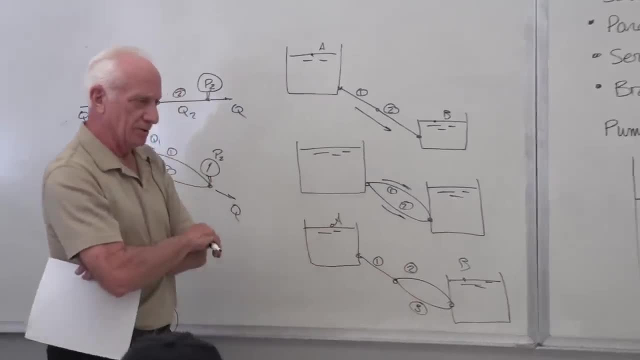 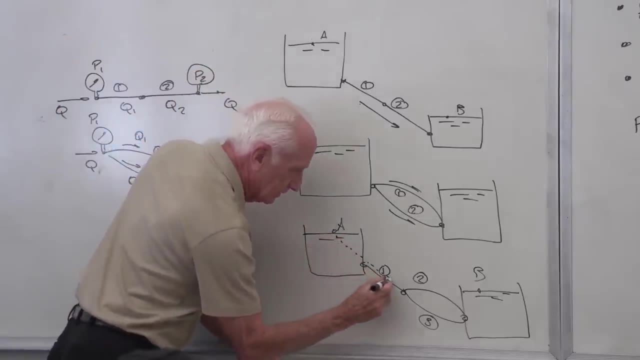 What it isn't is the friction loss from A to B is HF1 plus HF2 plus HF3.. No, you're wrong. Watch my pen. Some water goes that way. What's that going to be HF1 plus HF2.. 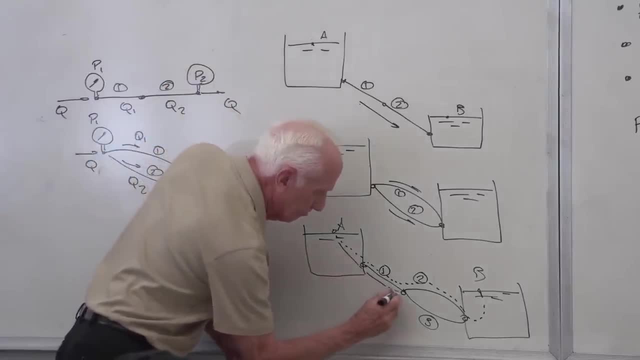 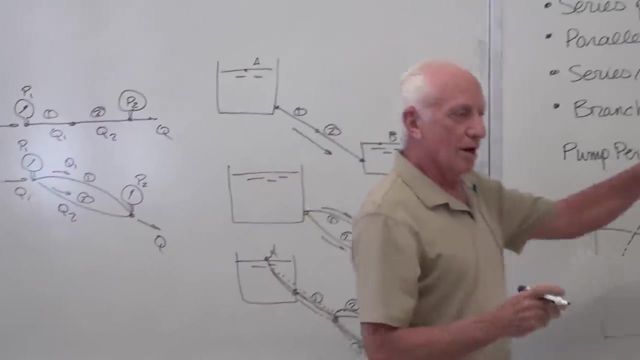 Or some water goes this way. But this is what water doesn't do. It comes down here, goes through here, goes back through here and back out. It doesn't do that. Believe me, It doesn't do that. Know how to draw the system curve.